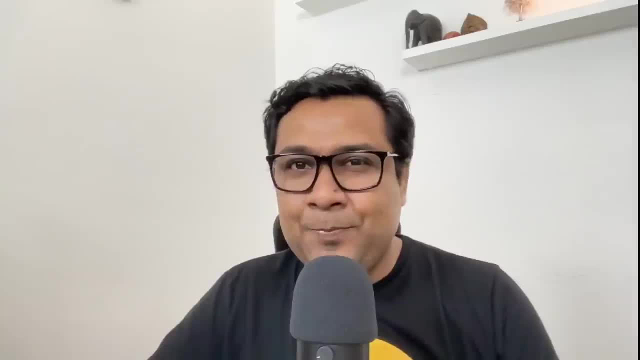 is about JavaScript functions, So we'll be going through a bunch of details about JavaScript functions in and out and try to understand, with lots of code like, how it works fundamentally. One thing I keep saying folks, is that the concept is much, much bigger than the syntaxes. 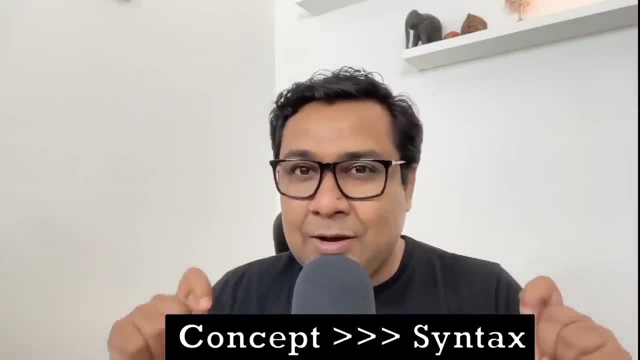 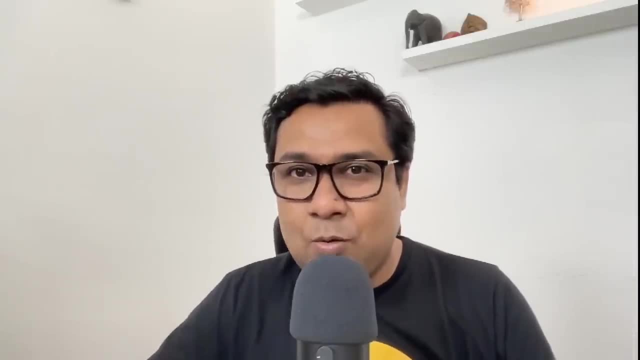 While we'll be writing code, but we want to deep down in the concept first and then complete that with the syntaxes. I hope you enjoy this entire course and, if you so, please like and share this video. If you like this video, please subscribe to my channel and hit the bell icon so you don't 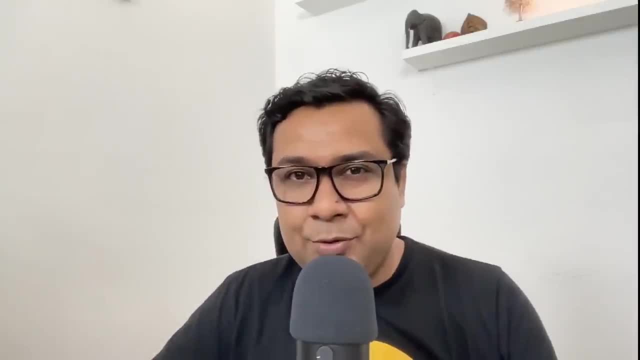 miss any new video. If you have any doubts, comment below. I'm going to respond to you with all the doubts clarifications. Be assured about that. Okay, so a few things before we get started. How to take this course. This is a longer video because of course, it's a. 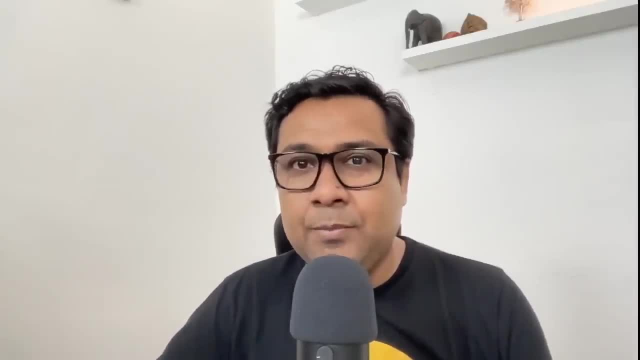 crash course. I have to fit in a lot of stuff within one video, But if you follow certain patterns, you will be enjoying the entire journey of going through each and every topic that we're discussing in this video. Okay, so, first thing, take breaks. Don't try to. 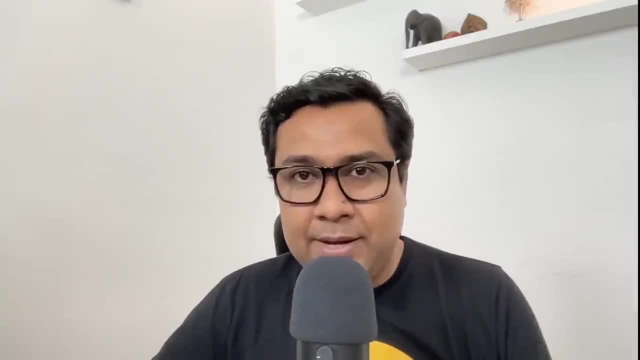 consume a lot of time. If you don't have time, take a break. Don't try to consume a lot of all the content at once. take adequate breaks and then try to feel like what you have learned are just few seconds back. second thing: after every logical chapter within this course, try to 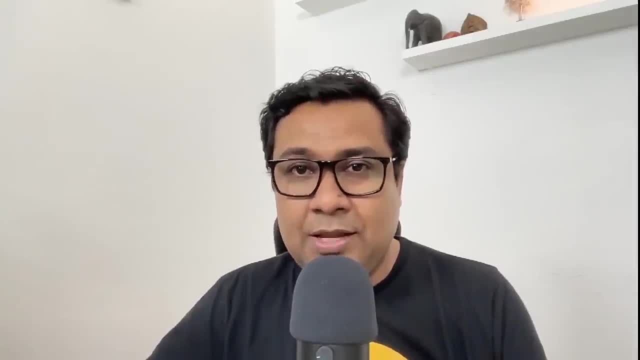 understand whether you have completely got the concept or not. if not, go back and try to relearn. no problem, anytime go and try to relearn. i will be teaching lot of exercises, so you have to do this exercise with me, but don't type them as i am teaching. okay, first try to understand what i 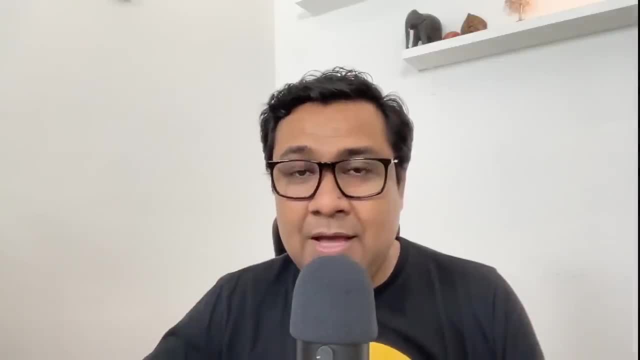 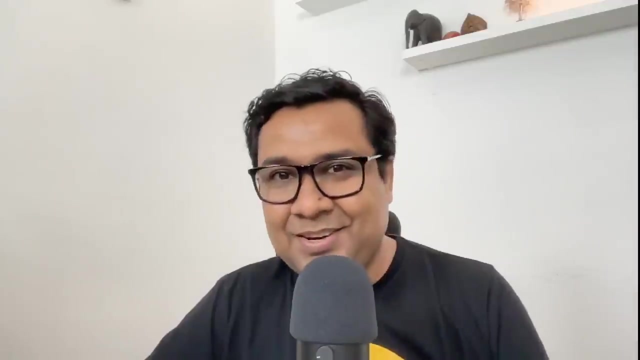 am teaching. try to completely get it in into yourself and after that pause the video. try to do this. you know those, those code part by yourself. all the code examples are already there on github and the link to that is there in the comment section. sorry, the description section of this. 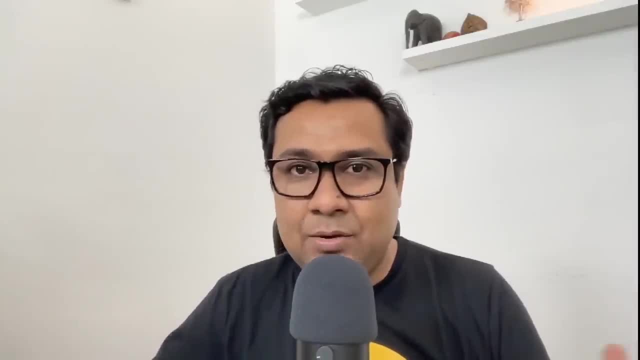 video. you can anytime pull it up and try to see, like you know, what is the code look like. so no worries about that, but try to understand what this is teaching. you do not know what i am teaching. okay, first try to understand what i am teaching, try to completely get it in into yourself and after 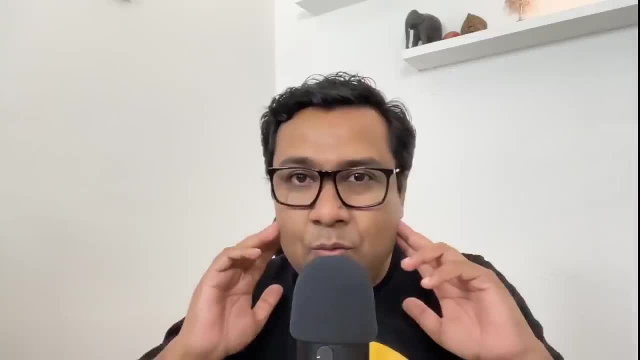 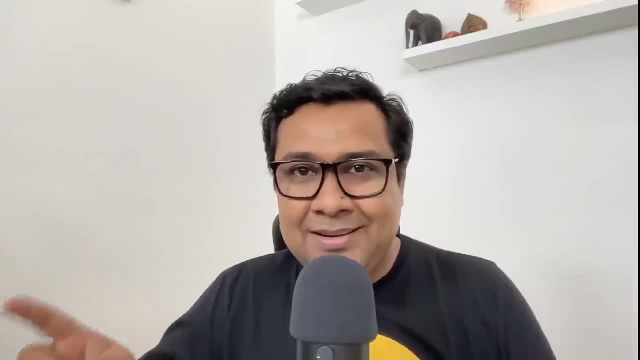 but don't type the code as i am teaching, because then you won't be focusing on what i am teaching, rather focus on learning and then try the code out. so go repeat, come back, learn and everything, and in case there is nothing clear, feel free to comment. i am going to respond to you. so 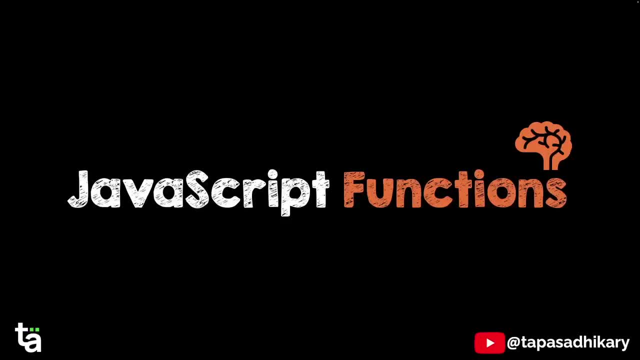 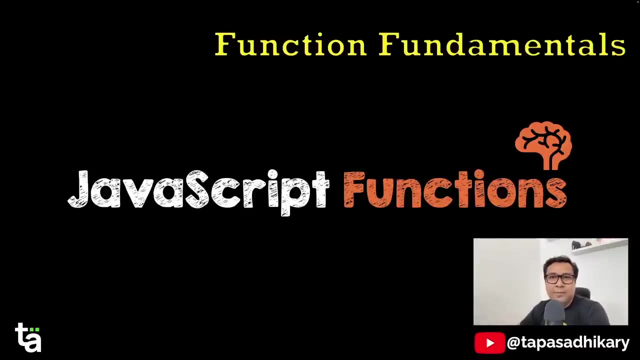 without any further delay, let us get started. let's quickly talk about the concepts we'll be covering in this crash course. so, first thing, we'll be talking about javascript: functions, fundamentals. what is function? what is it used about? a very, very basic level, right, i'm considering a beginner. when they watch this crash course, they will be able to. 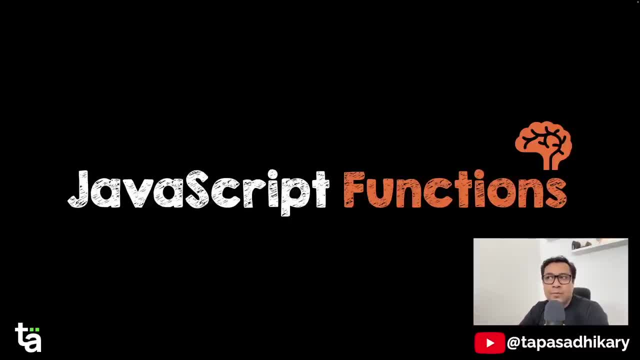 understand what functions are and why they are used, then we'll be clarifying few terminologies. there are few terminologies which are a bit confusing when you learn functions, for example, functions versus methods, parameters versus arguments, and there are many more such terminologies that we want to clarify. next, we want to talk about 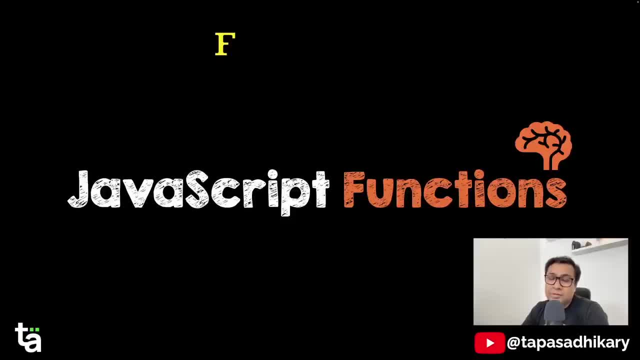 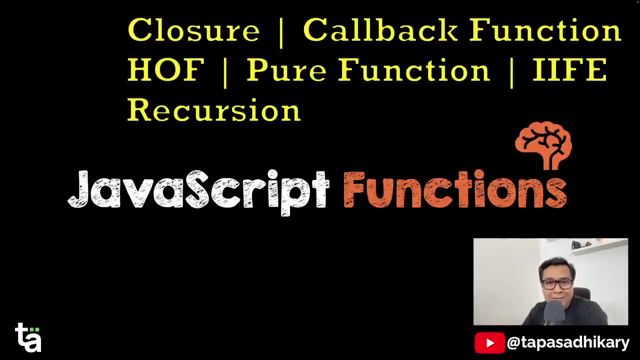 function declarations. we'll be talking about function executions. then we'll get into call stack, we'll talk about arrow function, nested function, function, scope. we'll talk about closure, we'll talk about callback functions, higher order functions, pure functions. we'll talk about iife, we'll talk about recursion. so there are lots, lots, lots to learn. there are lots to talk about. 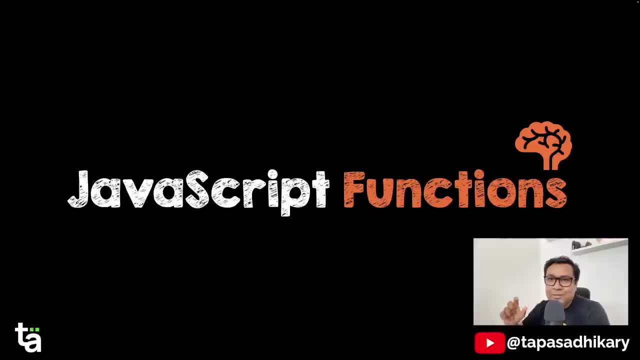 that's why i told you, like, when we go to each of this chapter in this course, understand one chapter before you go to the next one and please practice the chapter before you go to the next one. all right, so take your time and let's get started with the learning. the first one: 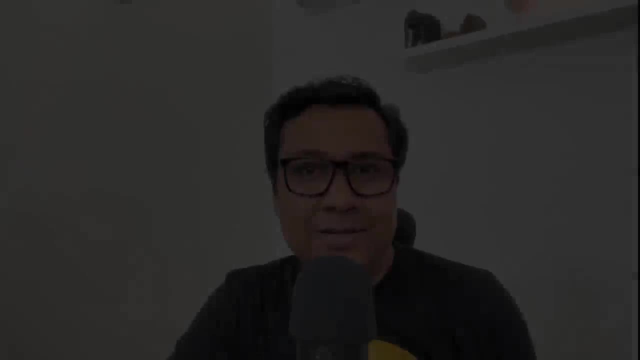 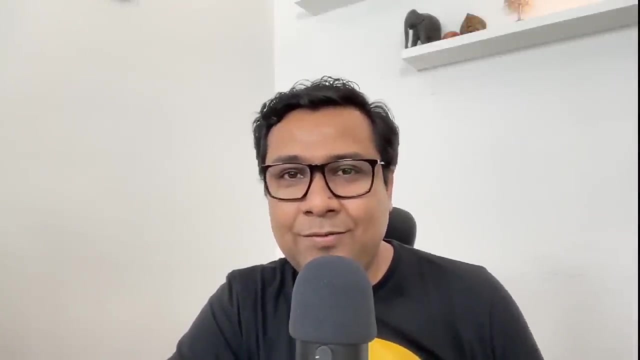 about javascript functions and its fundamentals. so what is javascript function? before i get there, let me tell you a story. it's the story of two friends, one of the friend actually trying to cook a dish, but she doesn't know the recipe of how to cook it. so she called her friend who is sitting abroad. 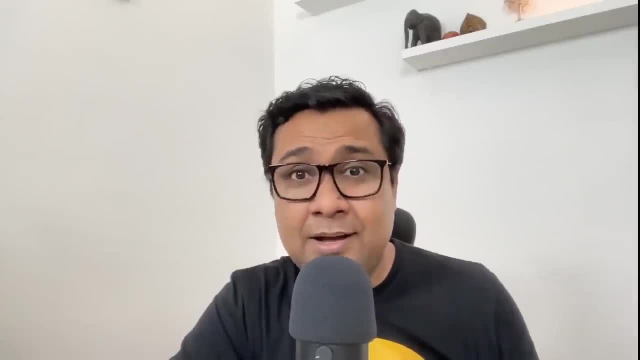 over phone try to ask for the recipe. the friend at the other end. she received the call and told the recipe line by line, saying that hey, if you want to cook this dish, you have to follow this recipe like, you have to put this first, then you have to put this one, then you have to cook it for. 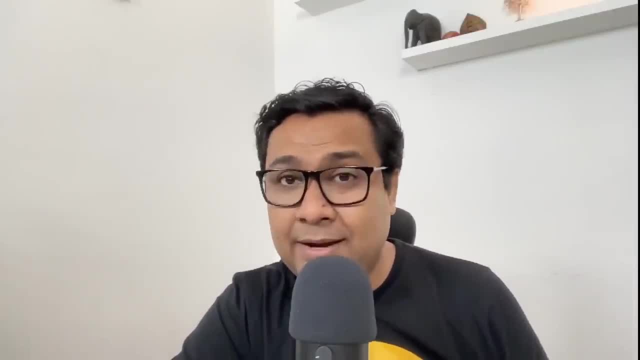 so long and then, finally, your dish is ready. great. the friend cooked the dish following the recipe that she got, but after a week, when she tried to cook it again, she felt like: okay, let me ring up my recipe. and the same thing happened. the friend gave the recipe over phone. she followed the. 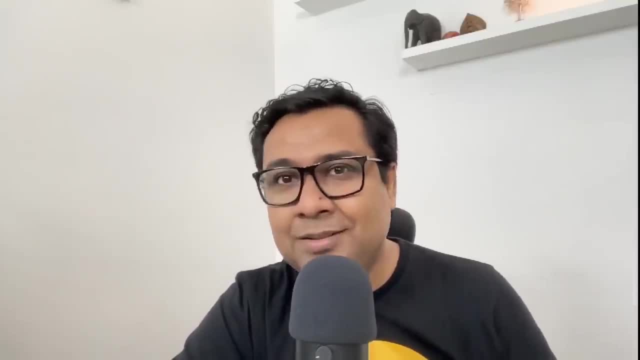 instruction, cooked the favorite dish. next month. the story remains same. she calls up the friend again, again got the recipe, cook the dish. for few months. it went on like that. but after that, even though their very best friend, the friend who is sitting abroad- really got frustrated of it. 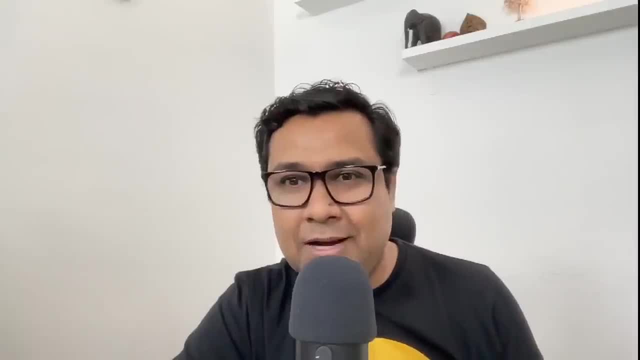 and just told: hey, i have been telling you this recipe for like four or five months now. why don't you write it down somewhere, so that you don't have to ask me again and again and i don't have to perform this task of telling you again and again? rather, wherever you're writing it, you 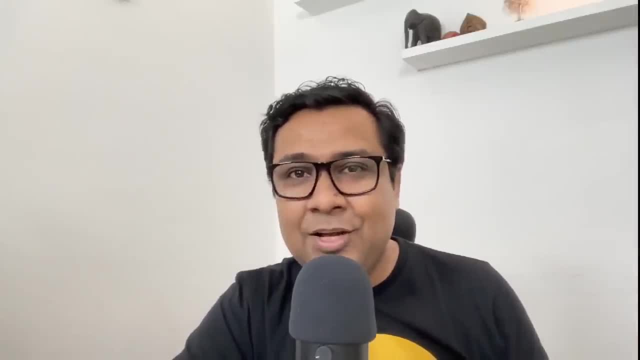 probably can fetch it from there. then what the friend did? she wrote the every instruction in her diary, and next time onwards she never rang up the friend abroad, rather followed it from the diary. javascript functions a little bit like that, so it saves you from repeating the same task again. 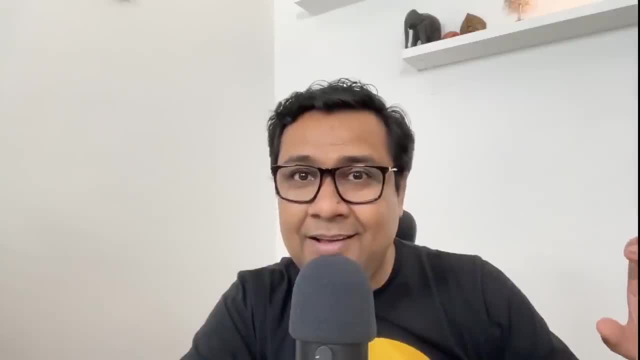 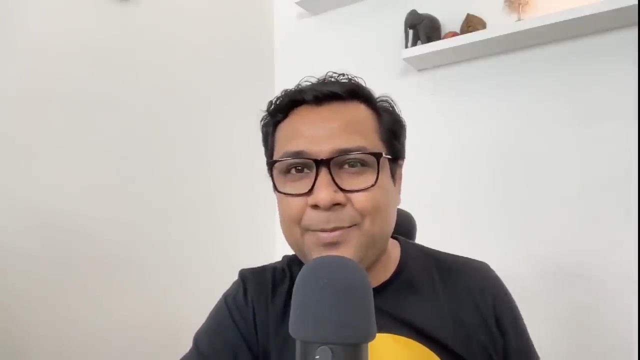 and again. rather, you put the task somewhere and then reuse that every time you have to perform the same. similarly to that friend's story who wanted to cook the dish but finally, actually, instead of giving the task of her friend to tell it again and again repeatedly, she fetched it from 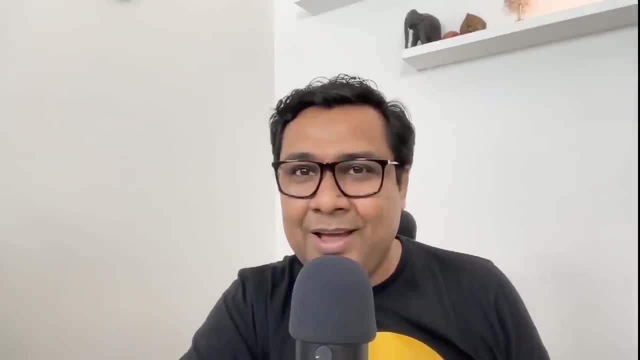 the diary, the friend never had to perform the task again. okay, so, with this analogy in mind, like reducing the task, performing the task again and again, rather, we will create something so that we can actually reuse it whenever required in our programming. that's the very, very fundamental aspect of functions. now we will be getting into a graphics. 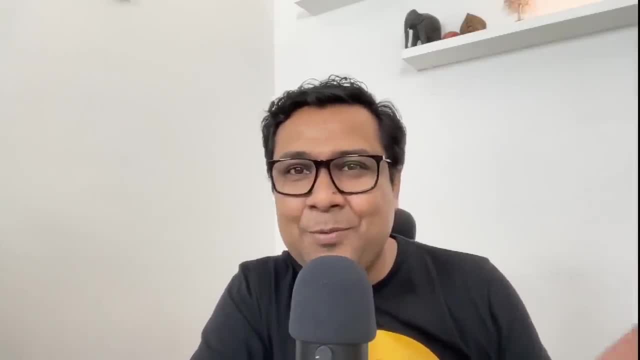 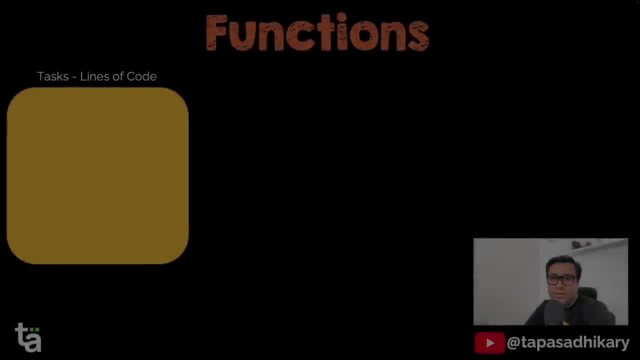 through which the similar kind of story we'll be putting into the code in a visual way and try to understand what exactly function does programming the yellow box you see on the screen. consider that is a program and in that you have bunch of lines of code. now 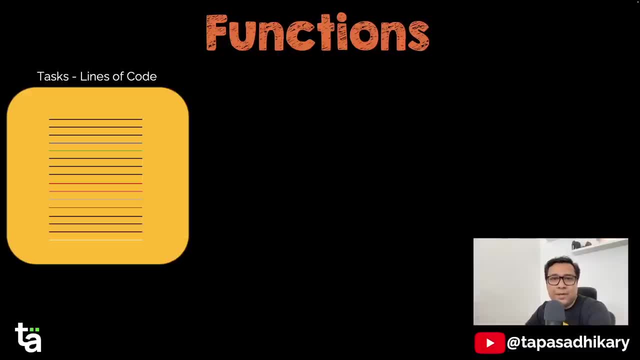 just look at it a little bit closely. there is a color coding. there are a bunch of black lines, then there is a green line, again bunch of black lines, and is a red, orange blue, again bunch of black lines, and then there is a white line, right? so what are you trying to mean here, those black? 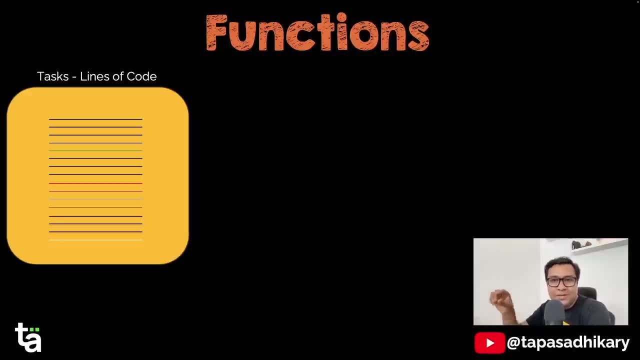 lines are the kind of code. the same code has been repeated multiple times. so 3 black lines, then some other code, then again same 3 black lines have been repeated, and some other code, then again 3 black lines got repeated, like that. right, there is a repetition exist. now we want to bring in the concept of java javascript functions here. 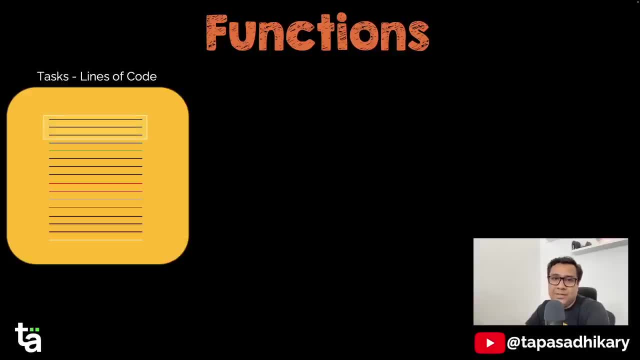 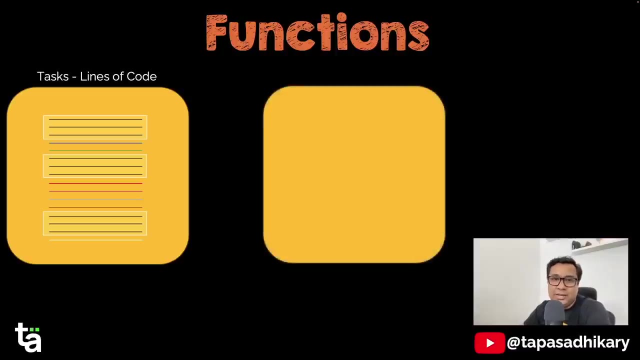 so that we can reduce this repetition. so what we do basically in this case, you know, going forward- is we first mark what are those lines, that is, that are getting repeated. so you see, here we have marked those lines that are getting repeated, and the next thing that we do is like: how can we? 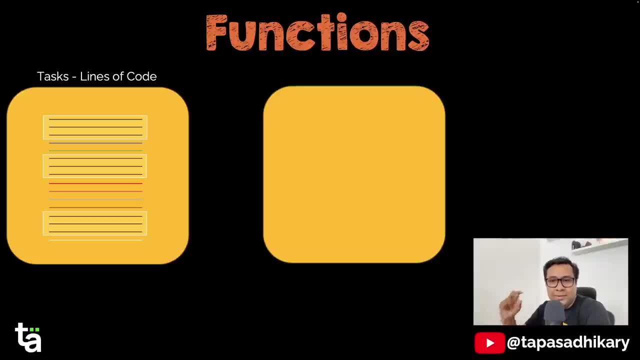 make this code better so that we don't repeat the same task, right the same lines, rather than that we kind of take those lines somewhere, give it a name- in this case, the name is like fun- and then what we do is like the same code that we got, change it in such a way that, instead of 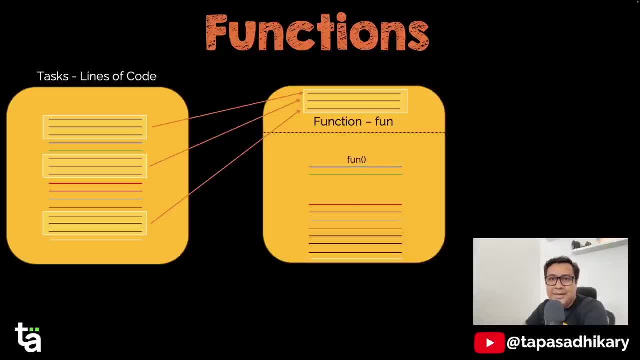 those line. we are going to use the same entity- the fun- we had created before. so do you see? this one, the number of lines of code has reduced drastically. you so what we did. instead of repeating the same task in your code- the first one- we have now put the 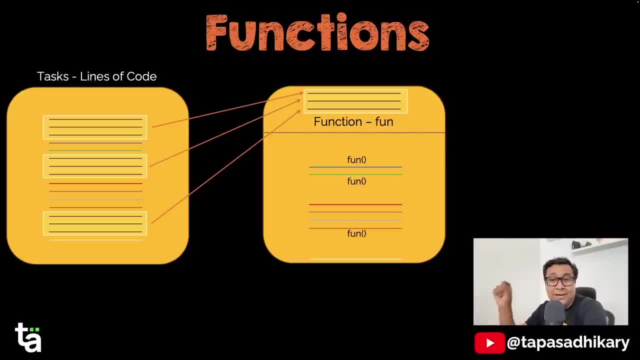 code in something which we call as function, given it a name called fun, and then use that fun in our code instead of repeating those lines every time. so we are not only reducing the number of lines of code in, you know, in our total source code, but what we are also doing is, basically, we are 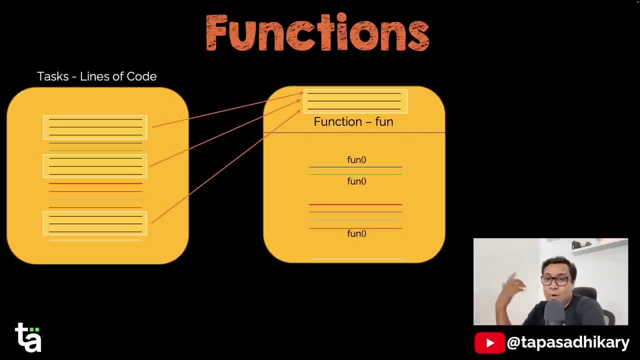 reusing something again and again. now think about this and we are going to do the same thing in the same way we have done in the previous case. so let's say we have a case like why, why do we need it? the best case probably is: let's say there is a problem in these three lines, there is a bug in these three lines. so in the previous case if there is a bug and you have to fix that bug or you have to fix that issue, you have to fix this issue at least three times. so you have to fix it in the first bunch of line, then again the second bunch of lines, then again in the third bunch of line. but as we have put this thing into a function in a single place and then reusing the same with its name in the multiple different places, if you have put this thing into a function in a single place and then reusing the same with its name in the multiple different places, if you have put this thing into a function in a single place and then reusing the same with its name in the multiple different places, if you have put this thing into a function in a single place and then reusing the same with its name in the multiple different places, if 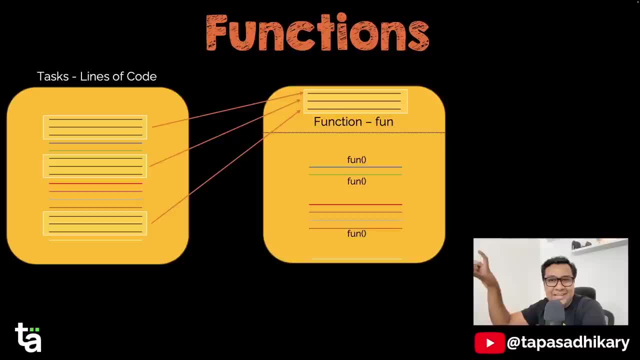 you have to fix the bug now. you have to fix it in one place, just inside that function's body, just inside that function, and then rest of it will work. so functions are a bunch of blocks that you keep together to perform something which otherwise will be very, very repeated in your code. functions should ideally have a name, but it can be without a name. also, in most of the cases you will have function with a name so that you can call. 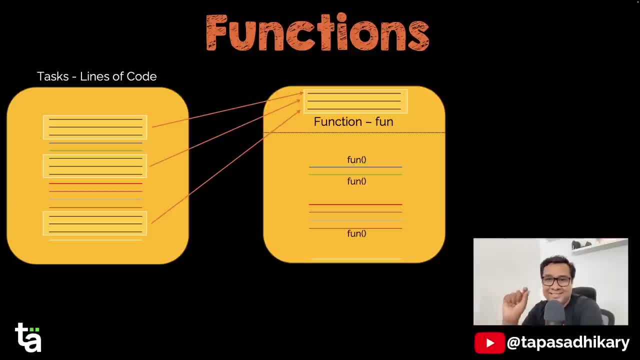 the function with that name. so you me, every human being, has a name and the purpose of the name is like we will be called by that name and when someone will call us by that name will respond and say: hey, i am here, i am, i am the person. similarly, for the function. when we call the function by the name, function will say like: hey, i am here and inside this i have this bunch of code. go ahead and execute this code. okay, so that's the beauty of javascript function. i hope you understood it. 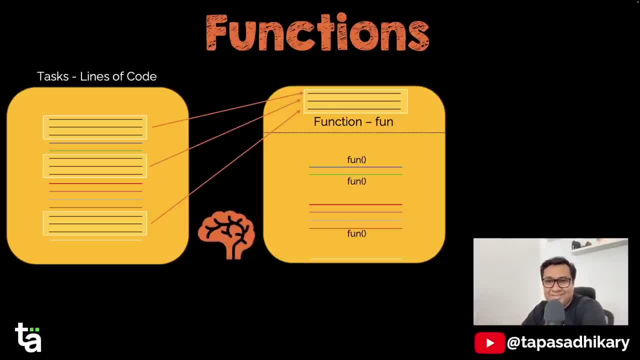 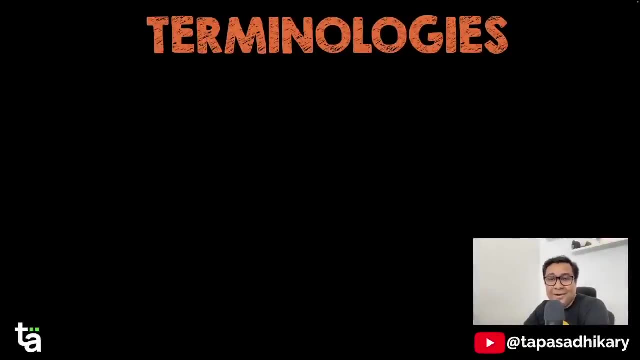 you know these graphics and please keep it in your brain, because you know the rest of the crash course. we are going to use this terminology again and again, you know, for better understanding. in programming, at times terminologies are much more harder than the programming itself, and when a developer gets stuck on those terminologies they feel so discouraged of learning that particular programming language. it happens so. that's where, when we are learning any programming language or an aspect of a programming language, 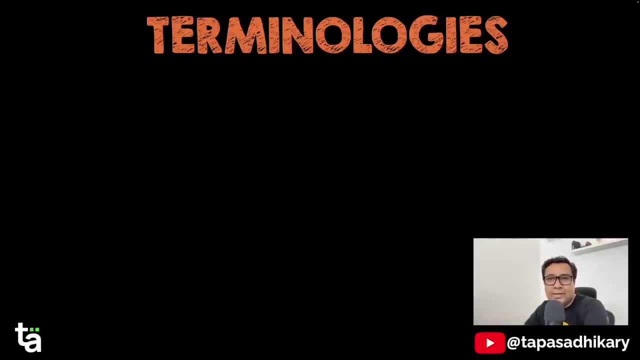 you have to make sure that we understand certain terminologies very well when you are learning javascript functions. there are few terminologies that you also need to know and you have to differentiate between them very well. so some of the terminologies are functions and methods. what are the differences? we're going to talk about that then. declaration and definitions: what is? 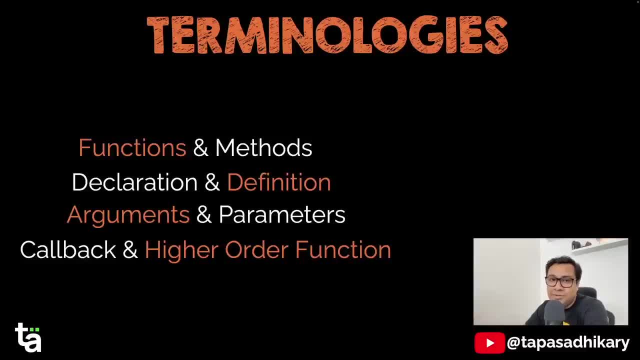 the difference? is there a difference between them? arguments and parameters- we'll be talking about that as well, and then callback and higher order functions. you will get confused often with these two. we'll be talking that also deep down when you go in the course itself. so these terminologies keep in your mind, like when we are talking about it. make 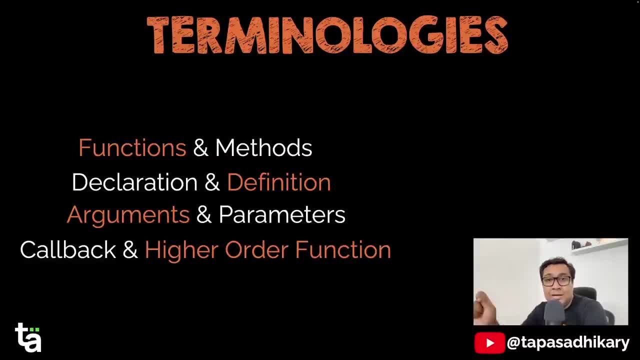 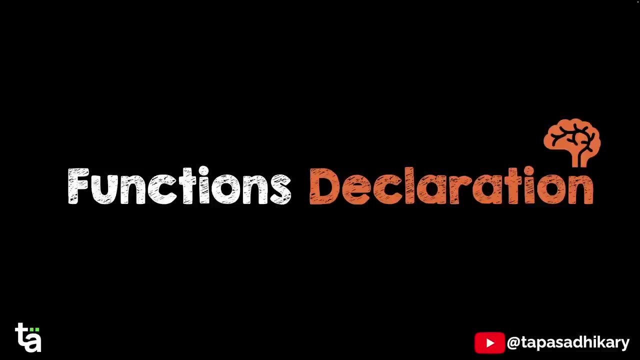 sure that in your head these terminologies and their differences or their similarities is completely chalked out, completely cleared. if not, go back and try to see like where i have explained this one. if you still have further questions, ask them in your comment section. i'll get back to you. 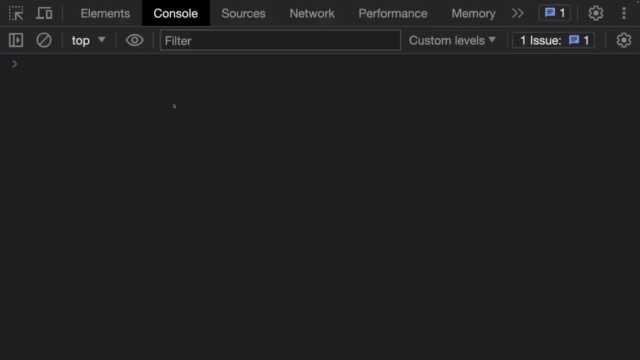 let us now start creating functions and try to learn like: how do we create functions? okay, as a thing before that, so you can use any editor, like you can use visual studio code or any other editor of your choice. while coding what i am using right now, i am using browser's dev tools and the console tab. 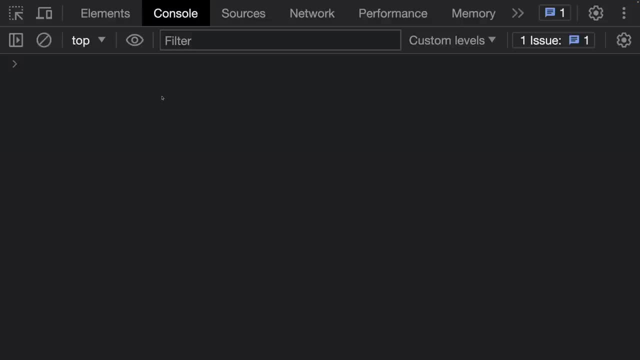 so that i can write the program here and execute them there and there. so if you want any other mechanism, like you will be writing on visual studio code and use the live server to run your program, most welcome. or you can actually practice them on the browser's dev tool: just go press f12. 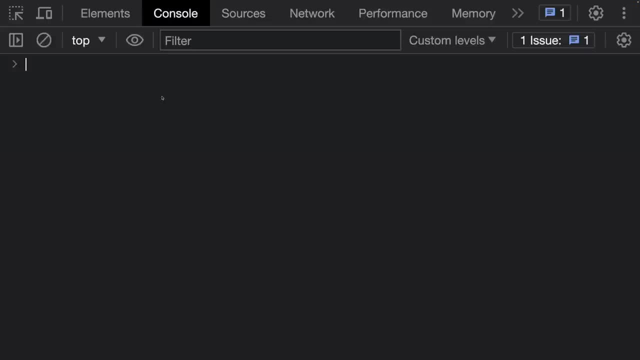 open the dev tools, go to console tab and start writing your program and execute it, because you are just practicing at this point of time. so first, first thing. first, what we'll be doing now is we'll be creating function. so we told that function is something which is going to help you. 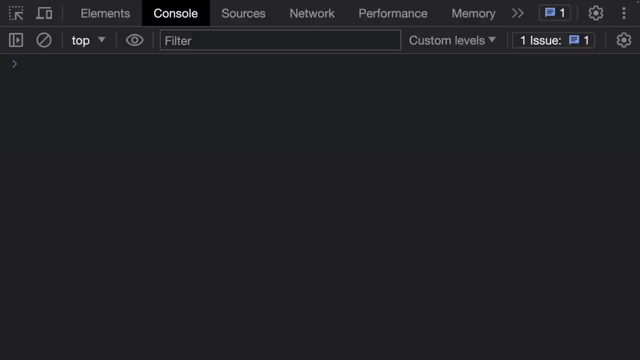 to keep a bunch of instruction and code in a place so that you can reuse it again and again when you need it now to declare or to define a function. so our first terminology bang declaration versus definition. so these two things are exactly same. when it comes to function, function declaration, function definitions- defining a function is kind of same. 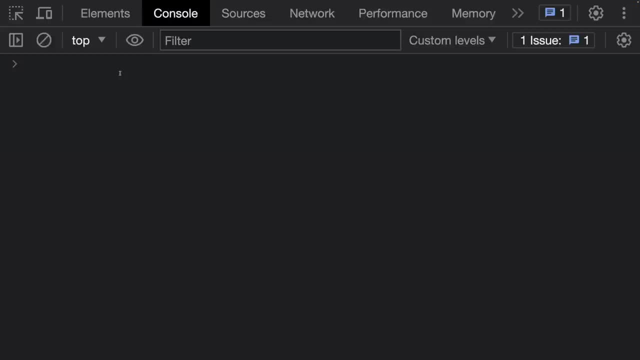 so if somebody is saying i'm declaring a function or another person is saying i'm defining a function, they are actually talking about the same thing, which is nothing but creating a function with bunch of logic. so what we're going to do now we're first going to create a function, so to do that i have to use a 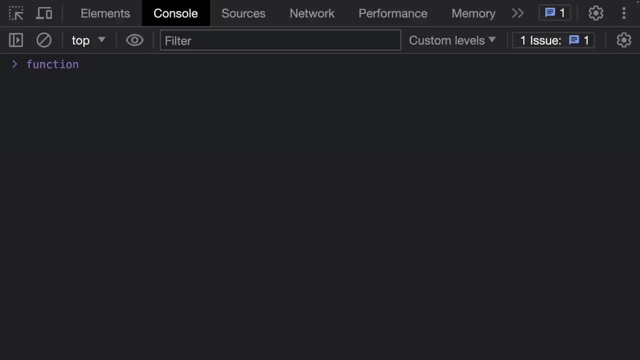 keyword called function. this is the keyword and then i have to give the function a name. i told just now the function may or may not have a name, but most of the time the function will have a name so that we can call the function by its name, just like the human being has name. there are situations. 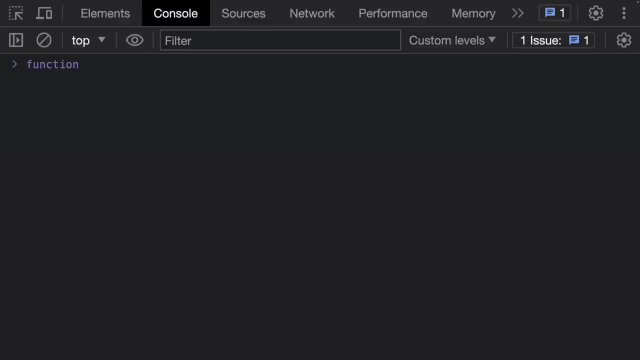 where the function may not have a name, and we'll talk about the situations in the in some time in this course. okay, so let's first give a name. let's give a name called print me and then give a- you know curly braces and then close that curly braces. so this is what you have declared, or you have defined a. 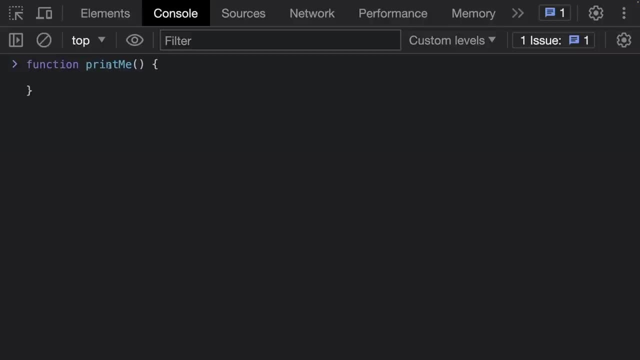 function okay. so right now the function has a keyword, a name, a bunch of parentheses and then a curly braces- open a curly braces, end. inside this curly braces, you are going to write every logic that you want this function to have, so that you can reuse this logic anywhere you want. so for 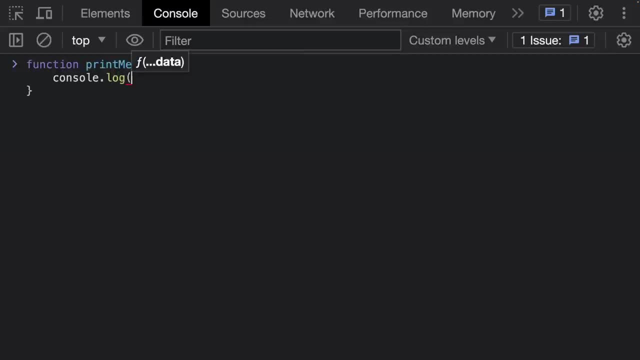 example, this particular function may just log certain thing into this console. so you do console dot log, console dot log. console is like an you know something that you already have with javascript on this particular debugger, so that you can use it for your coding purpose, for your debugging purpose. 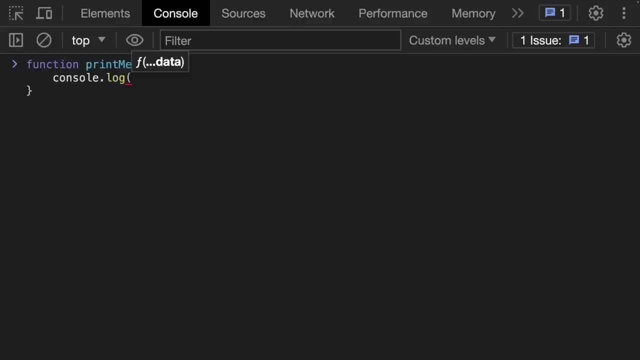 and on console. you have varieties of methods. one of the method is log, through which you can log something in the console so that you know you can actually read them, or it's more for the debugging purpose that you can use. okay, so let us do something like printing something like this: 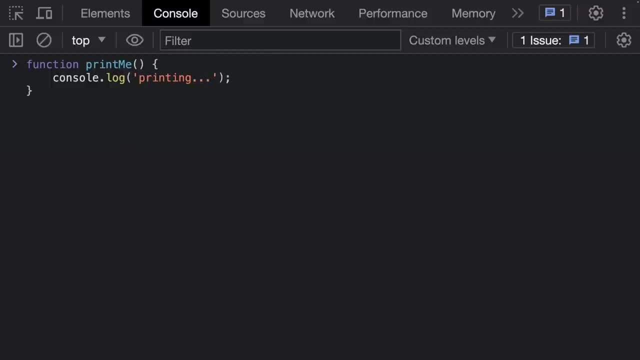 okay, so i have created a function with a function keyword and the name called print me, and the instruction the function has is is a log that i want to print in the console, and that log says printing. that's it. so that's my function definition, or function declaration. now, as i have declared this function, 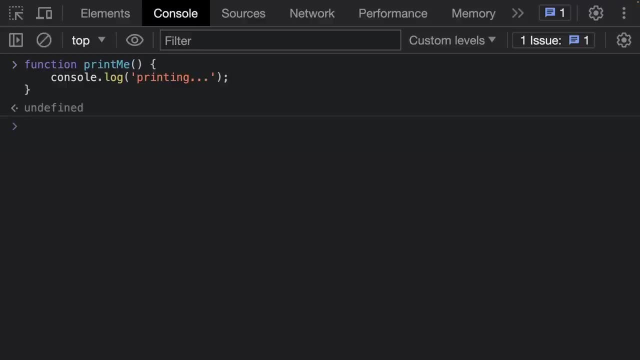 with the name. the next thing that i can do beautifully is by calling this function. so to call this function, just type the name of the function you know, print me over here. there is autocomplete already, and then to call it you have to give this parenthesis, otherwise you are just. 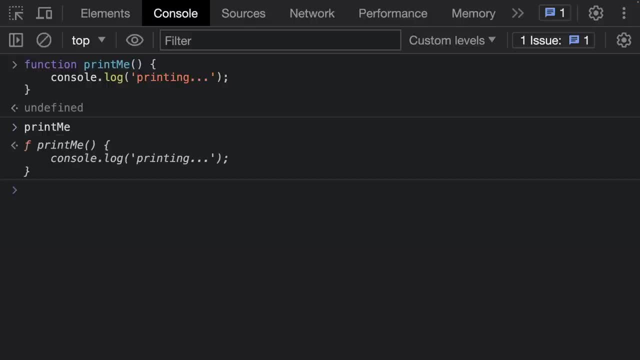 printing this particular function's name, and if you just do this, the function is going to print its complete body itself. so if you just do this, you are going to print this function's name, and if you just do print me the name itself, it is going to give you a string version of the entire. 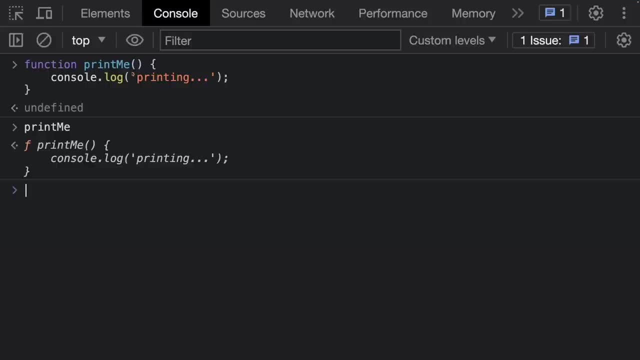 function's definition or declaration that you have done just now. but to execute, to call it specifically, you have to give this parenthesis. you must give this parenthesis and then you press enter, it will give its output. it's just log printing, because that's exactly what we ask. 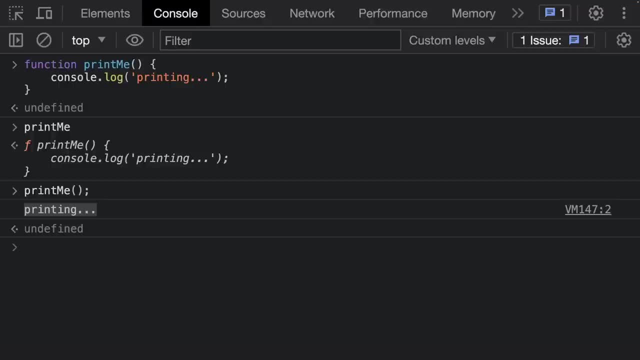 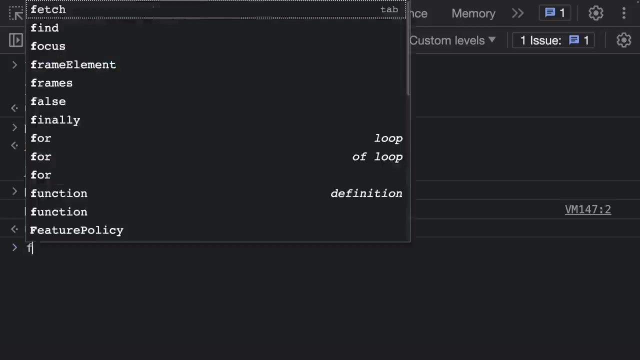 this particular function to do so. our function has worked. that's great. now, as the function has worked, um, i want to just do something more with this. okay, so this is where what i'm going to introduce, something called parameter. okay, so let's write the same function, function and we: 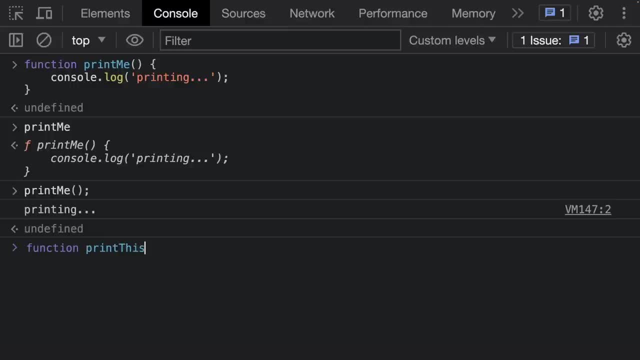 will say the name is: print this and we will pass something over here which we call as parameter. i'll get into it in a minute and then i'll close this function's body and inside this what i'm going to do. i am going to write like this: 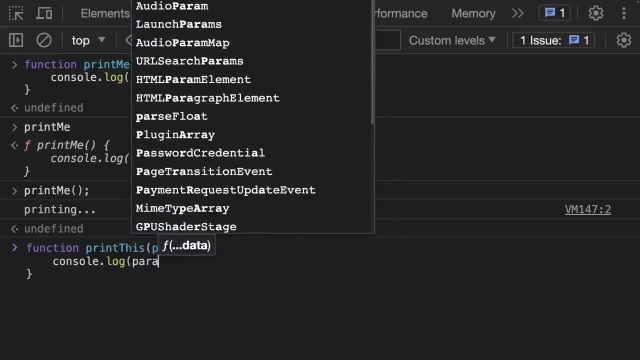 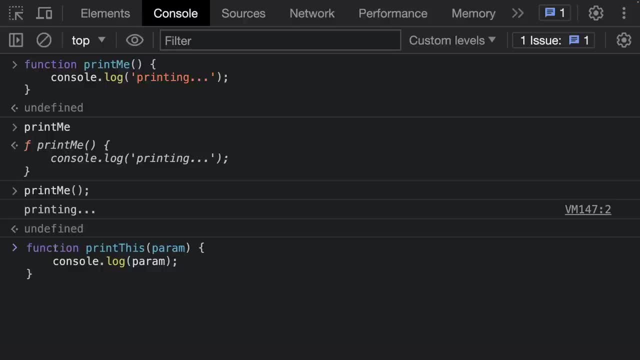 console dot log param. so what is it what? what does it mean? what? what i have done here? okay, so i have first similarly created a function with the function keyword and the function name. here i have not done anything between these two parentheses, but in this case i have done something in the 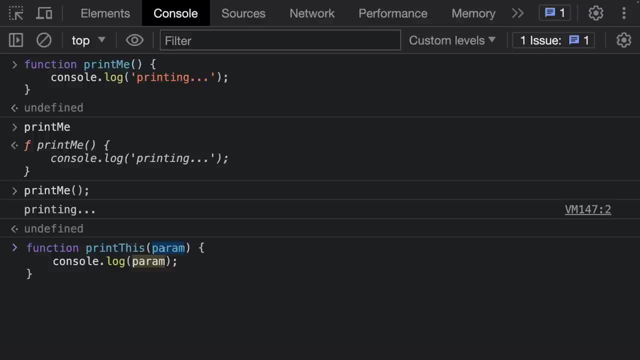 parentheses. so whatever you put inside this parentheses of a function, it's called parameters. okay, whatever you put inside this parentheses is called parameters. you can put as many parameters that you wish to, as long as you need in your programming logic. so if i am passing, param is going to just you know i can. 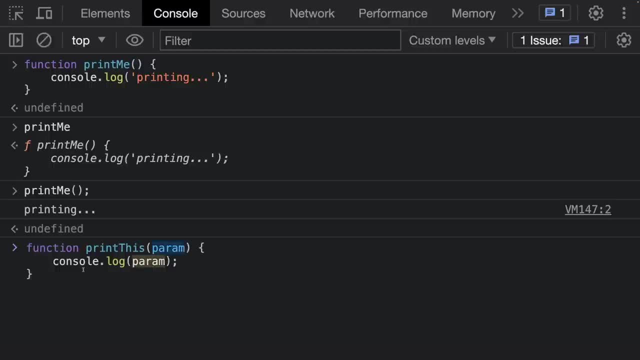 use this param anywhere inside this function so that i can do something with it. so, for example, i can just now do print this and pass this, so it's going to print the thing that i'm going to do and i'm going to do something with it. 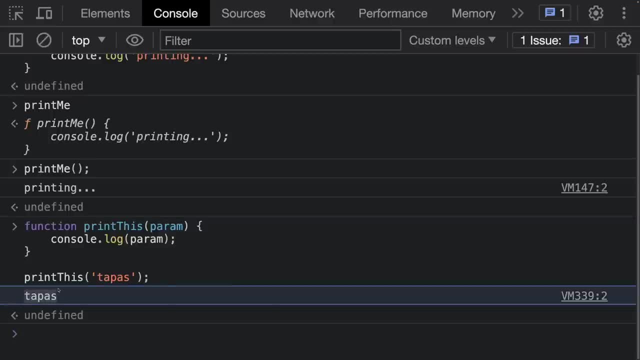 that i have just given over here. so it means i can pass a value to a function and that value actually get mapped to the parameter, and that's something that i can use, you know, inside the function to do anything that we want. so again, there is a thing that i want to call out over here. 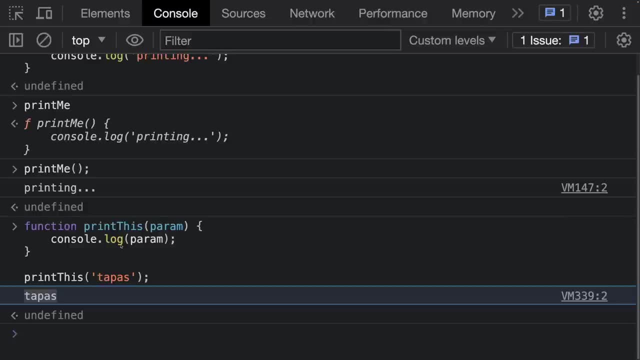 there is a terminology thing: a parameter versus argument. anything in the function definition you pass inside this parenthesis is a parameter. but when you call this function, invoke this function, the actual value that you're passing to this function is called argument. okay, so that's the difference. sometime, what happened that we call? 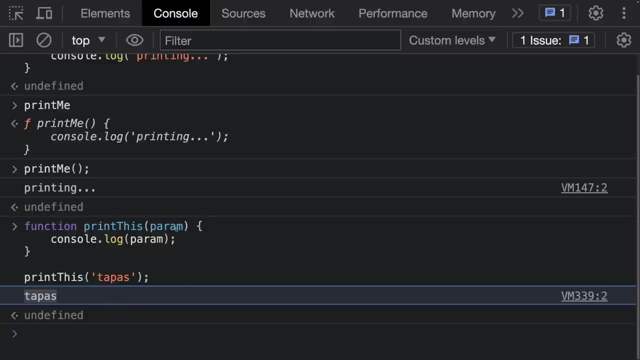 this also as parameter, that i am passing the parameter. we call this as an argument that i'm passing the argument. that's not the case. so parameter is something that you pass to a function while declaring or defining the function, which is like this: but when you call or invoke this function, 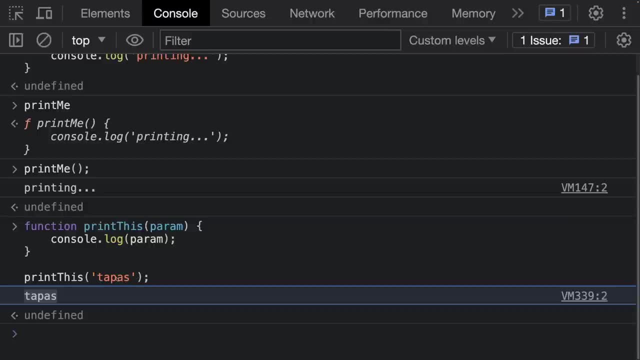 the actual value you pass to it. it's called the arguments. so i hope this is clear to you. the parameter versus argument. okay, great, so we have defined the function and we have now know what is parameter. we have now know what exactly is, you know argument and and things like that. okay, so the next thing: we have defined the. 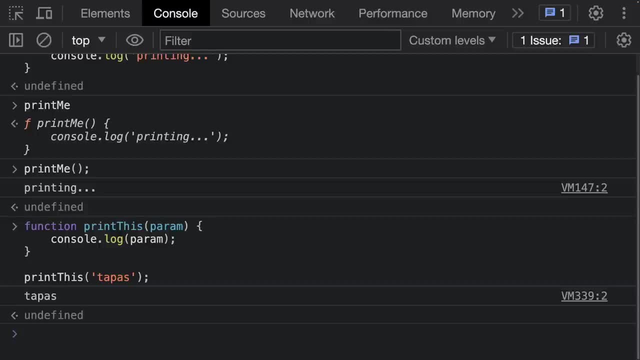 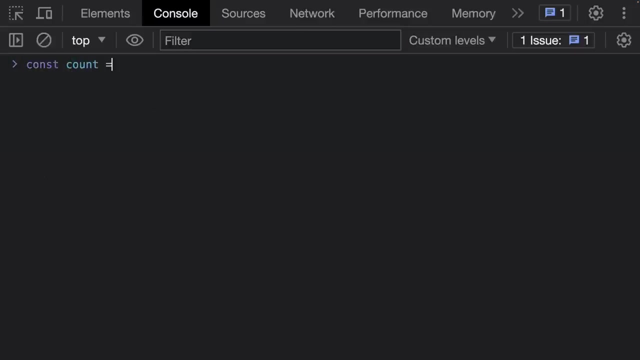 function. but there is one more way we can actually declare or define the function. that's called using the function expressions. okay, so what is expression? let's learn. but before that, let me just clear off all this thing that i have done because i don't need it. so if i say const, count equals to 100, this is an. 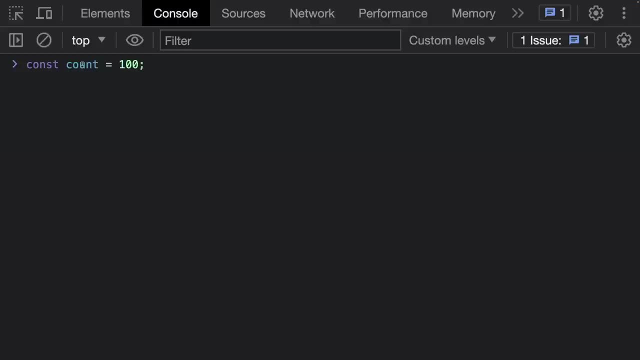 expression what this expression has. it has a variable name called count. it has, like you know, how we have defined this variable. we are saying this variable is a constant and then is a value of this particular variable. okay, so const count equals to 100 is an expression exactly similarly. 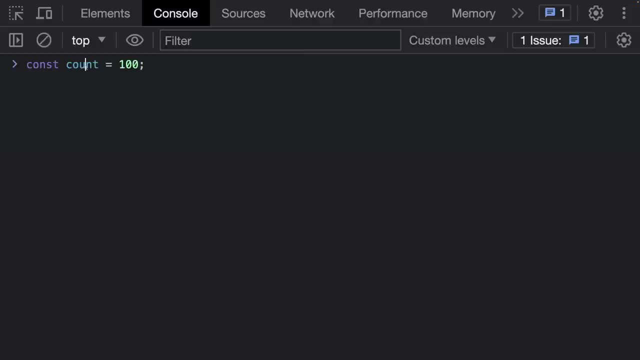 we can actually define a function. so let's take the print me function itself. so print the print me function. the print me is nothing but the function name which we can actually put as a variable over here. and then what we can do here: instead of that 100 value we can give function itself is a value, and then we give the function's body and inside 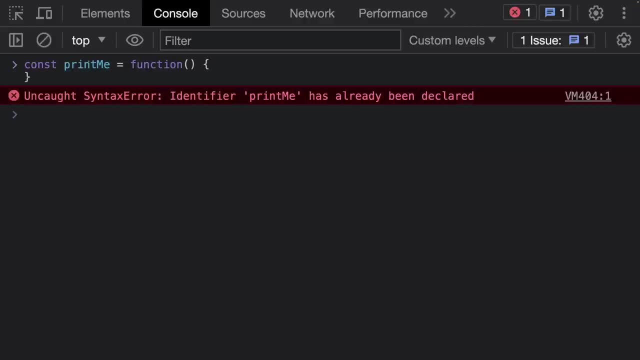 this function body we can give whatever we need. sorry, it's got executed. my bad, i'll just put it over here. um, you can give console Edward joker's llc function and object label. function name is with the first touch of the command l, and then we are going to give ourized this function name as well. so 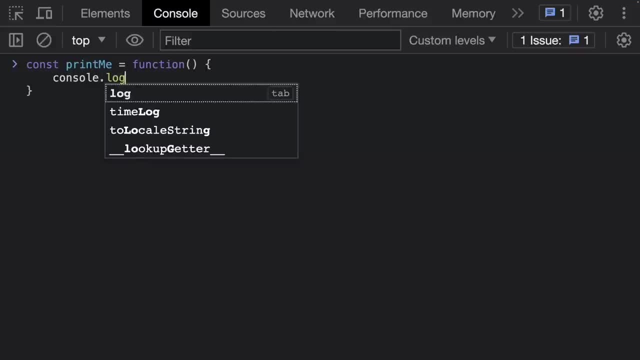 let's see how we will do this. we are going to just take it class memory and dot"amd console, dot log, say print, right, so this is what I have done. so I have const print, me equals to function, and then this, this thing. so previously what I have done. 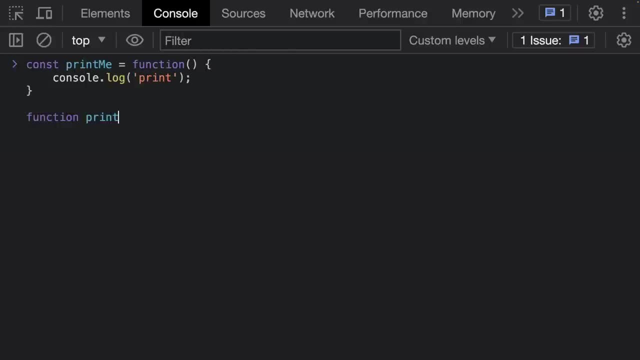 previously I have done this function print me okay. and then I have done here console dot log say printing. so now I have just defined the function, but I have defined the function in the function expression way. so it means that the name that I have used for function 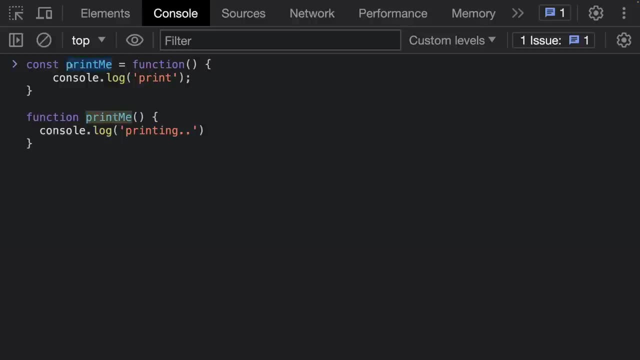 before. now it's a variable, basically, and then the variable: what I have assigned is nothing but a function. I have assigned that a function, so it means print me is nothing but a function. now, when, if I did const, print me equals to hundred, print P is nothing but a number, which value is hundred. now I have done. 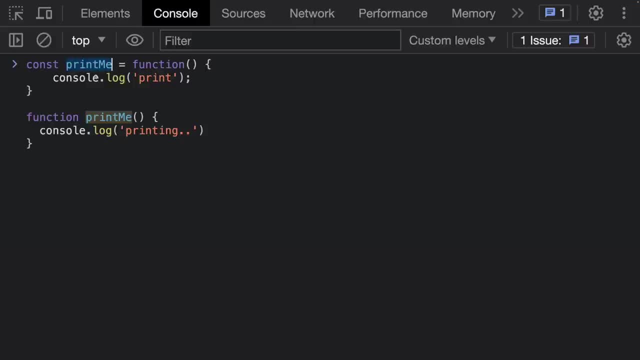 const print me equals to function. that means print me is a function, and then I should be able to execute this function. so first I'll define this: okay, print me, as already declared. because I have used this, let's use some other name for now. say: print me again, okay. so this is the name, and then 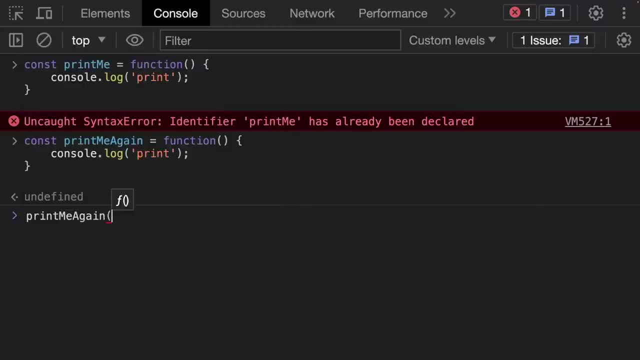 I do print me again and I have to execute me. so I have to do this parenthesis and I got the print. so this is another way I can actually define and declare a function right now. in the same thing, in the print me again, let's say print me again and let's say: 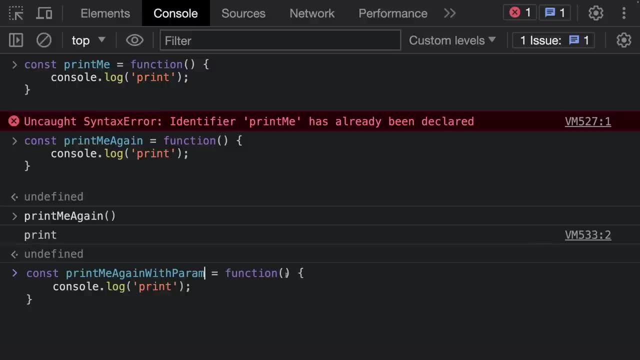 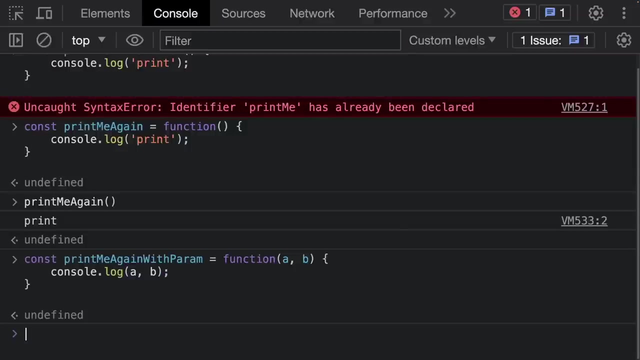 with param what I can do now. I can actually put any parameter here right. this time I'll put two parameters, a and b, and here after coming I'll be actually doing a and b. I have done now, declared it. now let's say, print me again with param if I do 10 and 20. 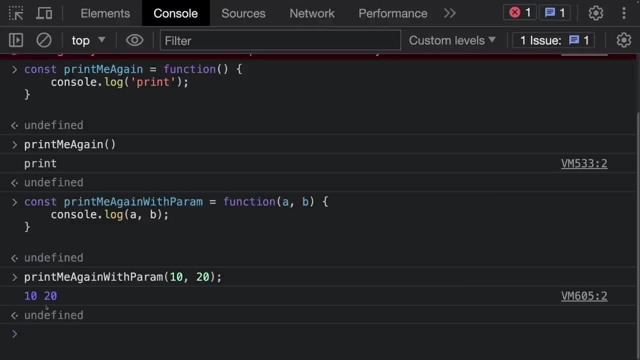 as an argument, is going to print 10, 10, 10 and 20.. So I hope this is clear and now you know, like, how we can actually define a function or declare a function. there are two ways we have done okay, so one is: 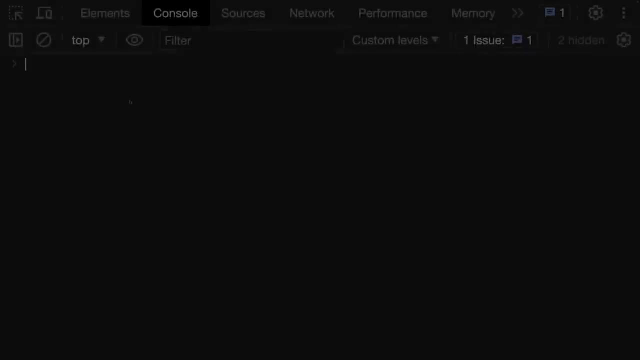 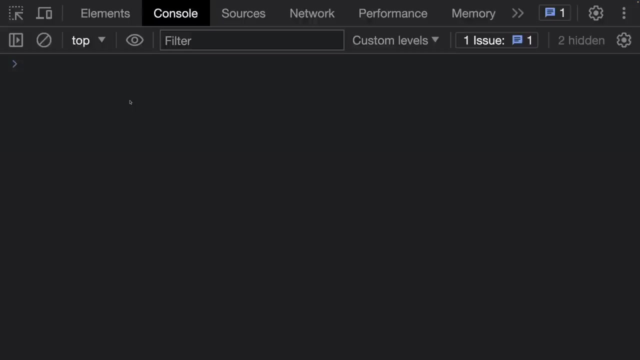 with expression, another is without expression. let's learn how to return from a functions. so return is something you will be using very often when you work with functions. so far, what we have done: we have created a function, but inside that we have just done a consolelock statement which is: 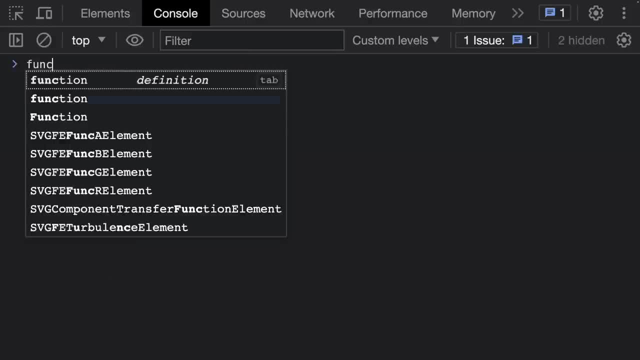 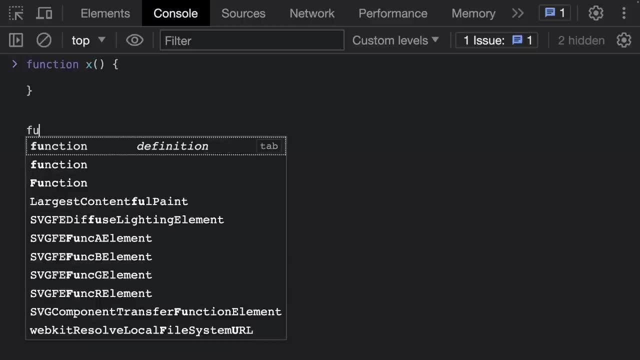 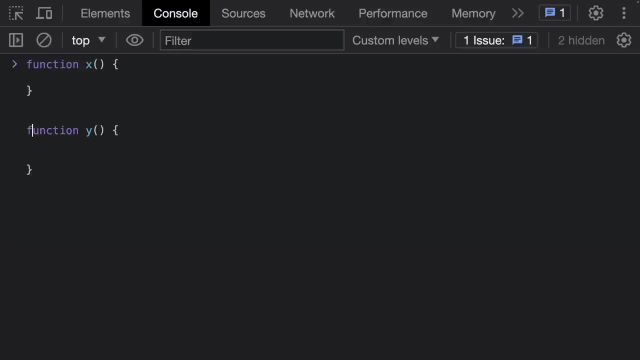 not enough. Usually what happen is like when you create a function like, say, function x, and you have something over here, right, and then you will have say, another function y- okay, and you have something over here, and then each of these functions are supposed to do their own task, right, and in the 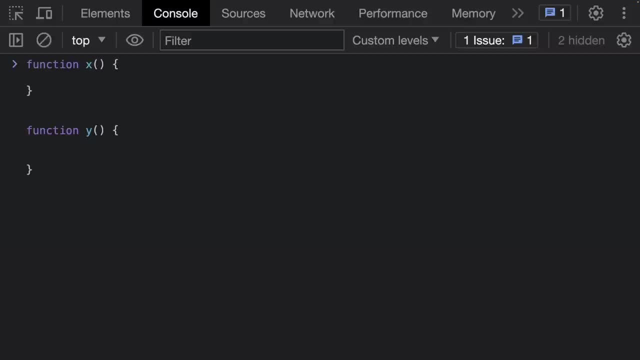 entire program or entire application is not like that. you will have only one function, you will have multiple functions and what we'll be doing is like, if function x, whatever is supposed to do, what you can use is basically, you can use it like the output value of function x and take this into. 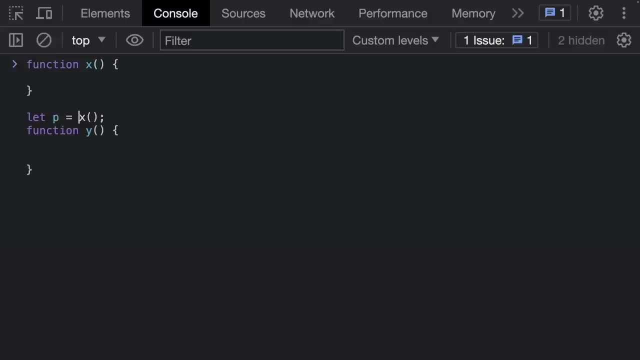 a variable like, say, let, p equals to this and basically can use this p somewhere inside another function or anywhere else that in that matter. So basically, whatever the value of that x function that returns, you can utilize that value anywhere else, maybe in another function or anywhere in your programming right. 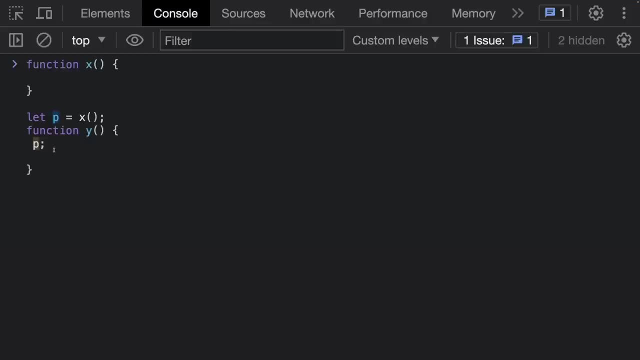 so that is, that is, that is very much a feasible thing in and the thing that you will be definitely doing Now, this thing to happen. if you see this expression, let me remove everything over here and just to put this for your consumption, this particular expression: what we are doing, we are 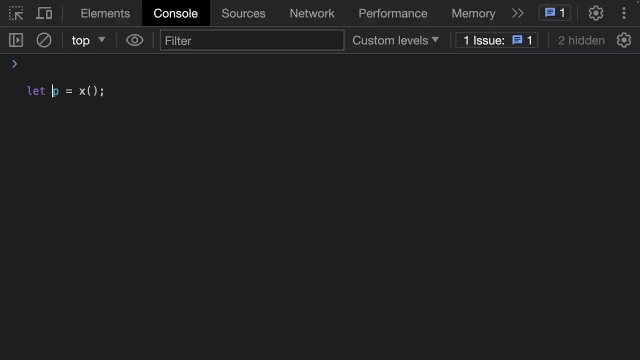 having a variable called p and the p's value is what is not the function, but the value we get from executing a function. Because we told a function name along with a parenthesis means executing, calling, invoking a function. a function name without a parenthesis means it just the string representation of the 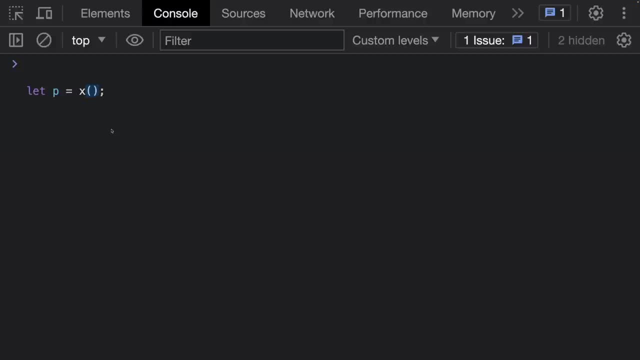 function definition itself. this is a. this is a difference that you have to keep in mind. So in this case we have parenthesis means the function will execute, function will be called or function will be invoked and, within that, if the function is returning any value, if the function 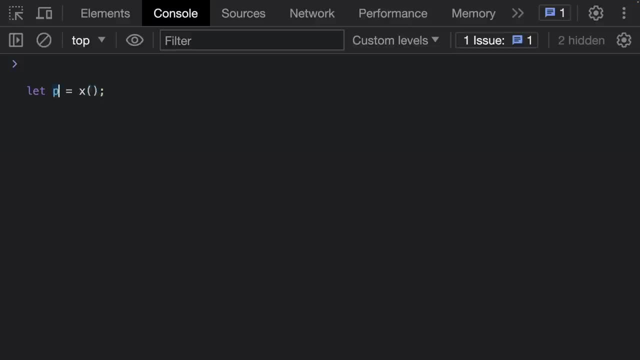 is returning any value, then it will be called parenthesis and that is the function name: any value. that value will be assigned to this variable. what if the function doesn't return any value? what if it just has a consolelog, like we have seen the function so far? in that case, simply, 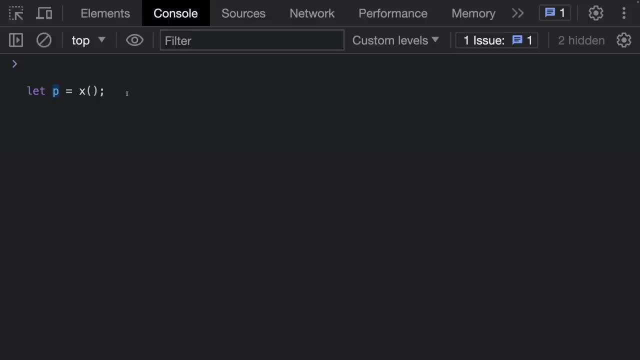 the function execution will return something very special, which is called undefined. okay, it means that something that is not defined yet is something called undefined. okay. so now let us create a function that returns something. so for that we'll create a function: say sum and we'll do a summation. 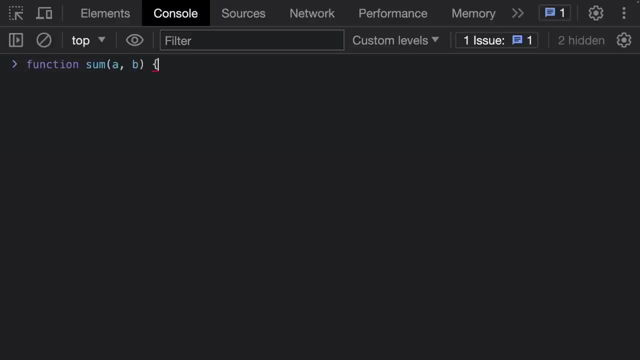 addition of two things. so we'll take a and b as two parameters. terminology matters and what we'll do is like we'll do return of a plus b, simple. so it means that this is a function whose name is sum, takes two parameters, a and b. it sum up those two parameter with this arithmetic operation. 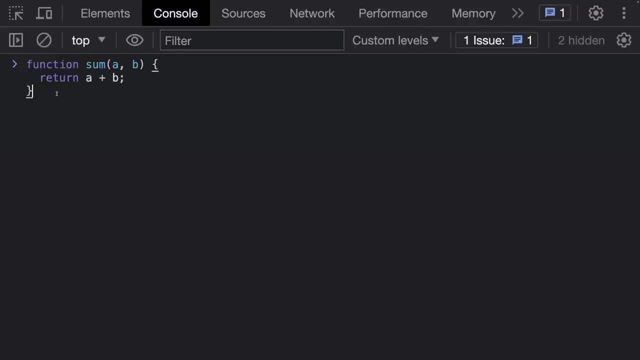 and the result: it returns sum. you know back, so let's execute sum. it takes two arguments. now let's put two and three. it means we are expecting a five. it's returning a five in the same method. we can actually write little bit differently, how? so let's write the same method: function sum. we will do again a comma b. 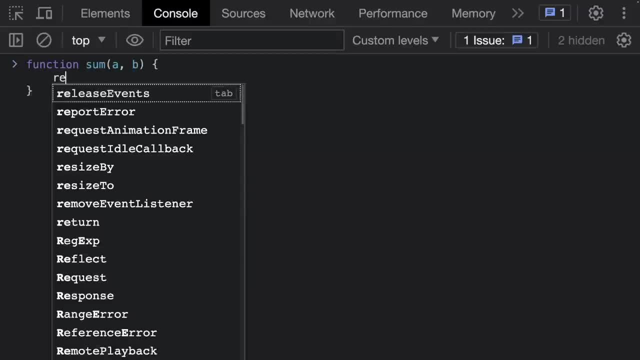 and in this case we just did return of a plus b instead of that. some time you might want to do this also, like let let turn a variable, a plus b, and then return that particular variable itself. that is also same thing, same as you know. we have done what. 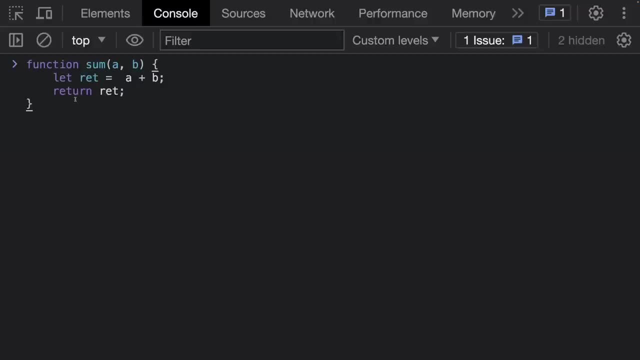 would have done before, like returning a plus b directly, right? so if it is just a simple calculation, returning it directly itself will be a shorter amount of code that people does, so please follow that. this is about returning- returning from a function. It means everything that you do inside a function, all the tasks. 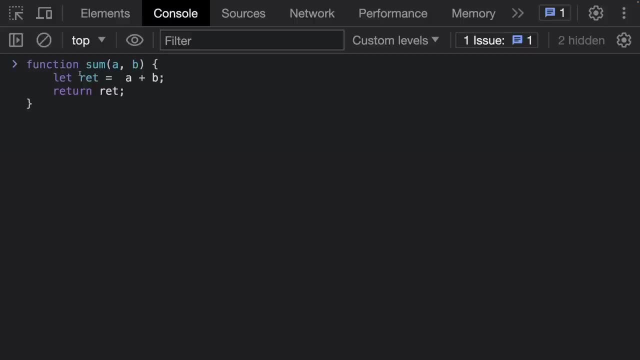 all the logic, all the operations and, at the end of it, if you want the function to return a value so that that value can be utilized elsewhere, you have to use the return statement, followed by what you want to return. I hope this is clear. 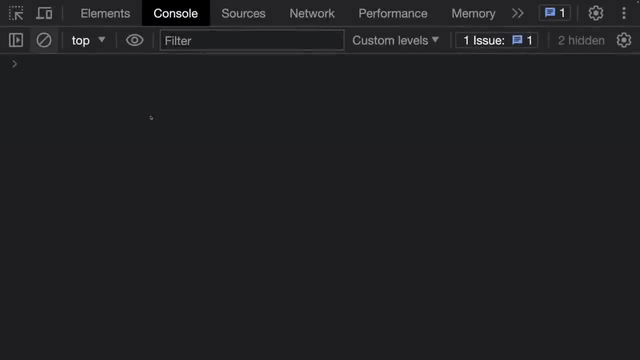 What is default parameter When you define a function? we know how to define a function, So let's define a function. Function will take the same, okay, a little bit different function. Let's say calc is a function and it takes two parameters, a and b, and what we do, we will return. 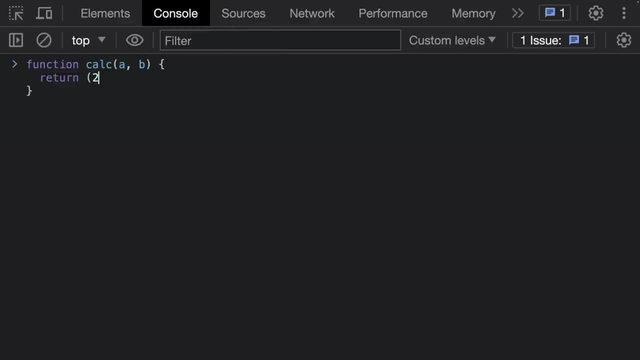 some value, and the value that we want to return is something like 2 into a plus b. okay, This is the value we are planning to return. So what does this function do? A simple function, A function whose name is calc Takes two parameters, a and b. What it returns is first sum up these two parameters: value. 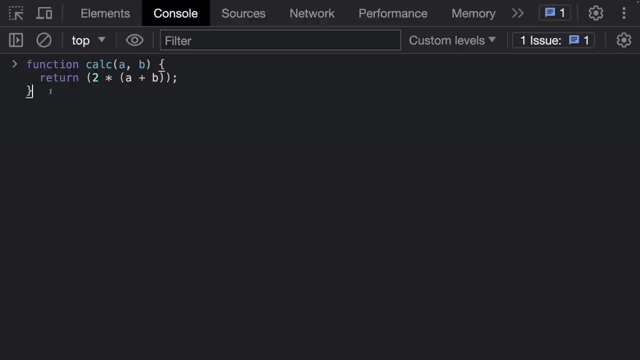 then multiply it with 2 and then return something back, a value back. So let's execute this, Let's call this function with 2 comma 3, all right. So what it gives you, It gives you 10.. Yeah, 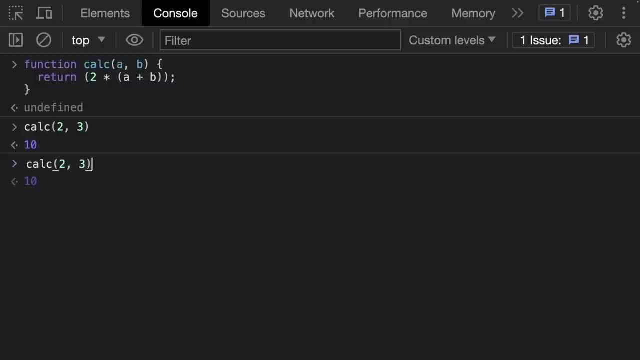 of course, because 2 plus 3 is 5.. 5 into 2 is 10.. Similarly, you can go do 3 into 3.. What is going to give you 12.. 3 plus 3 is 6 into 2 is 12.. Now let's say someone. 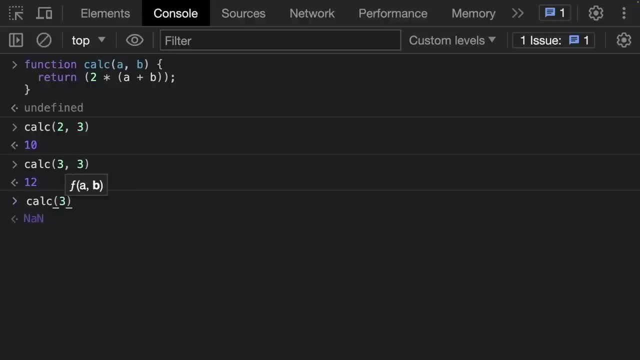 in the team forgot to pass this second argument. What do you get? You get not a number. Why do you get a not a number? Because when you don't pass an argument for a parameter for the function, the parameter value will be undefined. We told about that. So it means that in this case, 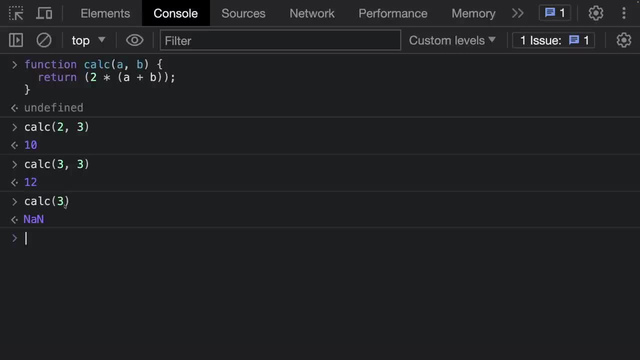 you are not passing the second argument. So value basically. so then b will be undefined. Now a plus undefined a will be 3.. b is undefined. 3 plus undefined is not a number. Of course, it returns not a number. 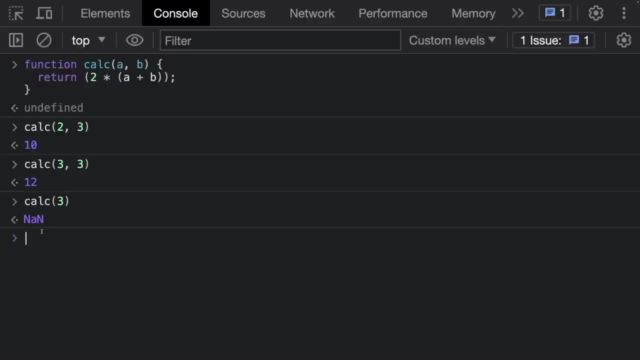 Now, in a situation like this, instead of getting not a number, you might want to safeguard it with some kind of default value right, Some kind of default value of these parameters, so that at least this won't fail like this. Rather, you can safeguard them with some values of. 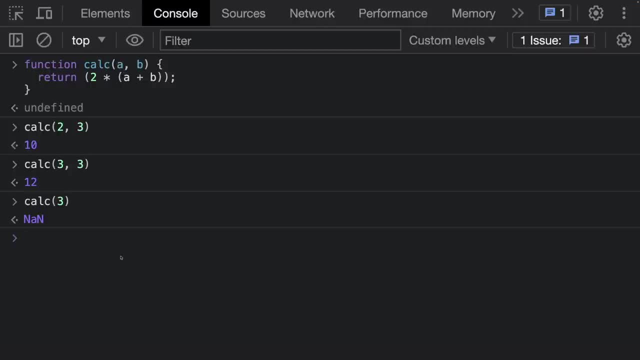 you know something that you are liking, okay. So what we're going to do? the same function I'm going to bring in again, And now I can actually default it to 0, okay, It's a default value, or default value for this parameter. 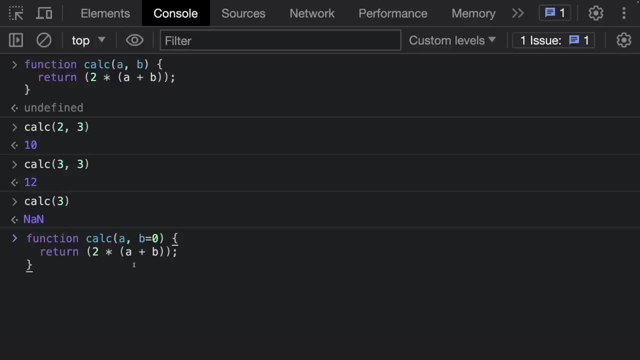 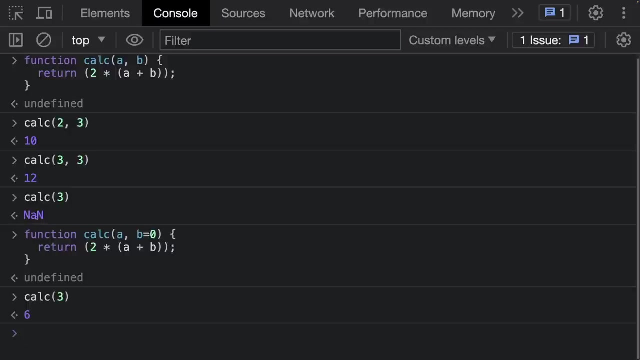 that I'm putting. So it means, if someone is not passing a value for this parameter using the argument, the value 0 will be used instead. okay, So let's do this Now. I'm going to do calc 3 again, If you see this, now, instead of nan, not a number, it is actually returning a value which is 6,. 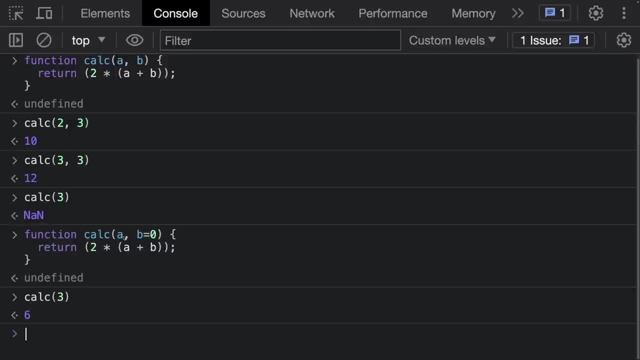 which is, let's do the computation: a is 3,, b is 0, 3 plus 0 is 3, 3 into 2 is 6,. okay, So you can do a default parameter value for your function if it's required to, And in that case you can safeguard it from an unnatural value. 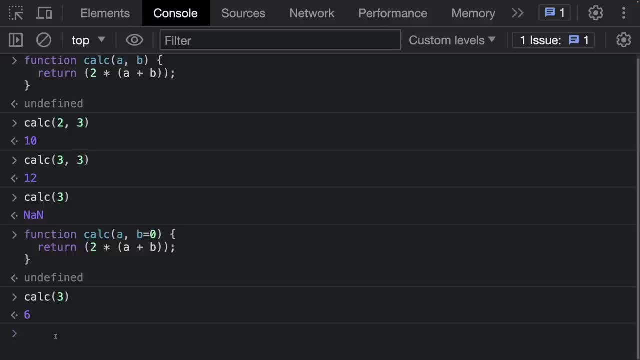 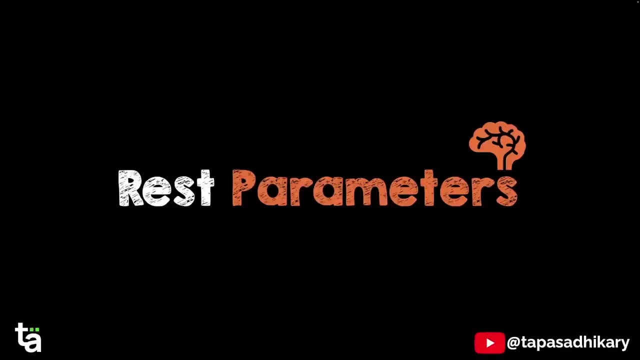 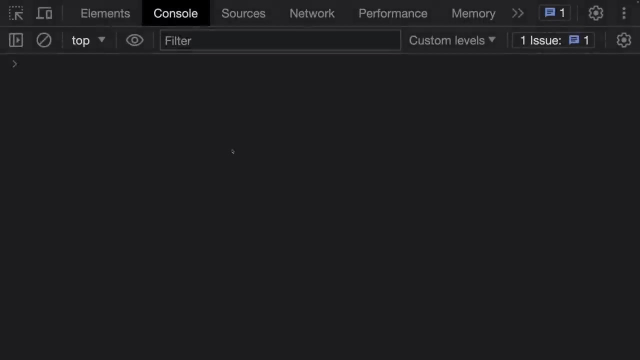 return value from the function, like not a number, And you can actually override the undefined value. Instead of having undefined, you can now set certain value with the default parameter: Rest parameters. What is rest parameter? So the rest parameter is something that allows a function. 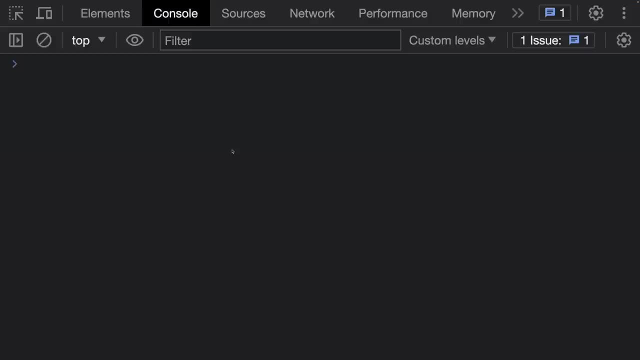 to accept any number of arguments as an array, any number of arguments. okay. Now, theory is one side. Let's do it with example. Let's create a function. Let's say, give a function name. We'll give a name called, say, collect things, okay, And we'll have two. 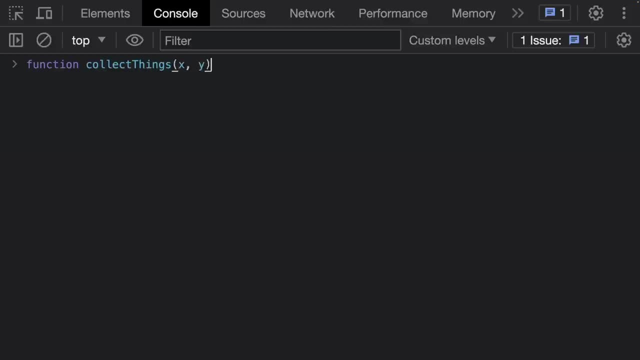 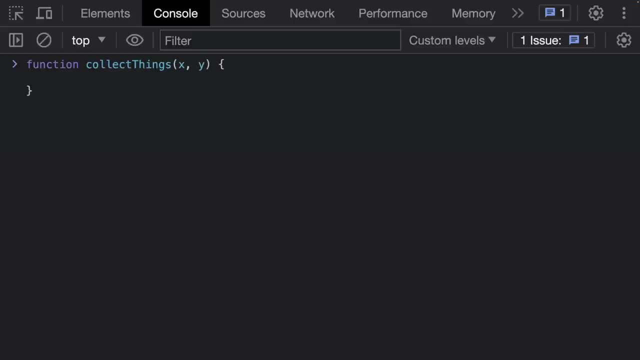 a different kind of special parameters. right, We know about default parameters. now, Now we are learning about the rest parameters, And I just now say the rest parameter allows a function to accept any number, an infinite number of arguments as an array. Now, to make sure the 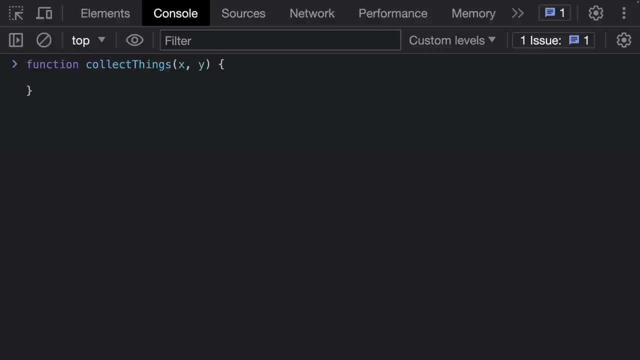 rest parameter accept an infinite number of arguments. what we have to do? we have to give a special syntax to it. The syntax is: we are going to give a function with three dots. So when we give three dots, what happen is like: 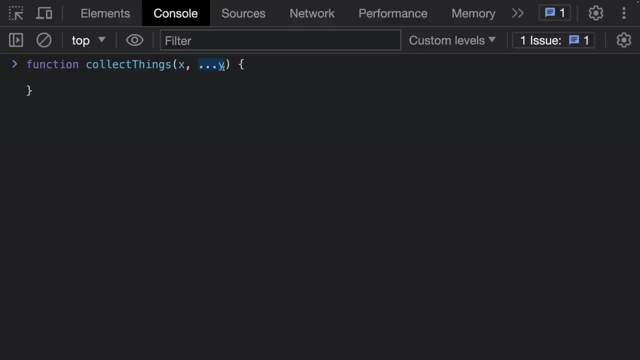 this, this: this particular parameter become rest parameter. Now here two things I want to call out. A function definition can have only one rest parameter. So it means that you cannot do x rest parameter, y rest parameter, z. You cannot do that, So it can have only one rest parameter. 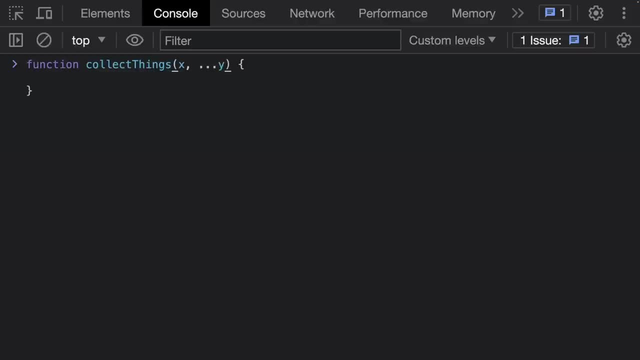 And the rest parameter must be the last parameter that you define for the function. These two rules please keep in mind. repeat again: a function definition can only have one rest parameter, as we have over here with y. the rest parameter must be the last parameter, like how we have here. so you cannot have, like you know. 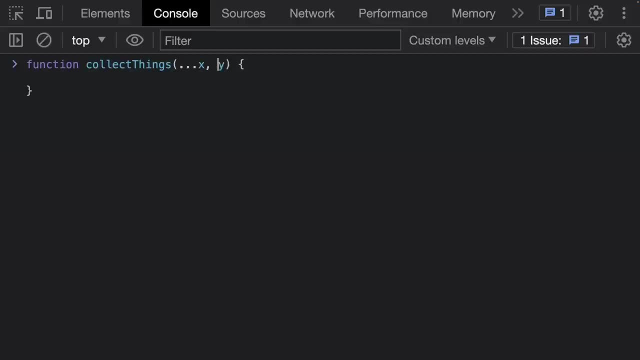 making this x as a rest parameter and then y as a normal parameter. you cannot have that. rather, you have to have like this. of course, the name suggests it means rest. rest means rest of it, rest of it means whatever is left over, so that is where it goes at the end. okay, now what i'm going to do. i'm 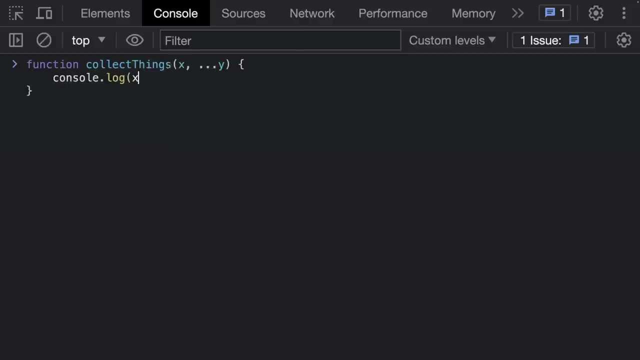 going to do a console dot log of x and then i'll go do console dot log of y so that i can actually print and see like what exactly it prints. now i have defined, let's just do collect things. sorry, let's just do collect things and then pass. 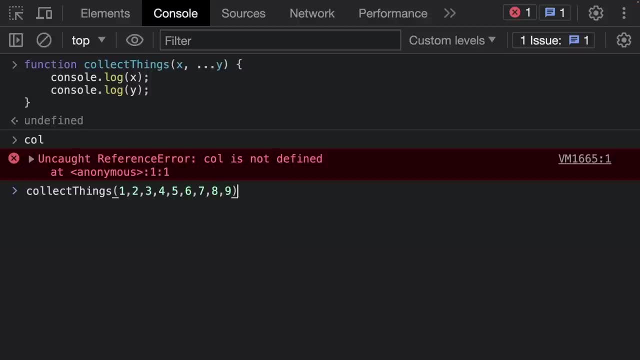 arguments: any number: five, six, seven, eight, nine, okay, nine, enough. now what i'm going to do? i'm going to call collect things with nine arguments. i can pass hundreds thousands, millions, if i have time. okay, so let's test it with nine. so what will happen? the first argument that gets mapped to the 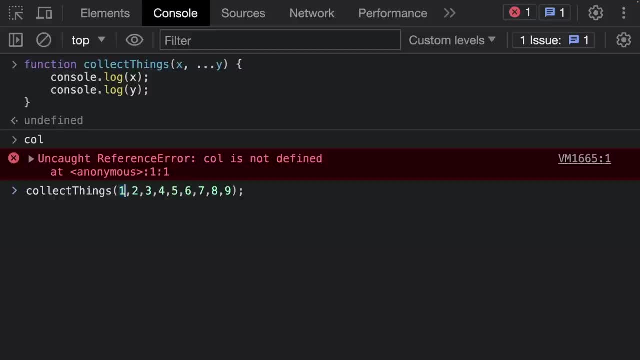 first parameter. so x value will be one and the rest of it- two to nine- goes to the rest parameter. so it means y will now accept from two to nine, but within an array. okay, so if i just printing it, so if you see the first sprint, x is one and then rest. 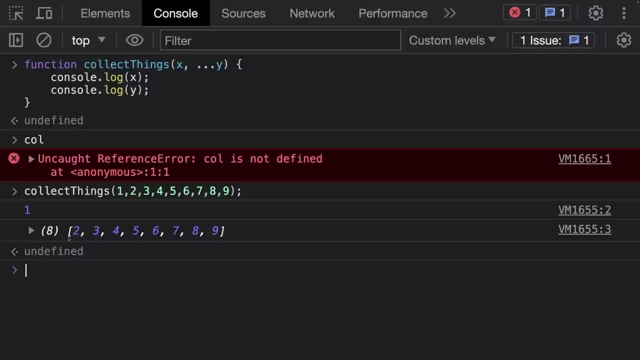 of the eight goes inside an array two to nine. this, this subscript, is a array notation two to nine and that that get assigned. this entire array get assigned to this y parameter. that's why it's called rest parameter. hope it was again easy for you to understand and you will try to practice a. 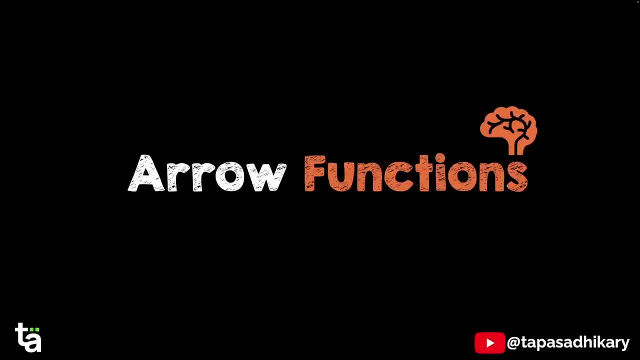 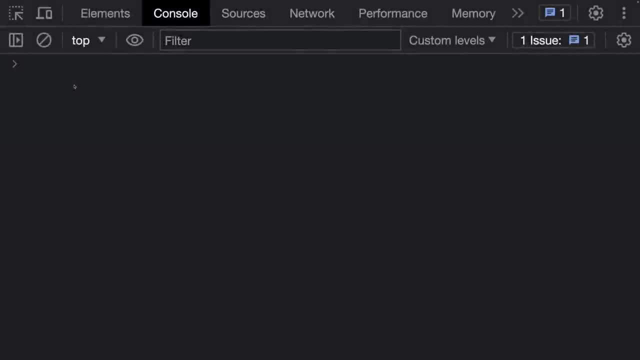 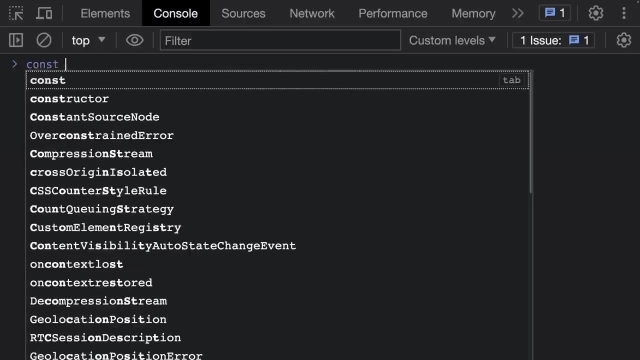 lot about the rest parameter. let's learn about arrow function or fat arrow syntax. all right, so we know how to define a function, right. let's do it again, but this time let's repeat the one we did with function expression const, add equals to of function, and then we have two parameters over here, and then we 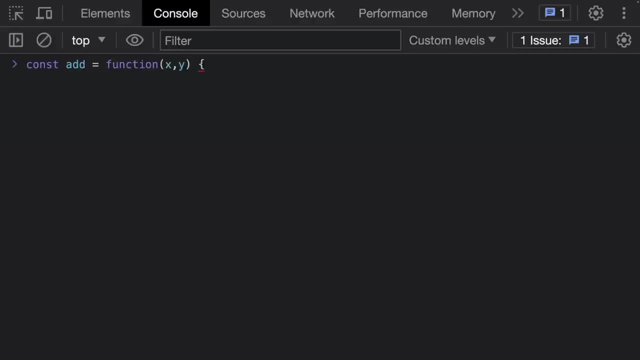 have return of x plus, and then we have return of x plus, and then we have return of x plus y and finally we close this particular breast. so that works. that's great right now, what we can do over here to convert this one to a arrow function or fat arrow syntax. there are few adjustments that. 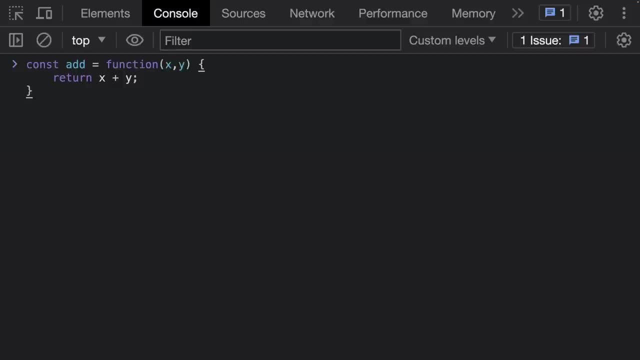 we have to do so. initially, the arrow function or the fat arrow syntax looks little weird, but how. i try to kind of remember writing it, and right now what happened is like i hardly write a function in the regular definition or declaration way. it's always about writing the function with the fat. 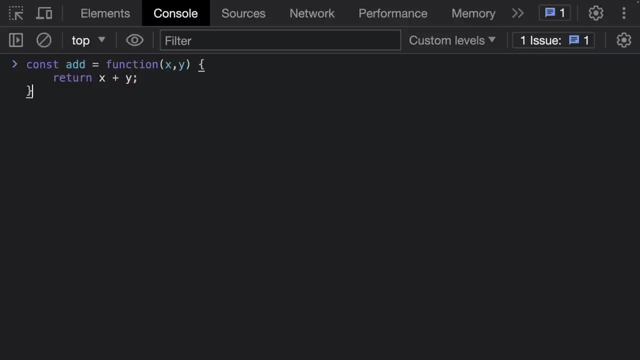 arrow syntax or the arrow syntax- okay, so let's convert it. if you're new to it, you will take some time to get a grip on it, but once you get a grip on it, i'm sure that you are going to write the arrow function again and again, because now i'm coming to the usage of it, because the best use is. 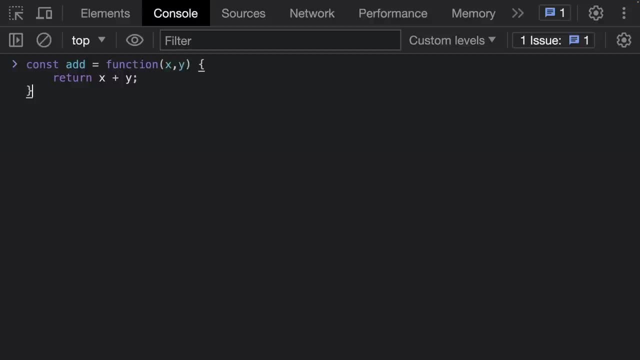 you will write less number of code. you will write lesser amount of code, and be it any framework or any library. today, in the modern web development, i think the de facto, the very normal coding syntax for function is using arrow function. it doesn't mean that you cannot go with the traditional way of declaring and defining. 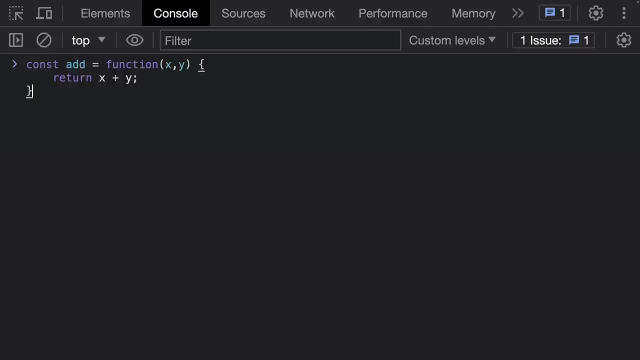 function or declare or define functions using expressions like the one we see on the screen. you can always go with that, but if you use arrow function or you use fat arrow syntax, it's, like you know, much more modern. it's much more less code. and, of course, there is one more thing that 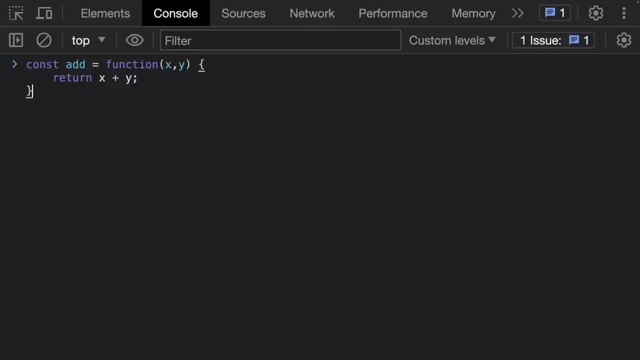 is there, which i won't be covering in this crash course, in the but, but in the following one: the relationship with the this keyword and arrow function. arrow functions: no binding to this keyword. that is what is another special case that comes, but that will be covering into the. 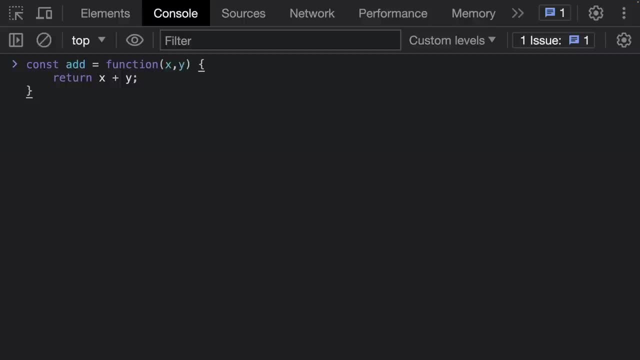 this video, the this keyword video that i'll be making next. okay, but let's now focus on how to convert this one to arrow function. okay, so to convert this one, what i have to do- simple thing one- is i'm going to remove this function keyword, so you don't need function keyword at all to make an arrow function. next we 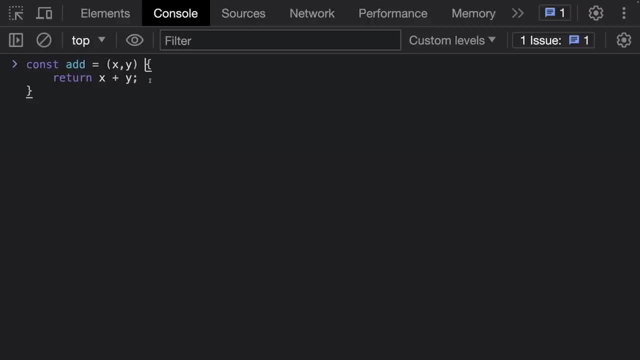 are talking about this arrow function, so you need an arrow. so arrow is a combination of this equals key and this greater than so if you have a greater than and the equals and the greater than key, without any space side by side, you actually have an arrow like syntax, and this is what is making 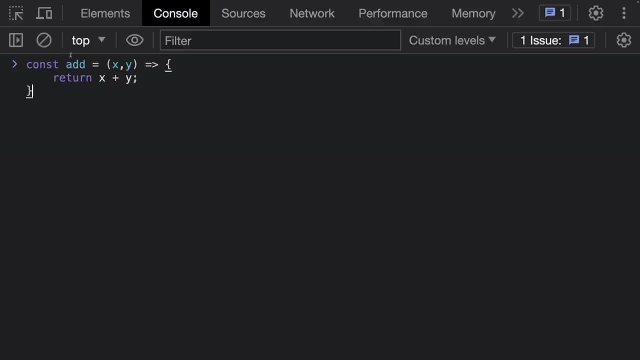 is an arrow function, so this is an arrow function. okay, const add: this is the parameter that we are going to be using. and then what is happening? basically, i am having an arrow and then the definition of the function. that's all about the arrow function, so i am not using the function. 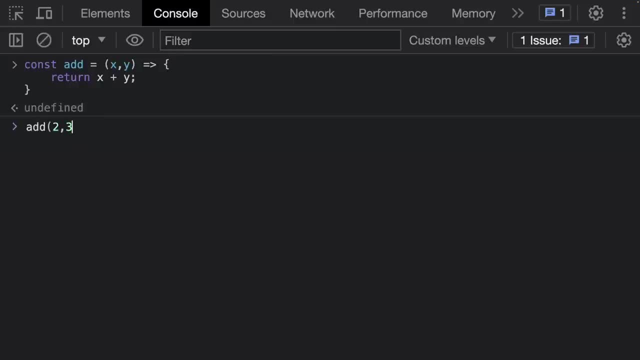 keyword at all. so let's just make sure that it runs two comma three, it runs five. okay, very good. but one more thing that i can do: if the arrow function body, the arrow functions declaration, having only one statement, just one line and one, and it's returning something, 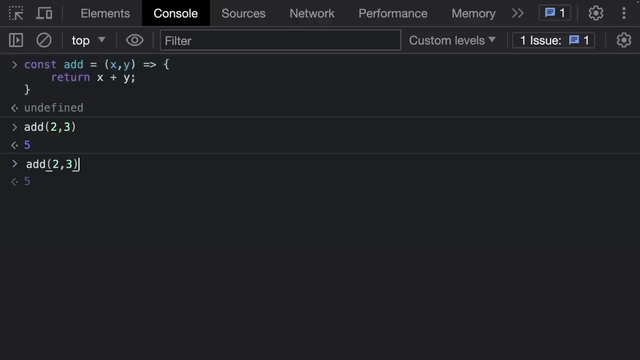 and you can even give this. you know curly braces, so this one you can very well define like: you don't need this, just get rid of it. and then you get rid of it, that's it. so this syntax, compared to this one- you know the with the function keyword, this is much, much simpler, isn't it? so if you have, 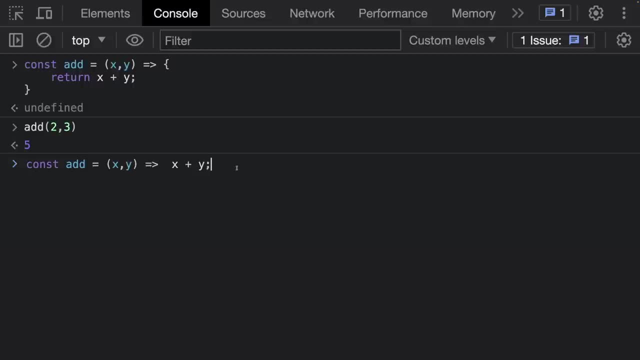 a syntax like this it is. it is way, way easy for you and if it is something like you know, you have dependency with just one parameter over here. you don't have to give it a name and you don't need to give this parenthesis. you can actually do things like this. so if you have, you know, just one line. 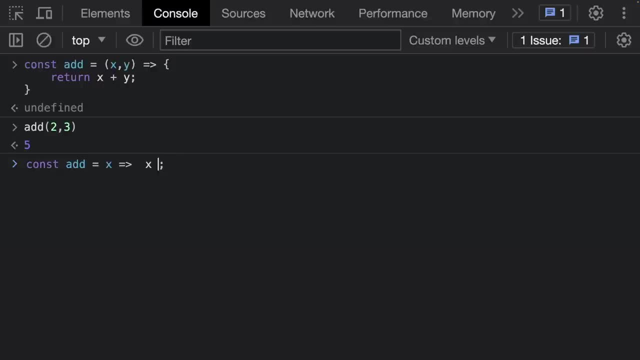 stuff over here. so it's much, much simpler. so this is the reason why our arrow function is very well depreciated, you know, appreciated- sorry, very well appreciated- by the developer community. it is very well received by developer community because you will be writing very less syntaxes, very less code. 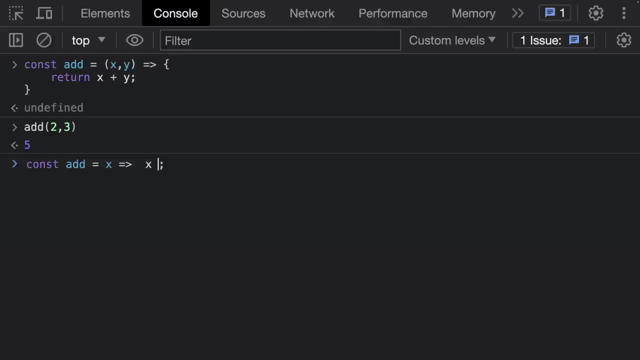 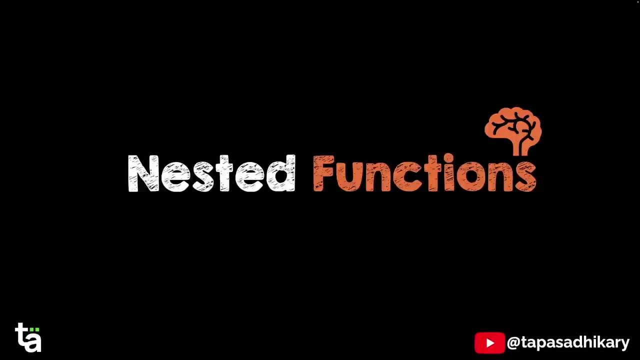 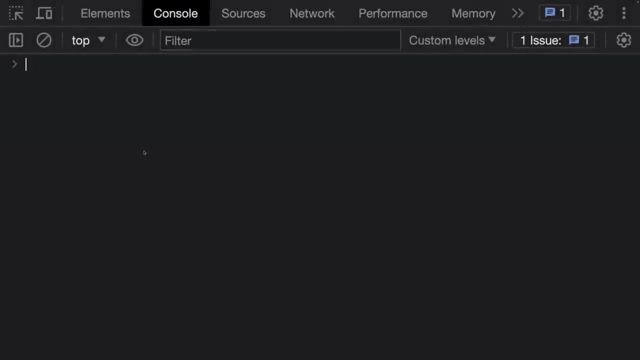 and in all the modern uh web development- uh, you know area- the arrow function is used very heavily. so please practice writing arrow function and i hope that you keep writing more and more arrow function in your code than writing the function in more traditional way. all right, so nested function: what does nesting means we know how to create a. 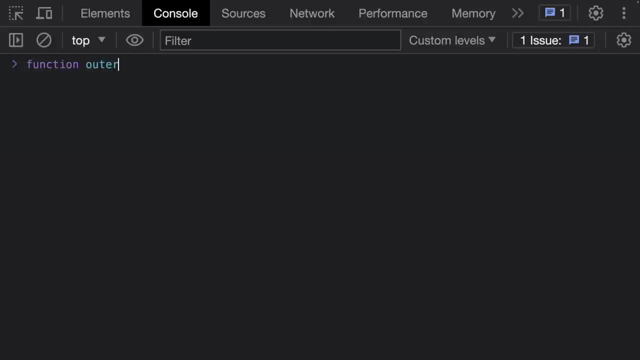 function. let's say we create a function called outer and that function has a body and it can have certain instruction like: what is this function supposed to do? maybe in this case the function is supposed to print something called outer into the log. now javascript allows you to create a function, to define a. 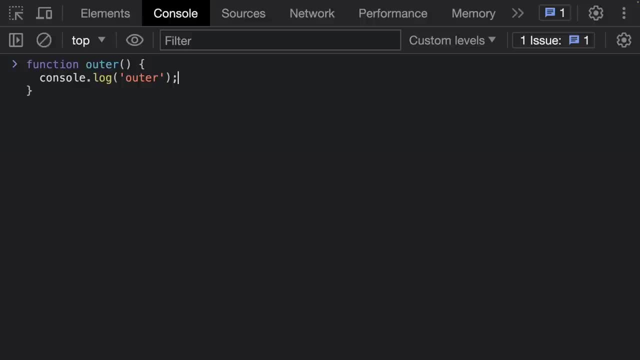 function within within another function. okay, it might sound a little bit strange if you're new to it, but this is a very, very powerful feature and this is the first basic thing towards understanding the concept of closure. the concept of closure in functions. in javascript function equals to the understanding of nested function plus. 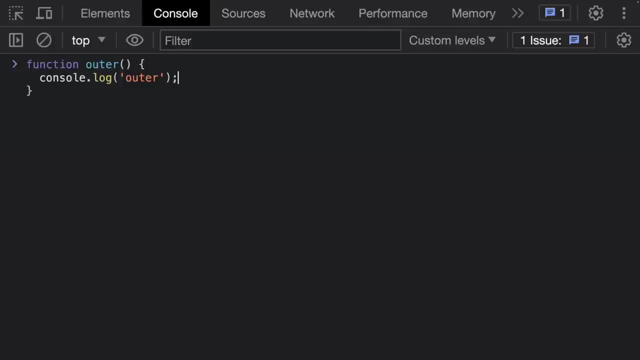 function scope. so if you want to understand closure deeply, i want your attention over here. first understand what nested function is. how does it work up? next we'll be talking about function scope and then we'll be talking about closure, so that everything is very, very clear to you and is 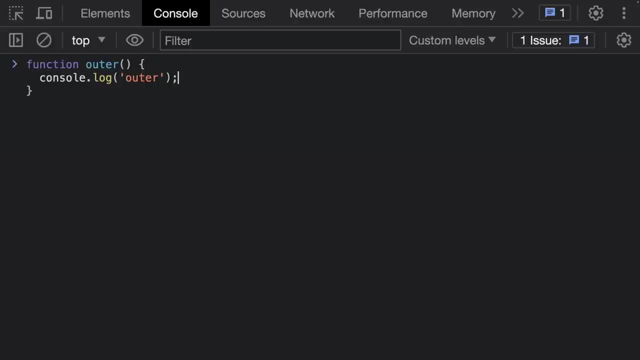 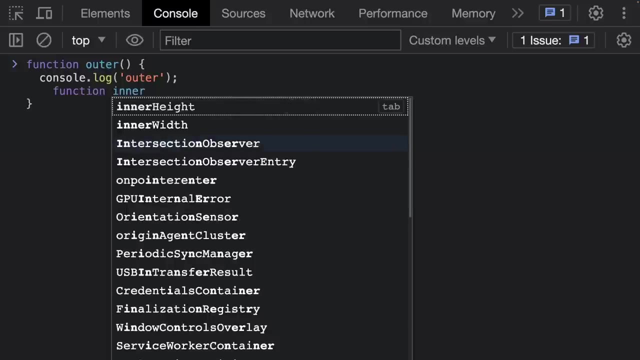 very straightforward to you all, right? so nested function, so function within a function. this means i can create a function within a function. this means i can create a function within a function. function over here. give it a name. maybe for simplicity i'm giving it an inner and i can give. 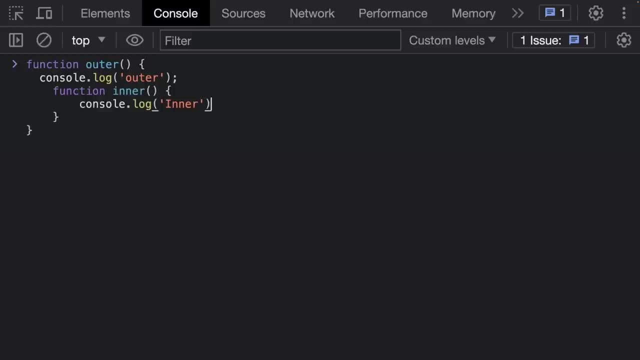 a consolelog. as i've defined this function using the outer function, this function is called a nested function and this nested function, as i've defined outside, you know, inside this outer function, i have to call this one inside the outer function itself. okay, so like this. so, right now, if i have 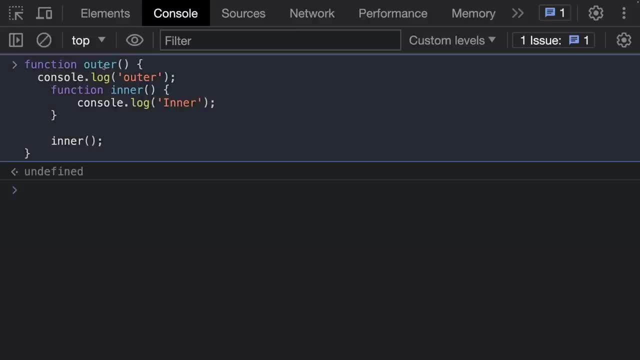 defined it this way and if i call the outer function, what will happen? the outer function will be invoked, it will print this consolelog, then it will see this inner function has been defined, the definition happen, and after that it will invoke the inner function also. so what will? 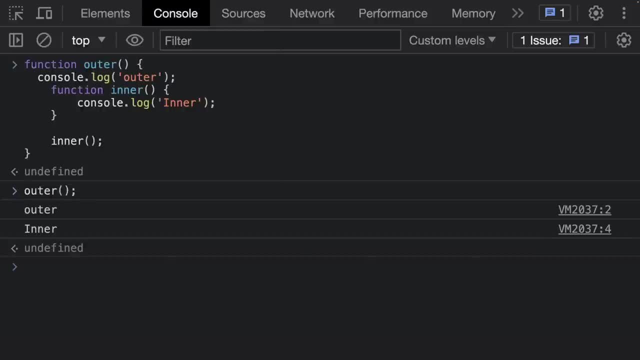 be the output if i do this outer over here. okay, so the output is outer and then the inner, so it first print the log outer and then the definition happen, the inner get executed and this, this inner, actually gets print out. so you can have nesting to any level in javascript functions, however you 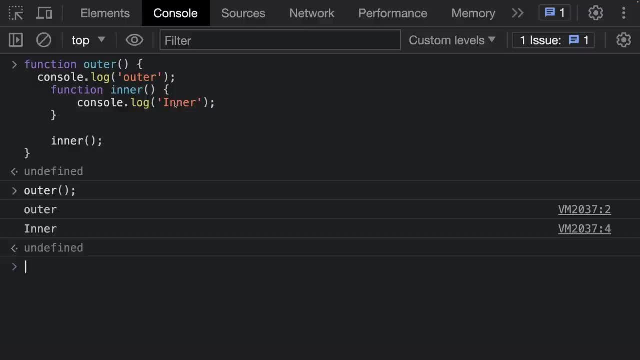 won't see in practice. uh, you know too much level of nesting. but you definitely will see. now, if you go back and see the code, the various javascript code, you'll definitely will see some level of nesting, some level of defining one function another inside another function happening and 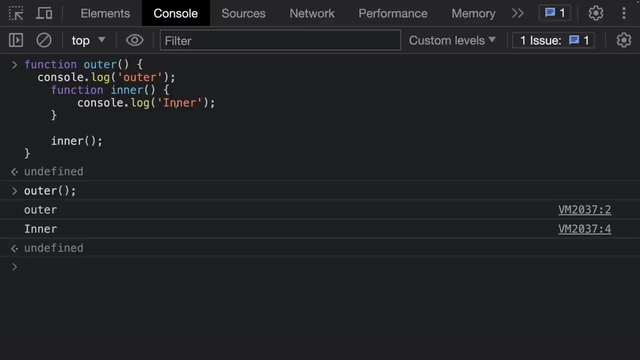 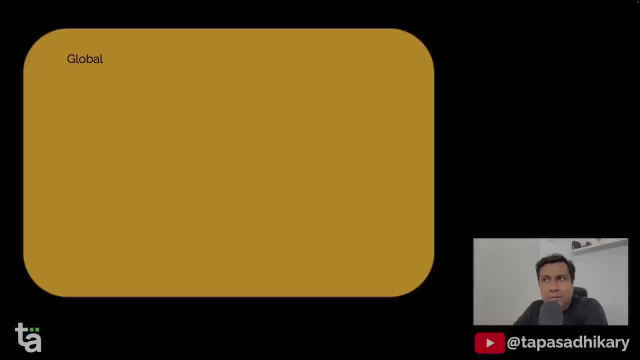 it's a very powerful feature. we'll be able to see this in a moment. okay, just now we have seen what nested function is and now we are stepping into understanding function scope. okay, these two are a bit interrelated because you have to understand the concept of nested function. you can define a function within another function and then the function. 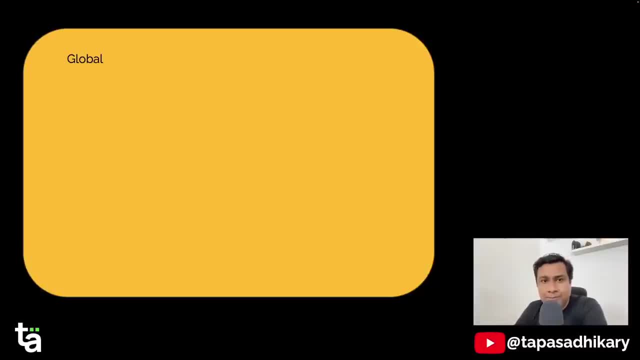 scope is important to understand who can access what. okay, now there are certain generic rules, but to understand those rules, i thought a graphical picture will be much more important, so please pay attention to this graphic over here. so let's say, there is a javascript file, you know, and a function is defined inside that. 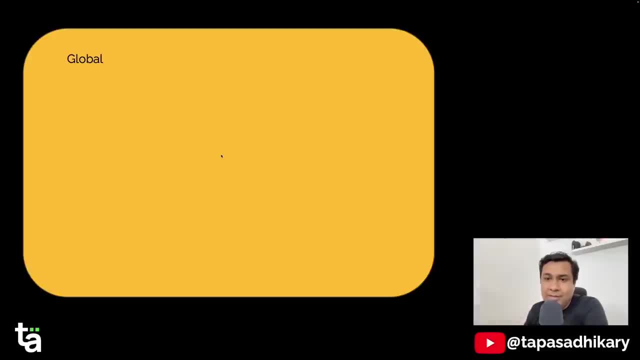 so the function is running globally. it means that the function is not inside any other function. so this blue one is a function. this particular function is not inside any other function. okay, the function is just defined globally. now what happened? there are, there are actually two rules, two primary rules that you have to keep in mind, and these two rules are very important, if you 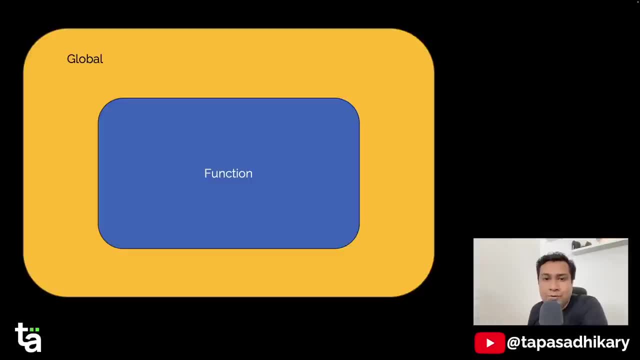 want to understand. i want to understand. closure. okay, so the first rule over here is variable that are defined inside a function. the variable that are defined inside a function that cannot be accessed anywhere outside of the function. okay, so the variable that this one is defined inside this function cannot be. 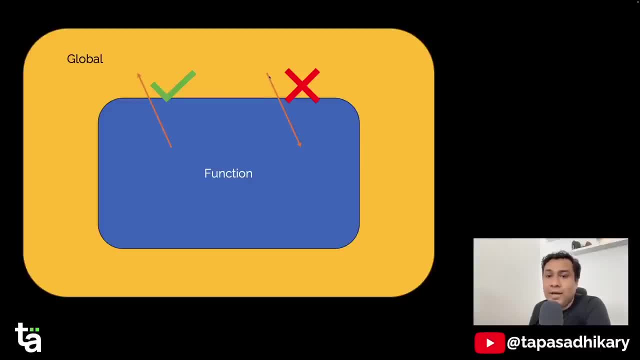 accessed from anywhere outside of the function. okay, so anything defined in this blue box cannot be accessed outside of the blue box understood. first principle, okay, of variable defined inside a function cannot be accessed anywhere outside of the function. second principle: the opposite of it: a function can access all the variables inside the scope it is defined. a function can. 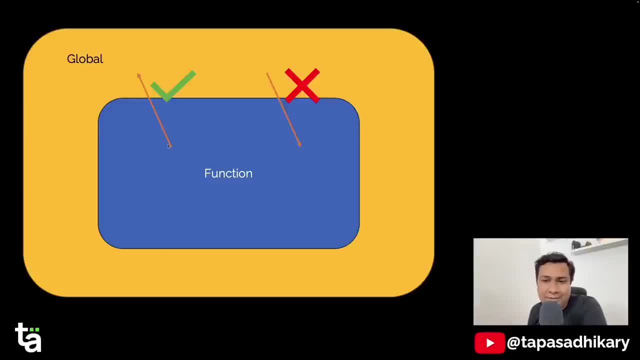 access all the variable inside the scope it is defined. so it means this blue function can access all the variables. that is defined. you know, in the scope the function is defined in the global scope. so inside the global scope if I am defining I'm having any variable, I will be able to access that from this. 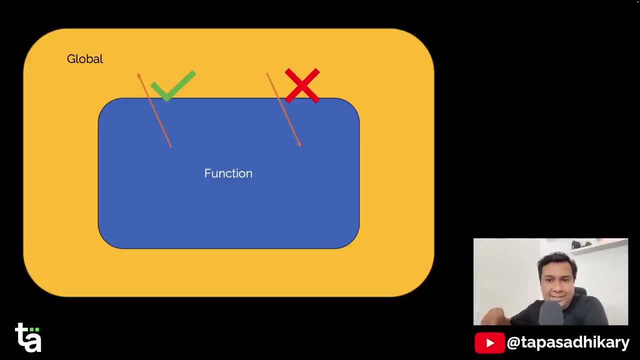 function. but the reverse is not true. from the outside you cannot access the thing which is inside. understood this to rule. let's repeat those two legate because it's very important for us to understand closure: variables defined inside a function cannot be accessed anywhere outside of the function. first, rule. second, a function. 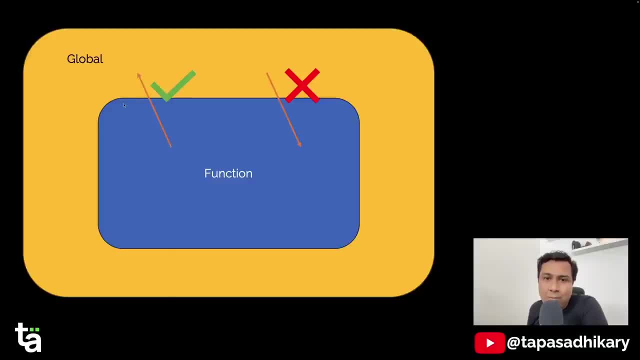 can access all the variables inside the scope that it is defined. so this blue box is defined in the global scope. so in the global scope, if there are any variables from this blue box, the blue function, I should be able to access it. great, now we have learned about nested function. no, so just replace the. 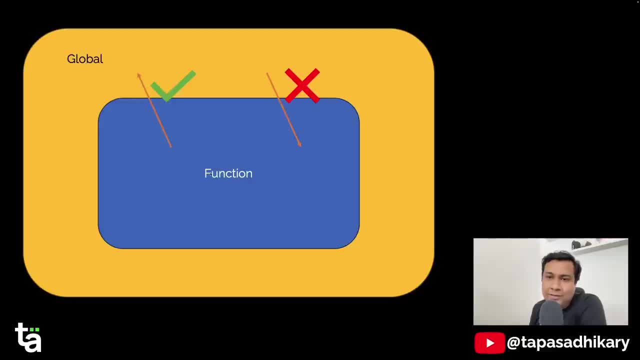 value of the function. right, hope, this is a goodину one. relative to the other series, roof one is defined in the global scope. this class item. what we should understand is when we are having a should be able to access the variable. inside a square is defined only using two form then, while inside repealing. 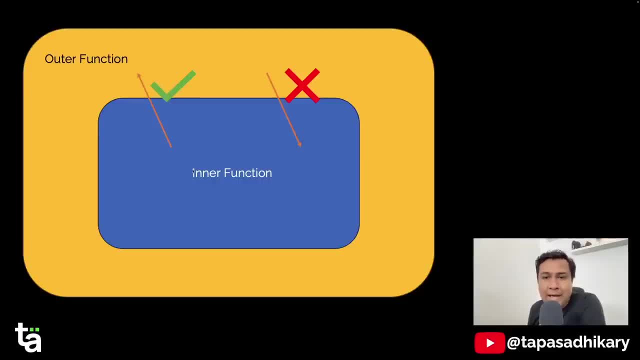 which mean under function. so this is, create this class in the middle section of the initial set of the column, the left columnian, added to the first set of the column- outer function, because inner function is defined in the outer function scope. very simple, right. so now, if it goes, keep going nesting like in. if there is another function, inside is there is another. 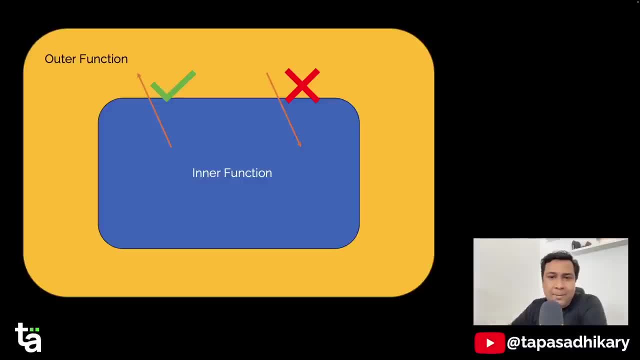 function say: same rule applicable. we have the same rule applied over there, so this is how it works. so you have to keep this thing in your mind. now we are going to see with some code example here. okay, we'll be seeing some code example over here, but you have to really remember this rule, that a. 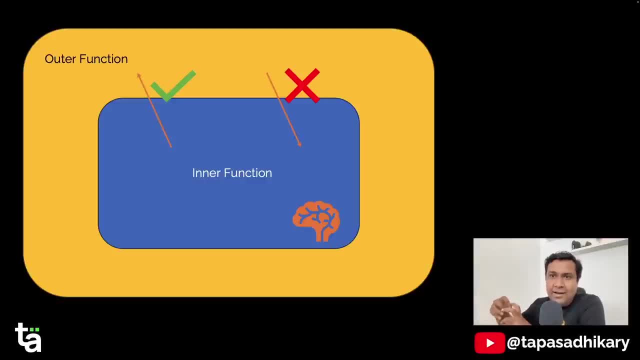 variable defined inside a function cannot access anywhere outside of the function. you know, from outside of the function a function can access all the variables inside the scope that it is defined. so these arrows and these things, if you keep in, keep it in your mind, i think things will. 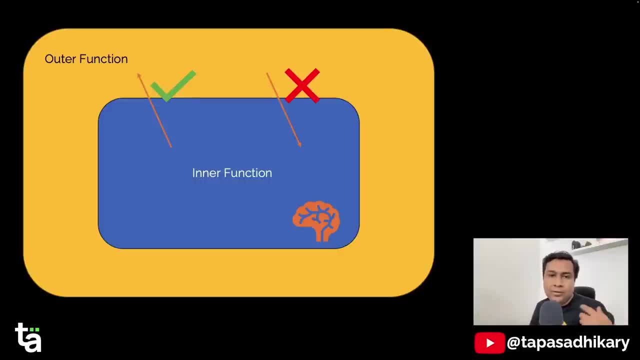 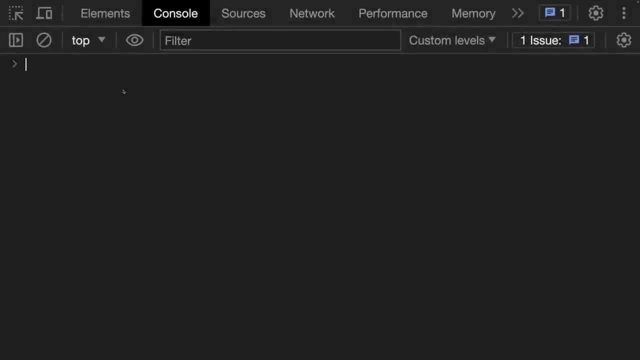 be very clear, okay, so let's move on and try to see, like, how the things works code wise. we'll be doing some coding now. so, based on the rules that we have learned so far, we are going to write the code so that we understand this thing clearly. right, let's create a function. 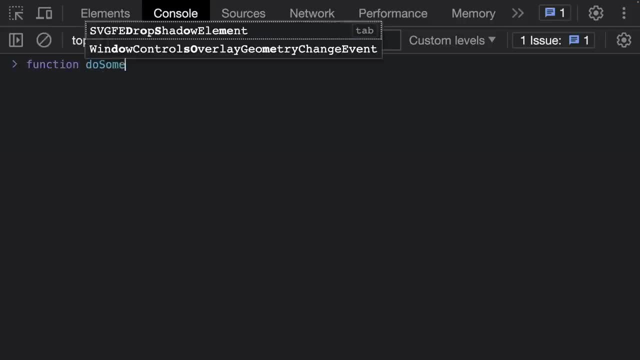 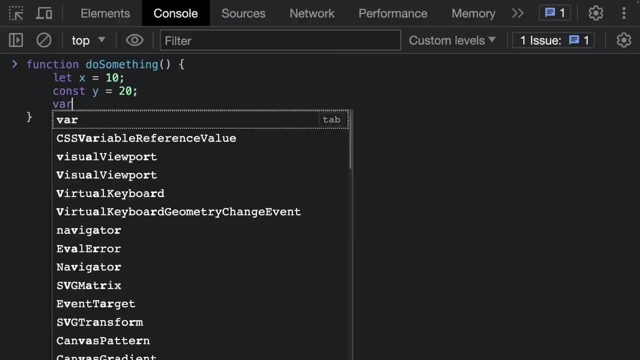 let's create a function called say do something. okay, and what is this function doing? it's basically um, let's create a few variables inside that, okay. so let's do: let x equals to 10, const y equals to 20, and then let const. okay, let's get var z equals to 30, okay, and then simply. 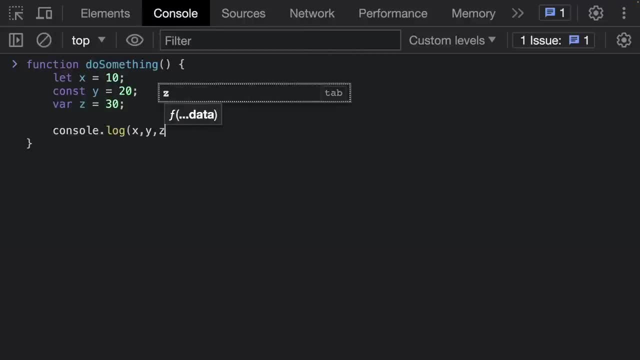 do a console dot log of x comma y comma z. okay, so, we know. if i now do do something, i just call this function. i know what will be. the output is 10, 20, 30, very, very, uh straightforward things that we have created over here. okay so, but this is where our rule number. 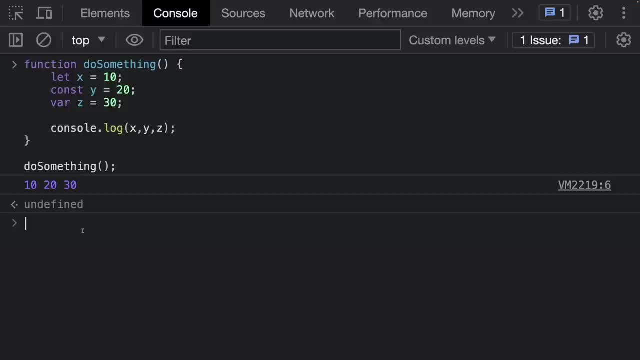 one comes into the picture. what was the rule? number one: variable defined inside a function cannot be accessed from outside right. so it means i have defined let x, const, y, var, z inside the do something function and i've executed do something. it's executed. this console dot log x, y, z. now if i try to take this console, 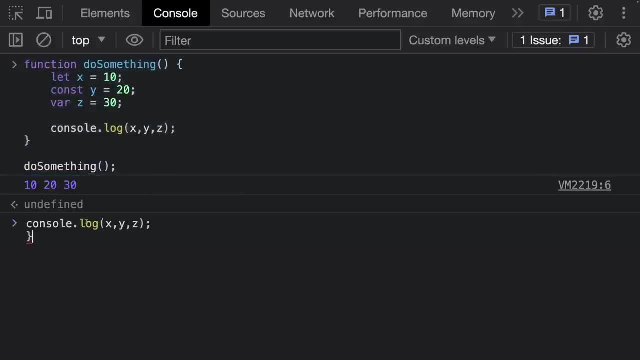 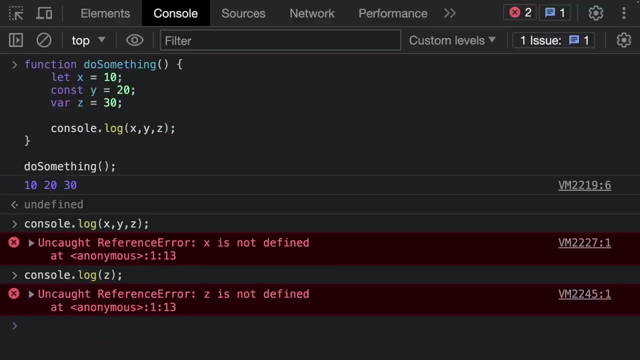 dot log and try to execute outside. what is going to happen? do you see that it says x is not defined. okay, x is not defined. maybe x is late so it's not able to define. y also is constant. how about the var? no, even if it is var and it is defined within a function, you cannot access this variable. 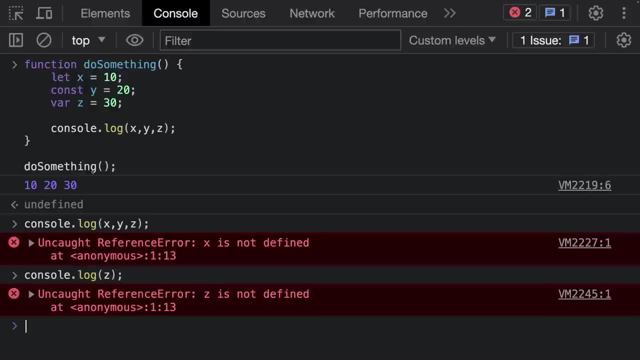 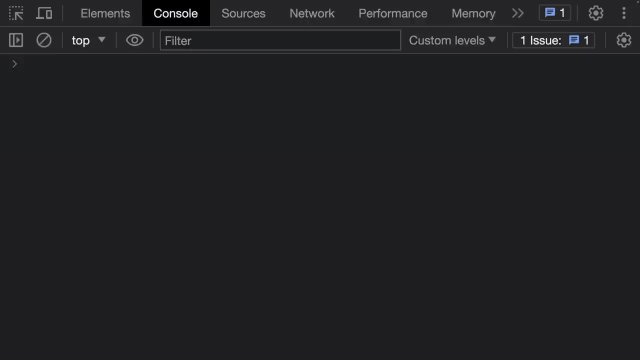 outside a scope, outside of this function, you cannot access. that is the first principle that we have learned just now, right now. second principle: what was the second principle, do you remember? the second principle was about: uh, if the function basically now can access anything and Scope basically the scope where it is defined, Okay, so let's see the second rule now. 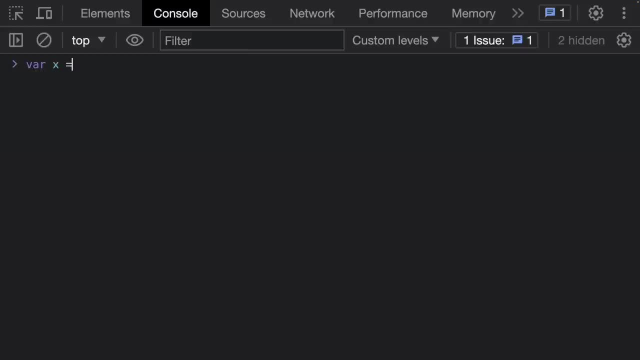 What will be doing? we will be defining var x equals to 10, const y equals to 20, let z equals to 30. okay, now if I do Function, Do something And Do a Console dot log of x comma, y, comma z. what do you think will happen if I just execute? do something. 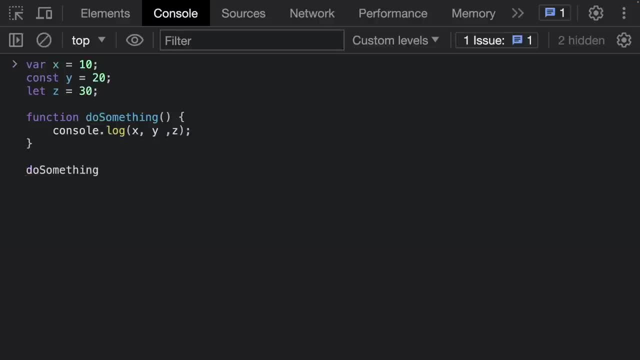 What will happen? Do you think it is going to give an error or is going to print? is going to print successfully, why? Because our second will say: Wherever the function, whatever the scope, the function is defined in that scope. if there are variables declared, the function can access. 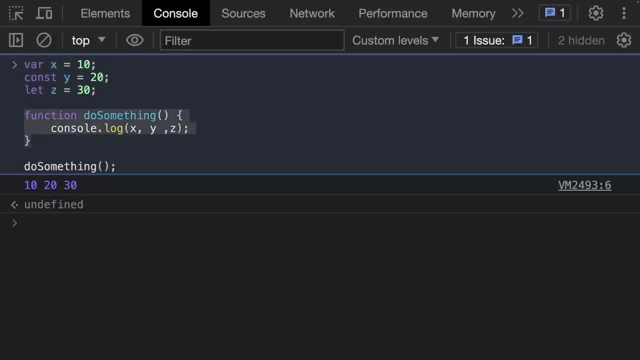 This variable, this function is declared in the global scope. It means that function is not inside another function. So it means if the global scope is having any variables, So the function will be able to access those variables inside the function itself. But when we did the thing other way around, we have declared all this thing inside the function and tried to access them from outside. 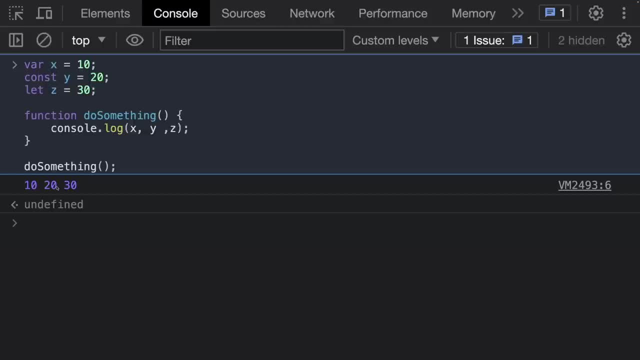 It doesn't work. So these two rules define the functional scope. the scope that we are talking about is the functional scope. you have to remember What is accessible where. simple thing: if it is in the outer scope. if it is, if it is defined in the same scope. 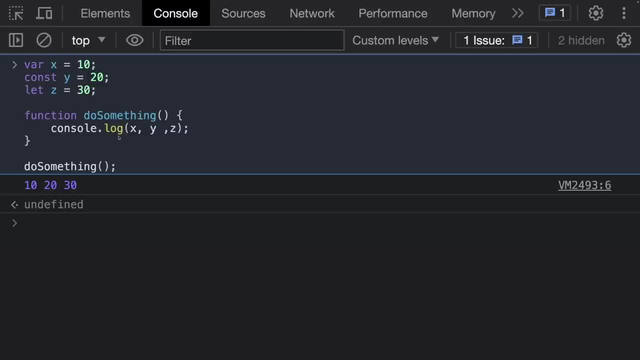 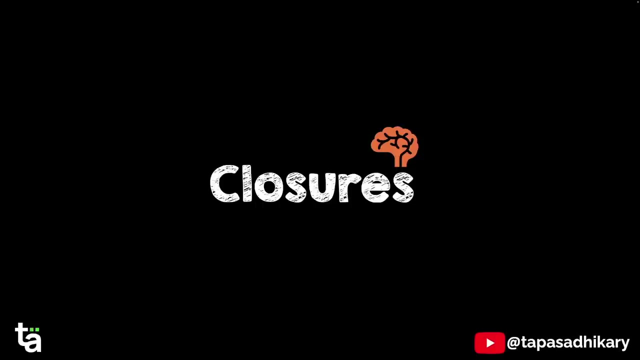 Where the function is defined, it is accessible within the function, But if it is defined within the function, it is not accessible from outside, even if it is a word that is declared and Defined inside the function. clear about it, great. So ask a developer about a complex JavaScript topic. 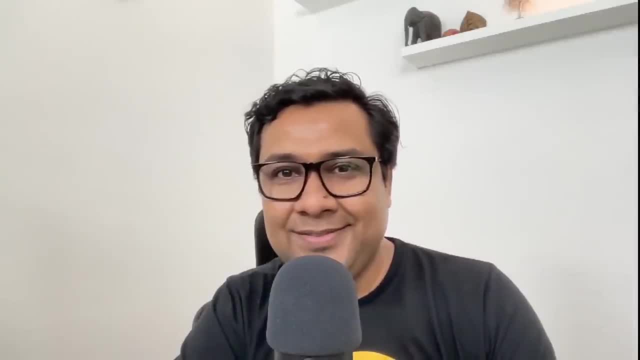 There are higher chances that you will hear back closures. This is because The closures are not understood fundamentally by connecting the dots. Okay, from connecting the dots point of view, If you don't know about connecting the dots and creating a mind map to learn a complex topic, 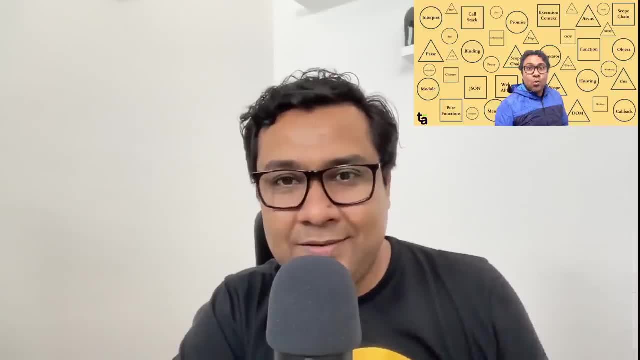 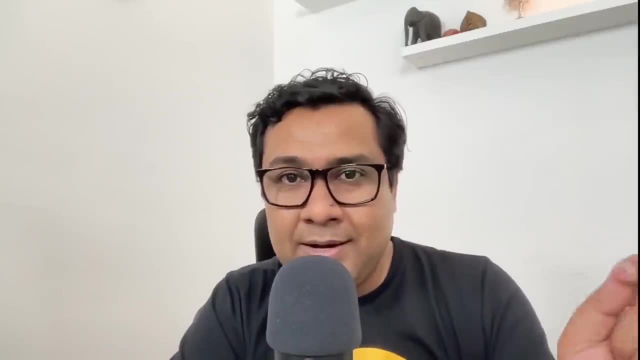 I have created a video on how to learn JavaScript by connecting the dots. Please go ahead and take a look. Now, coming back to closures, if you learn closures by connecting the dots, You will find closures understanding much easy. if you just jump into closure and trying to understand, you may not understand it. 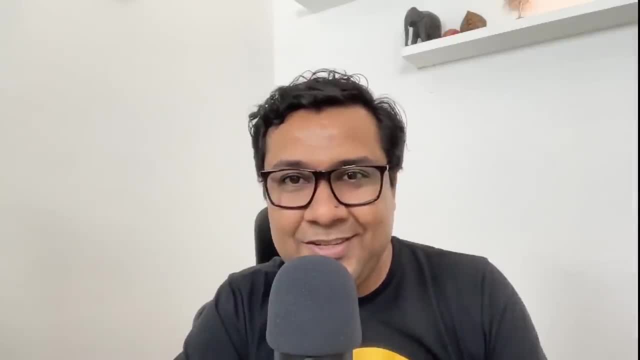 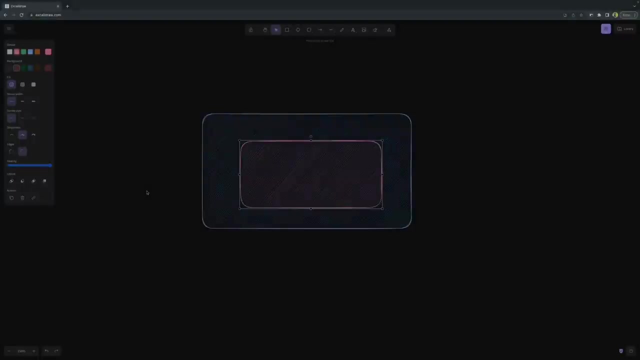 Well, but if you come from the background of nested function, then function scope, you will be able to understand closure very easily. Okay, so let's get into Understanding closures so that we can actually fill it. It's easy. Take a look into this picture on your screen. 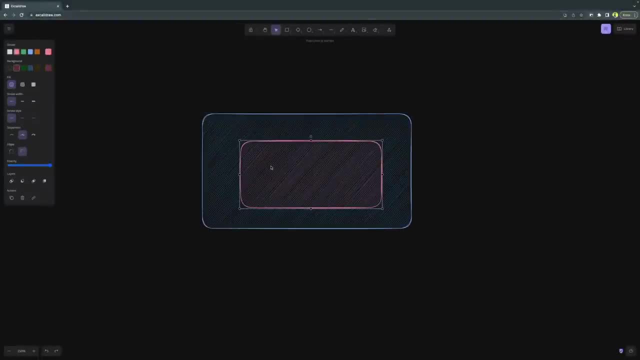 So there is a box inside that there is another box. consider this one as an Outer function and this one as an inner function. We have learned about the nested function already, right, So let's give them a name. For example, I'll give them, give the for this one as f1, as a function 1, or I'll give it as a name. 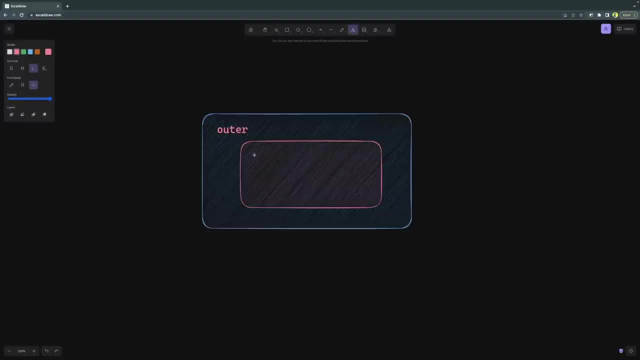 The outer to be very sure that they're out. This is outer and this one, of course, you know. now, you know, if I define a variable over here, say a, This variable is not accessible from outside. but if I Define a variable over here, say B- 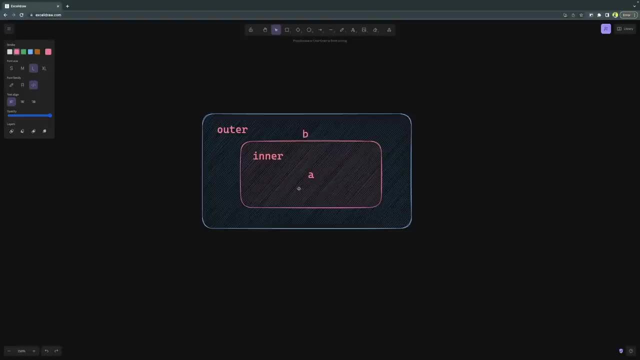 This variable is accessible from inside the inner function. So we have learned this in the nested function and the function scope very clearly. Okay, now What is closure? The nested function is a closure. This inner function is nothing but a closure. Okay, as simple as that. 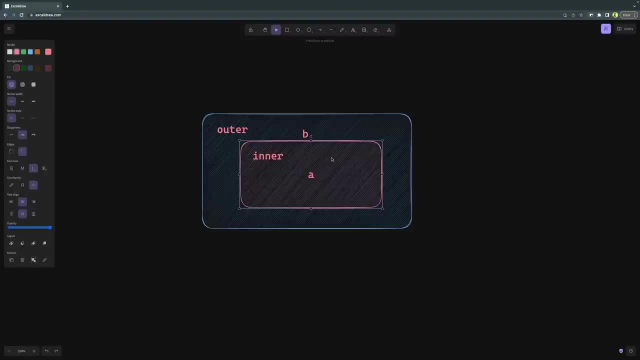 So if anybody asks you a definition of closure, you can tell this nested function is a closure. Now, if you go for a bookish, you know closure definition. for example, if you go to MDN and Try to look for what is closure, You will get a definition like a closure is a function that can have free variables. 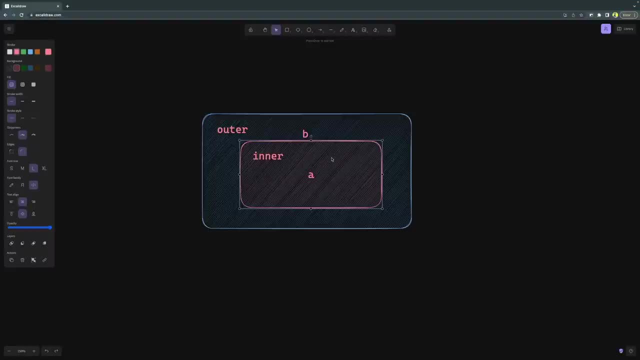 together with an environment that can run that variable. okay, which means it, the. the environment means nothing but this inner function, and the variable means every variable that is defined inside that inner function, And there is an ability through which you will be able to run things which is in this inner function. 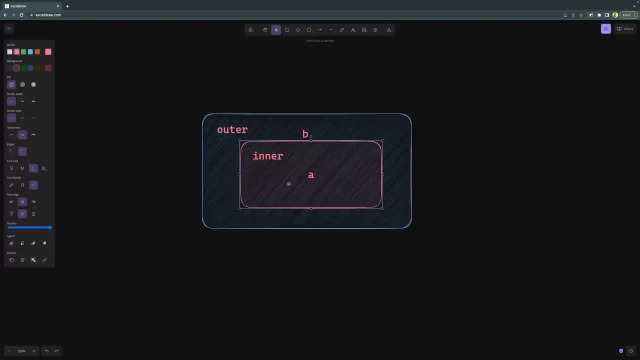 So this inner function is basically is a closure. Okay, it's, it's it. This is how we should be understanding closure. Now Let me summarize: the inner function can be accessed only from the statements in The outer function- correct, We'll see it in code also. and the inner function from a closure. It means the inner function can use. 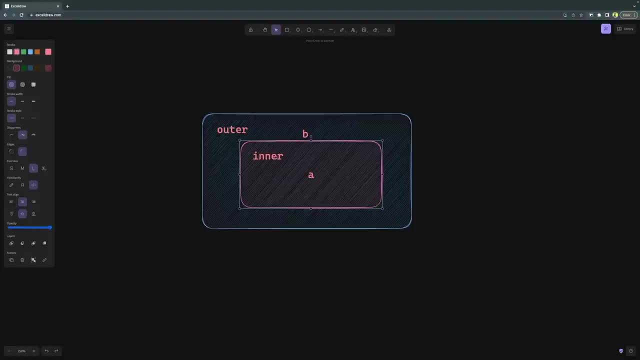 The variables, the arguments, everything from the outer function, while the outer function cannot Use the arguments and the variable from the inner function. You have seen, with this one, if we understand like, what is closure, the closure is nothing but the nested function, Because it provides an environment, you know, to the outer world. 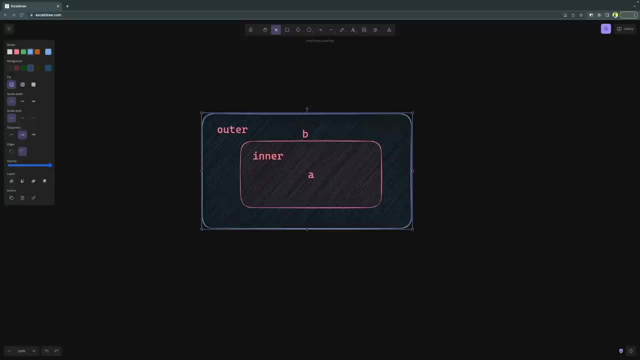 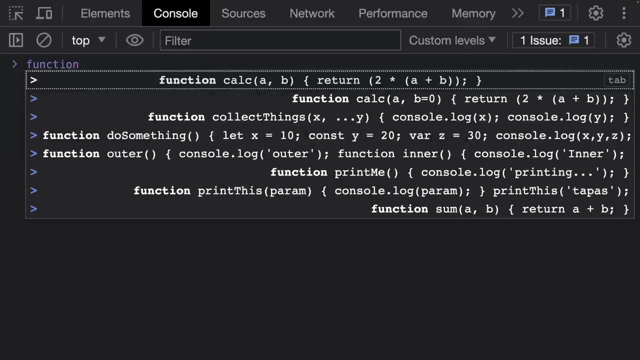 So this nested function can leave in a longer. the nested function can leave longer for execution. and So this next function does not provide an environment. It provides an environment. So it provides an environment which can give us an information and it can actually perform the All the required operations. right, So let's write a function. 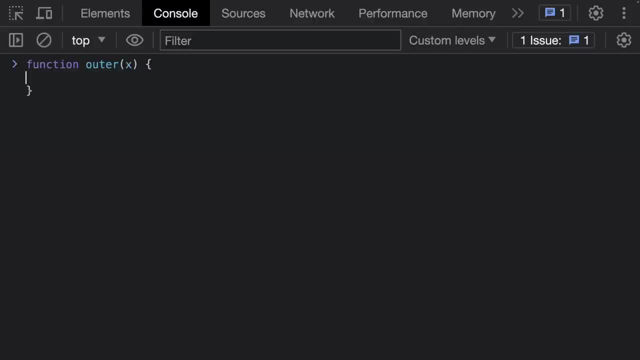 Will give the dim as outer and let's take a parameter of this one outer function and Then let's take another function, nested function, which is like inner. we will also take a parameter over here, and this is the beauty of it: the inner function can access the outer functions, variable and argument. 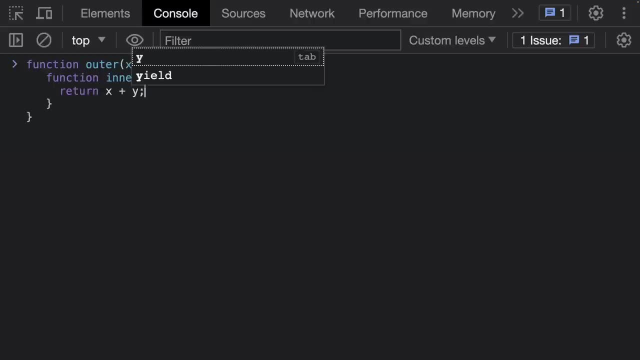 so i can do return x plus y. correct, inner function can access the outer functions argument or any variable that is declared inside outer function. so i can do return x plus y pretty well over here. okay, and then finally, what i can do, i can do return inner. okay, i am returning this. 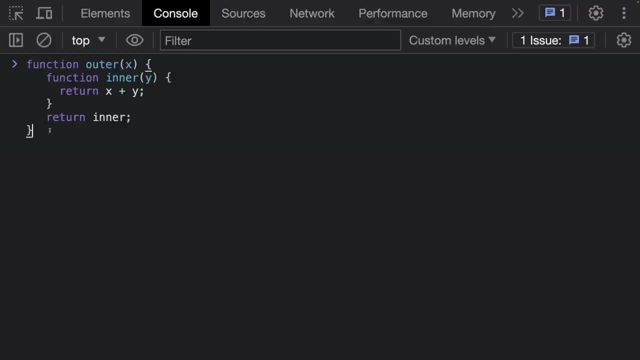 inner function as well. okay now, since the inner function, the inner function, is which one? this one forms the closure. this is what is closure. okay, now, what i can do? basically, i can call this outer function okay, and specify the argument and then leverage both the- the outer and inner- together. that's the advantage, okay, so let me see how can i do this. i will just 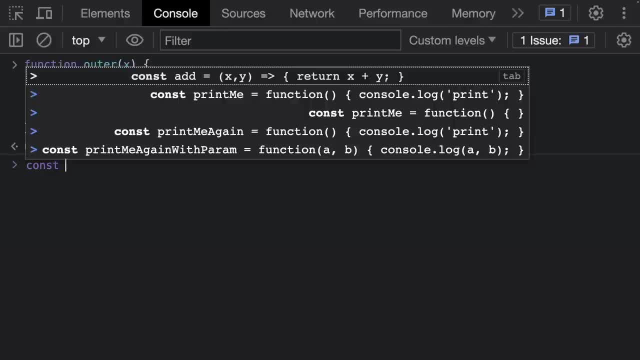 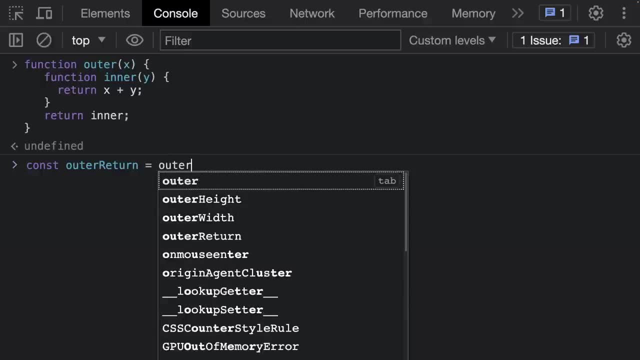 press enter now, first, what i can do: const: outer return equals to outer. let's give 10. what do you think will be returned over here? this is, this is this is the. this is the most interesting part. what will return? so, once we call this outer function, outer function return, nothing but. 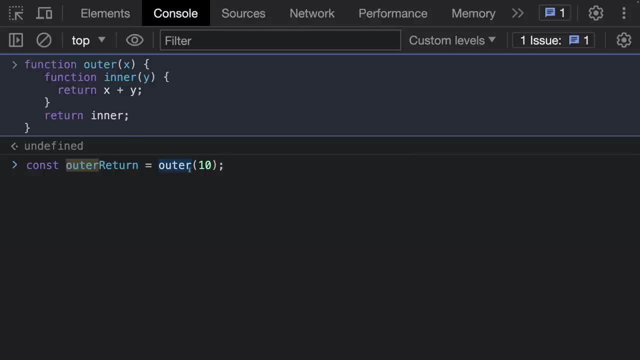 a function which is like an inner function. now, when the function execution is over, the call is over, that function is over, right, that function is nowhere in the picture. so if i end press and enter over here, outer is just over. it is nowhere in the picture, but the beauty of it, the beauty of it, is the argument i have passed to outer. 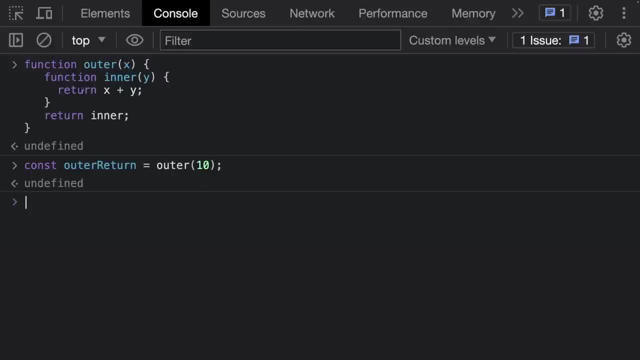 is still leaves where it still leaves inside inner, because this 10 was passed over here, this 10 is still used over here and it still leaves even after the outer execution because outer returns the inner. so inner is actually over here, outer return. so let me just, if i just do, outer return. 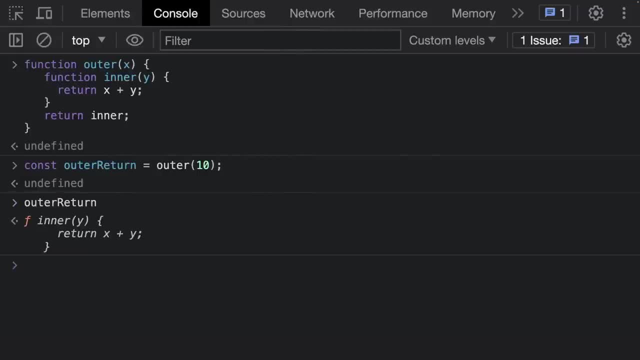 for you. if i just do this one and print this for you, what it returns is: returns inner y, return x plus y. this is return, this function, where x is nothing but this 10 that i have passed. so, though, the execution of outer is over, but the value that we have passed through outer still leaves within. 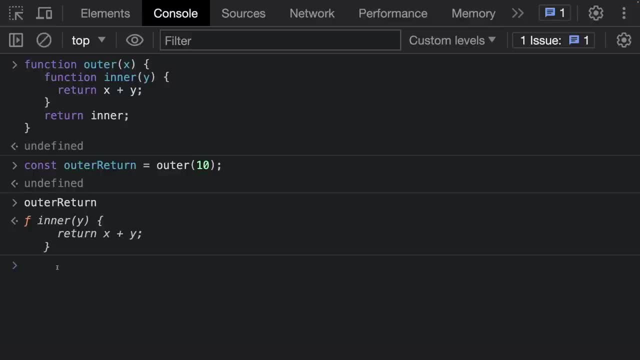 inner. so it means. it means if i just execute outer, outer return now, outer return now, with the parameter set 2, is going to give me the output of 12. why? because outer return is nothing but this inner function. inner function expects a parameter over here. the parameter that i have passed, as you know, pass the argument over here, but what it did it actually? 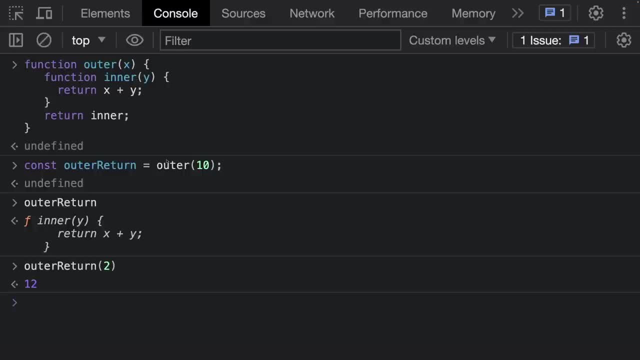 used this 2 with a variable that i have passed long back and the execution is over here, so that's why this is called closure. this is created a closure. closure is nothing but the variables and an environment that you can actually execute freely. what do you mean by freely? it means 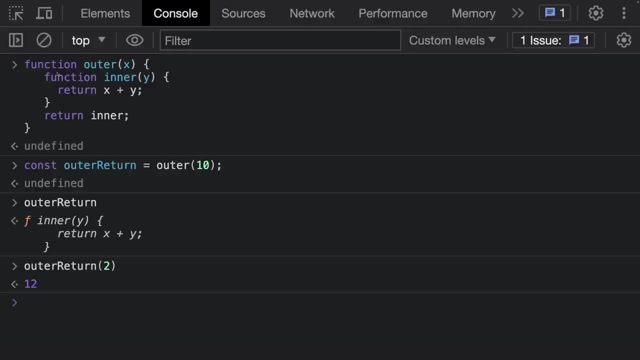 usually in functions, whenever the function execution is completely over, this is done. any variable, that is, that is actually created inside. that that's all gone is basically you are not going to get it anymore. but in this case, though, outer is not going to get it anymore, so that's. 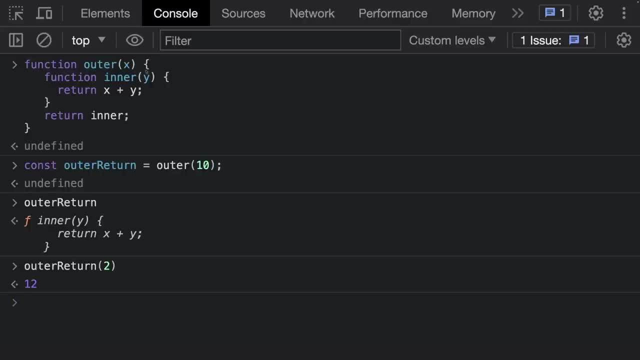 why it is executed long back. but the argument or the parameter we have passed through outer is still leaves within inner, because inner is a closure and i can actually utilize it, you know, at a later point of time. so this is what the concept of closure that you need to understand. 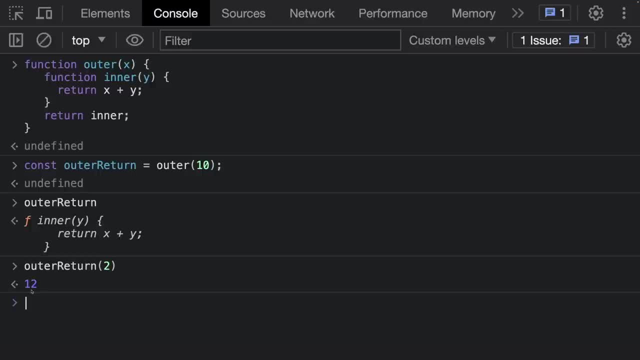 this is what you need to understand is like: uh, why closure is really a handy method, why closure is really useful. so you can use closure for various use cases. one of the use case that i have seen over here is like preserving the variable, so i have passed 10, though the function execution is. 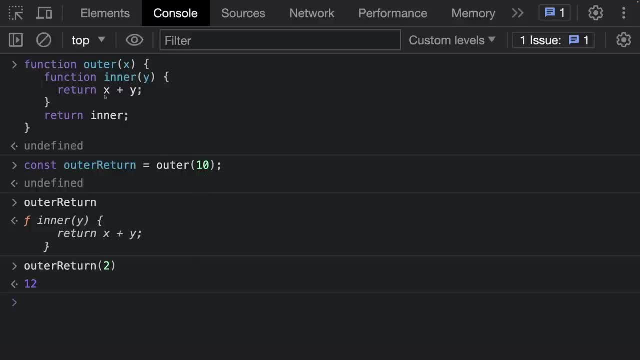 over, but still 10 is preserved over here and as it is preserved over here, it can be utilized with another value to compute something and return right. that's why the closure is useful in the video that i'll be creating, focusing on closure only there i'll be talking about much more real. 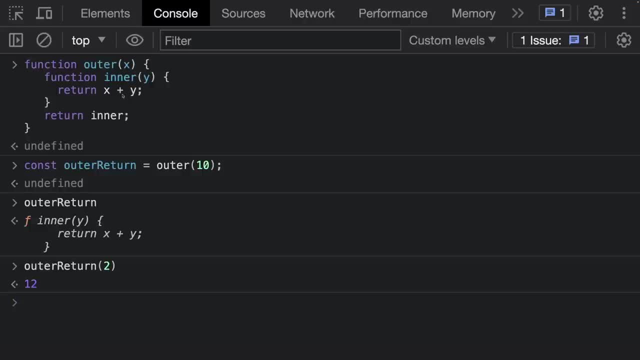 life examples and the use case that you can actually build with closure. so, as you understand closure fundamentally right now, start with the first one and then you will be able to build a second one and then you will start practicing, start creating this kind of a small example. 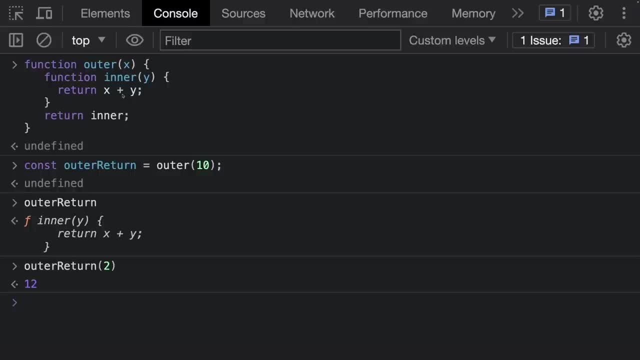 where you have a outer function, inner function, outer inner, both take some argument. you return the inner function from the outer function and see, after outer execution gets over, how the value that you have passed through outer you can still used inside inner at a later point of time. so this kind of thing, the example that you are seeing over here, try to find out this example. 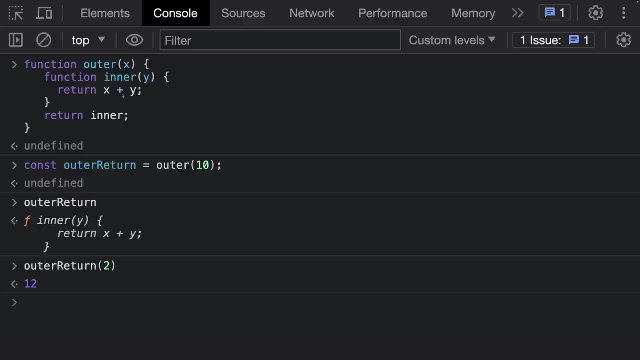 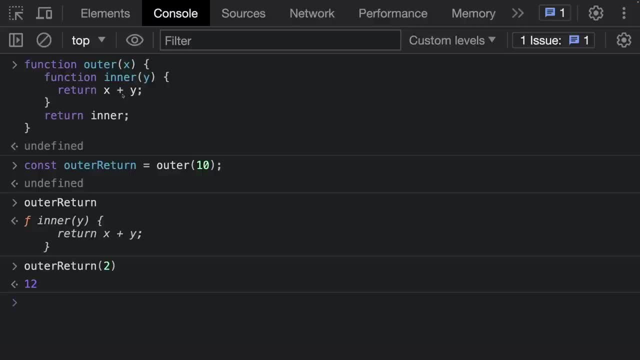 i hope this clarify your concept. now, just to recap it once, the closure understanding is depending on your understanding of nested function plus function scope. we know by nested function that a function can define one more function within it. we know why the function scope is like the outer. 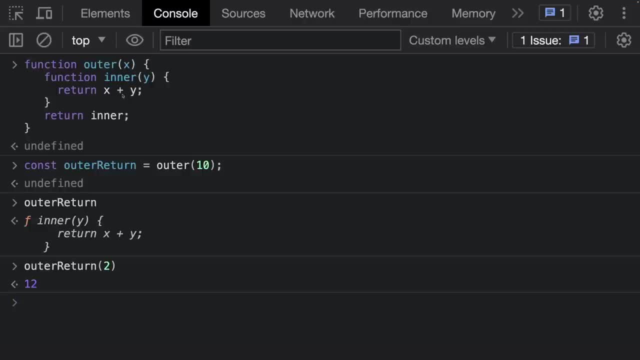 function cannot access any variable inside the inner function. however, inner function can access any variable and the argument of the outer function can access any variable and the argument of the outer function. this ability gives us a very powerful feature called closure, through which, even if the outer function execution is over, but we can persist certain values which was passed to the outer 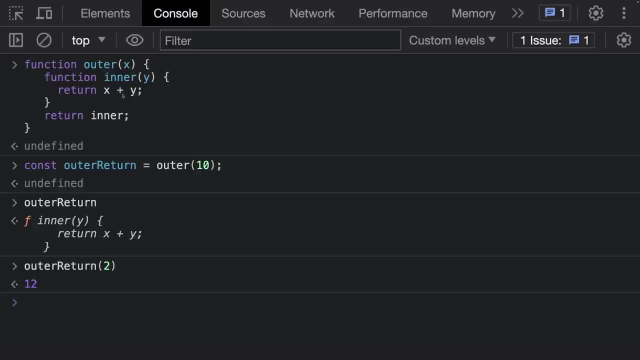 function within inner function and compute it at a later point of time. that becomes a powerful feature itself, a powerful design pattern itself in javascript, which is called closure. i hope this is clear to you. now we learn about the function of the outer function and the function of the inner function. 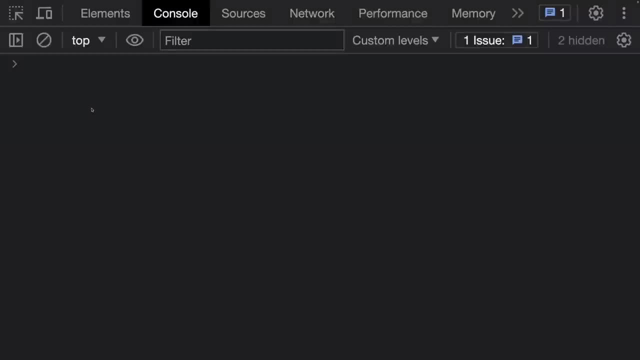 now we learn about callback functions. what is callback? okay, so everything is in the name itself: callback. it means call it back some point of time. but let's understand with some example now. in javascript, function is a first class citizen. what do you? what do you mean by that? 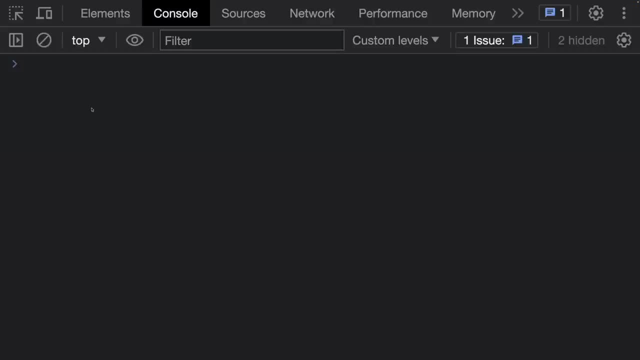 it means that we can create a function. we have seen function definition. we can assign a function. we have seen like, when you do const, x equals to function and then, basically, we can assign this function to a variable. we can assign a function, we can return, we can define a function within another function. we have seen this from the 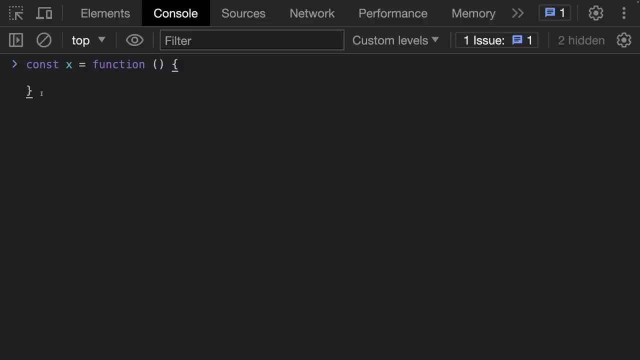 nested function. now the next thing that we are going to see is like we can pass function as a parameter to another function. okay, that is where the callback function comes into picture, and we'll see what these use cases are. okay, first let's define a function called foo. 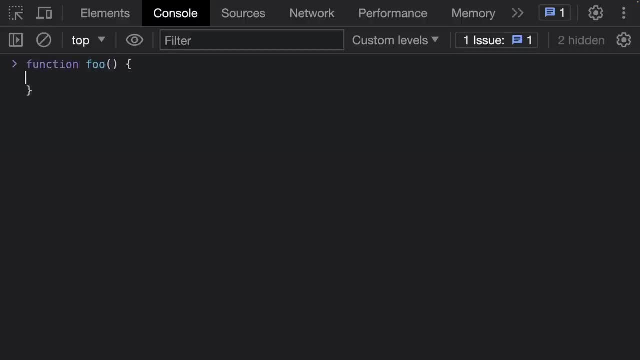 and this is the foo function. what is this foo function doing over here? let's assume that foo function cat can take another function as a parameter. let's pass another function function as a parameter called boo. or let's call bar, because that's foo, bar, bus are the things that we usually use. these names, for example. now, as this function takes an. 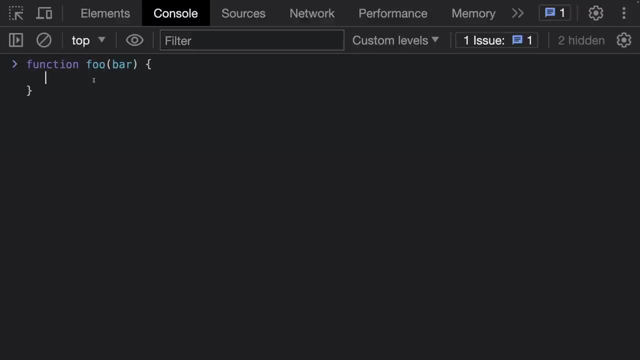 you know, argument, which is nothing but another function. so it means i can capture it as a bar parameter and assume that this bar is nothing but another function. so it means that inside this i should be able to execute this function very simple. if it was a string, i could have printed the string or concatenated. 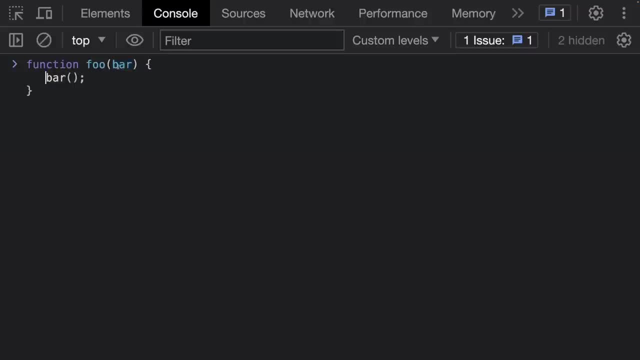 with something else, or done something with the screen. if it is a number, i would have done something with the number. if it is a function, i'll simply execute this function now. to execute this function, we know that we have to give this parenthesis to call this function, and then we 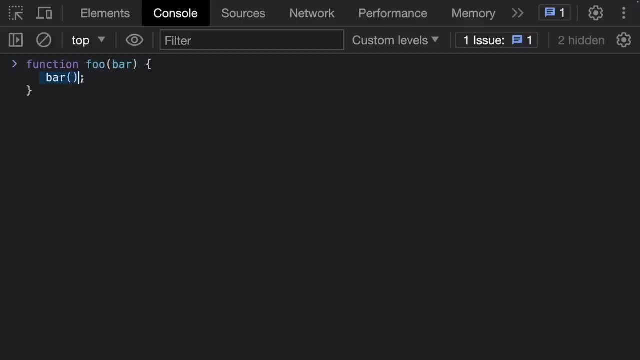 call this function or execute this function. this particular function is called a callback. okay, this particular function is called a callback, but why? we'll come to that. but first i want to execute this. how do we execute this one? i have defined it. now, if i have to execute, 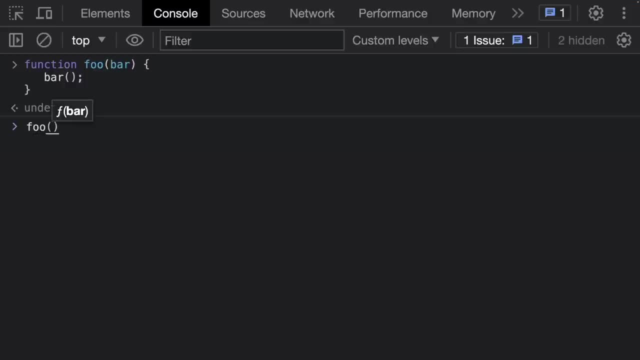 this: i know that foo takes a function, so i can actually pass a function to it. okay, and let's do something like this. so what i did? foo takes a function. of course we told foo takes a function, bar is a function and we execute it inside that. this means that i can pass a function as an 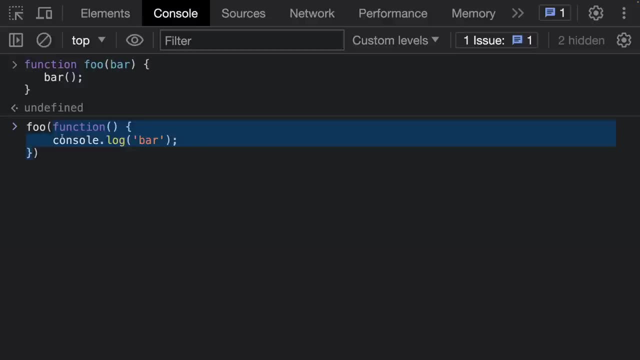 argument to foo. so i have passed a function. do you guys realize one thing over here? i have created a function which doesn't have a name, so this function is called anonymous function. the function that doesn't have a name is called anonymous function because it doesn't have a 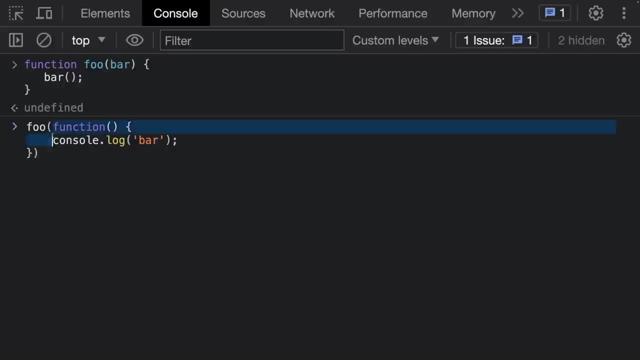 name and as i will be using this function instantly over here, i didn't bother about creating it again. okay, so if i just execute this one, this function get passed over here and then it gets executed in this line. once it get executed in this line, this consolelog get executed and it. 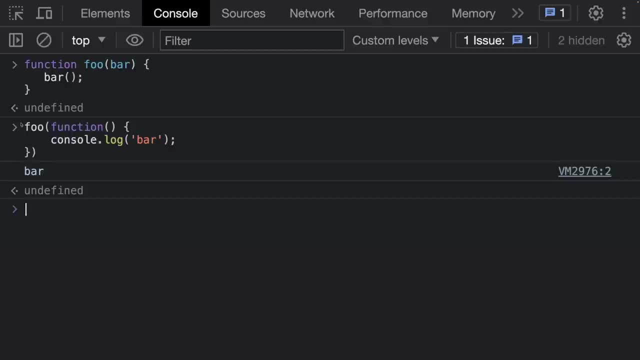 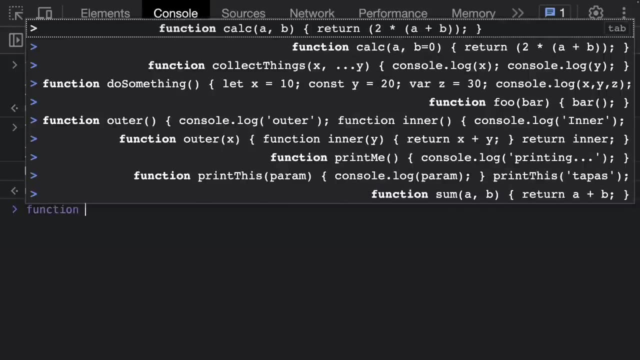 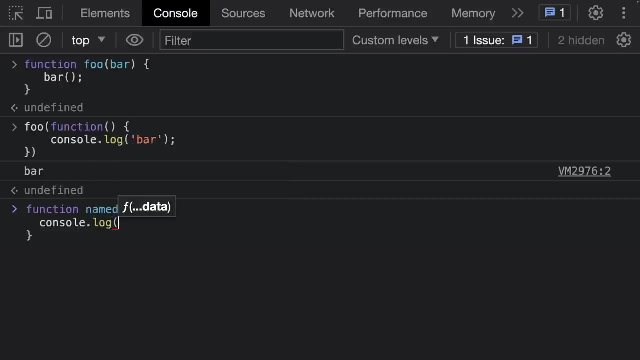 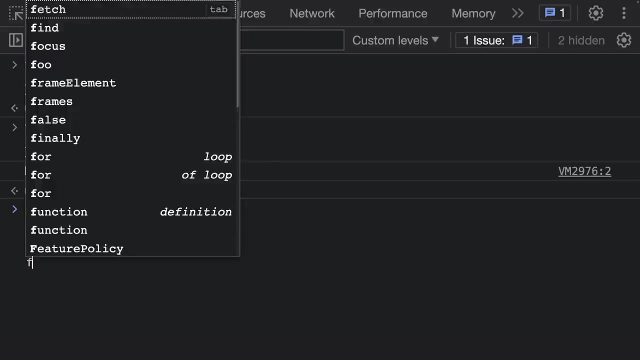 prints bar- same thing. what i can do instead of doing this line, for you to understand, is better. i can create a function with a name, for example, function named, and instead of that i can actually say consolelog of bar- again same thing like the previous function. instead of passing it directly, now i can do foo of named. right is exactly the. 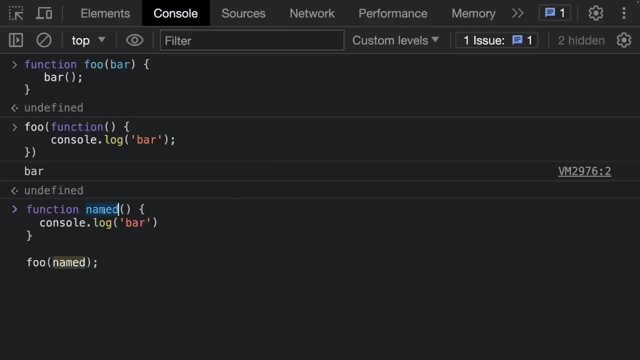 same thing that whatever. instead of again declaring the function with the name function and then passing the function over here, i just pass the function directly over there. that's the only difference, but output is same. okay, so now you know. a function can take a function as an argument and i can actually. 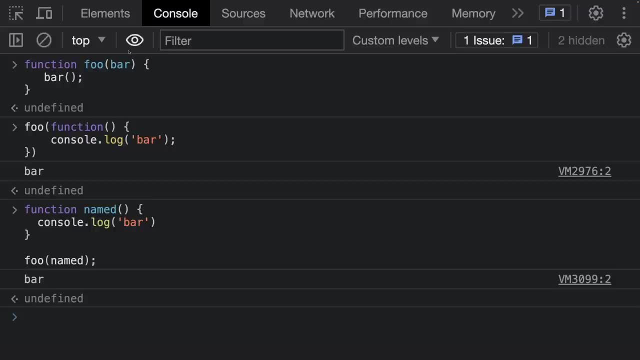 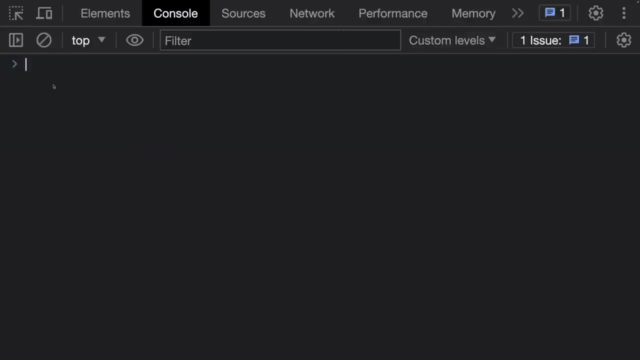 do that and the function which is passed as a parameter- and i'm using it, you know, inside it at a later point of time- is called callback function. but why it's called callback function? that's the thing. let's go from the beginning again to understand why it's called a callback. 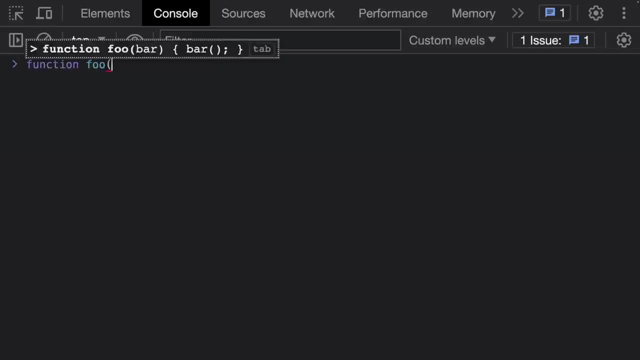 function. so again we'll be defining function foo. take another function, bar, and let's say i have some condition. condition is if its night. consider that its night is a boolean variable. it can be true or false. in that case you call bar, okay, usually under at the night only, like you know, bars. 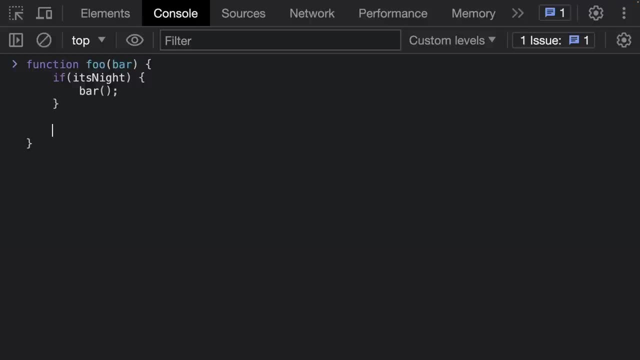 will be like flourishing everywhere. or let's say, another condition is there if is drinks over a shake on line, in this case only okay, spelling mistake: check online. in this case itself, you call bar. so we have two conditions where we want to call this particular function call bar. the one condition. 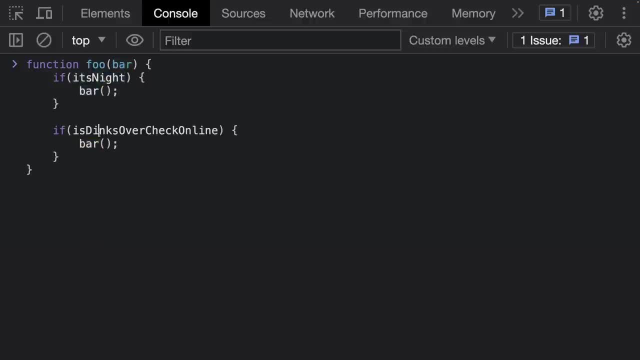 is: if it is night, then call bar function or maybe do an online call, a network call, to check whether the drinks is over. then only you call bar. so it means that calling back bar is based on certain kind of conditions that is happening within this function. this is a case where you actually want. 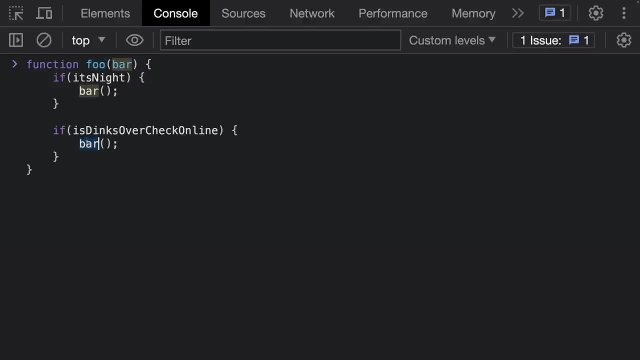 to call this function as a call back function. you are calling it back based on certain conditions, based on certain things. it is so, so, amazingly powerful because you can pass any function to another function and call this past function based on any condition at a later point of time. that's why it is called call back now, if you want. 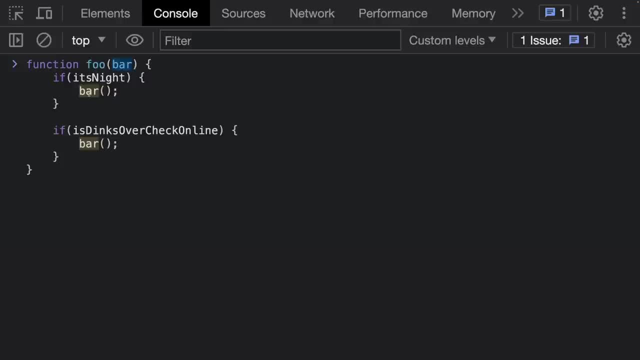 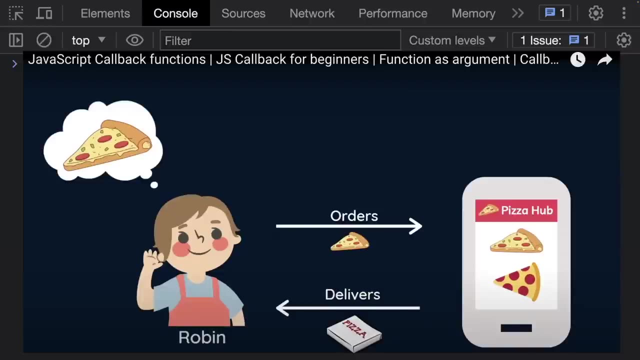 to understand this concept with much deeper example. i have created an example with the pizza hub, or the pizza hub and a little boy story. it's like a storytelling, so that anybody can understand. that video is already out there. go ahead and check out that video. the link of that video is in the. 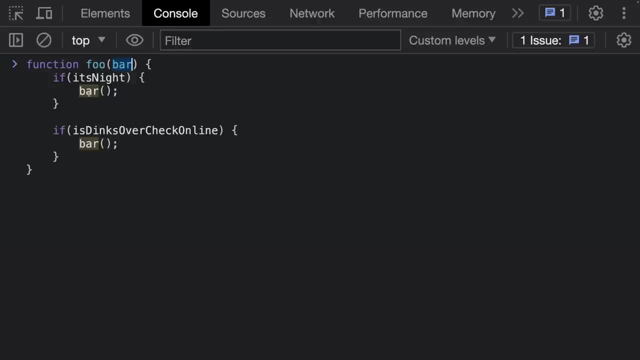 description of this video. you can check out and find out, like you know, how, in a real life application, you can use this function to call back bar. so that's why it is called call back. you know effortlessly. so i hope the callback functions is clear to you now. 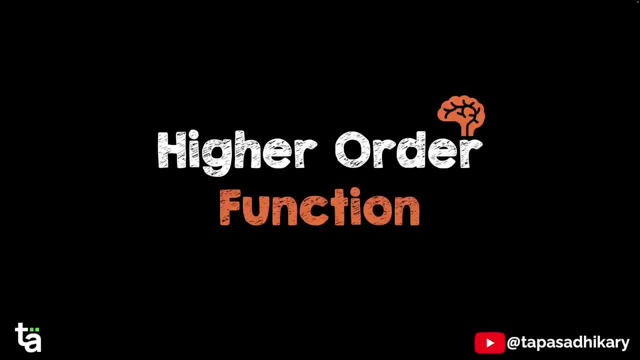 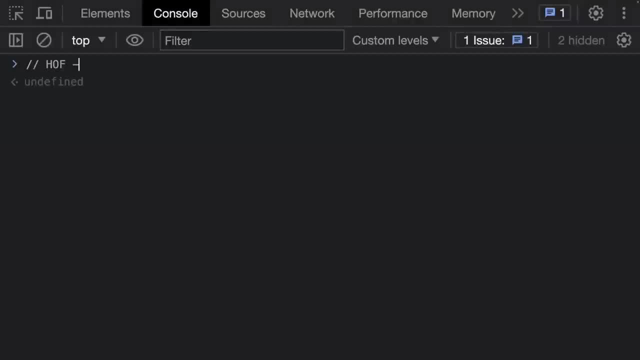 now we learn about higher order function. higher order function or hof. okay, what is higher order function? a higher order function, by definition, is a regular function. it's a normal function that takes one or more function as an argument and or returns a function. that is a regular function. that is a normal function. that is a regular function. 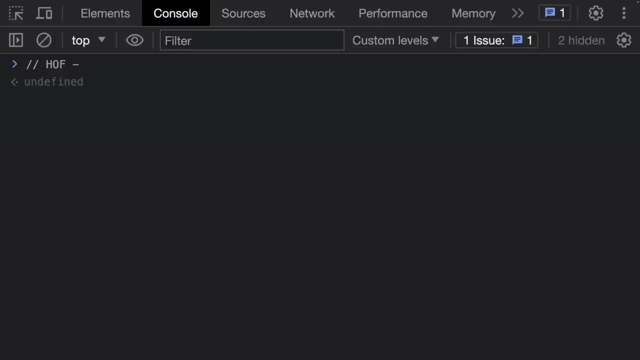 returns a function as a value from it. okay, let's write it down. it's a bit complex in that way. so one condition is like it takes one or more functions as argument. okay, this is the first thing, and then the second thing: it may return a function. okay, so not necessarily. 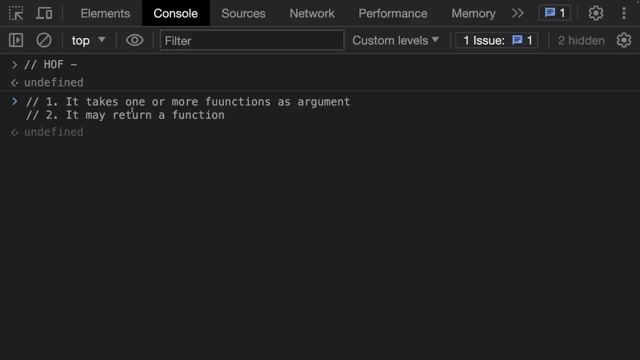 all the conditions has to be made for a higher order function. if any of the condition meets, it's actually a higher order function. now, we just now spoke about a callback function. right, what is told about callback function? a callback function is a function which takes a function as an argument. 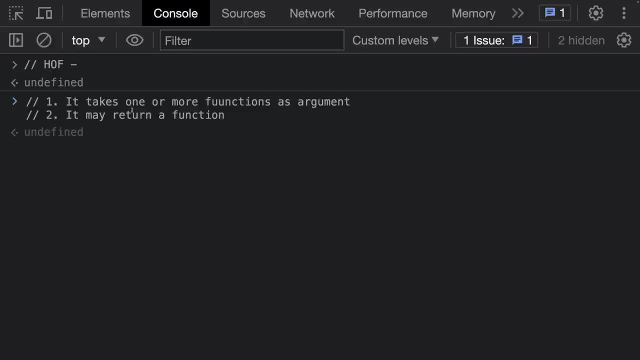 based on certain conditions or something. whatever the function we are passing as an argument, it is going to invoke that function inside. now, in the first case of the h of h of bar, you can see h of higher order function is about taking one or more function as an argument. so it means 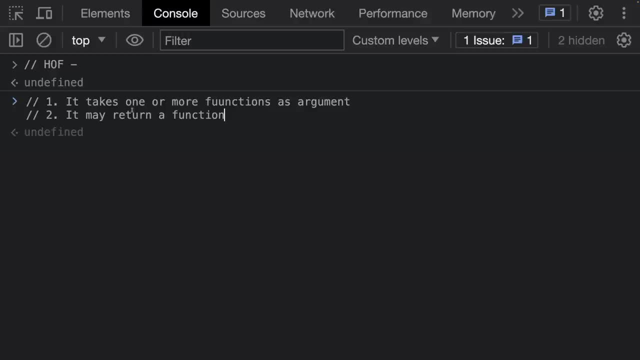 there is a relationship between a higher order function and a callback function and that is where sometime in interviews interviewers put some tricky question: is h of and callback are same? no, h of and callback are not exactly same, because for callback functions it is not mandatory for 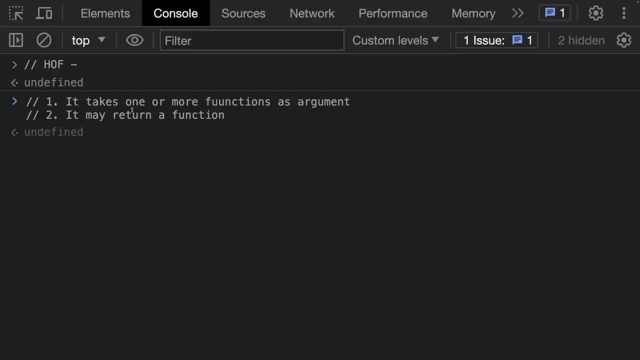 the main function to return any function. it can accept a function as a argument, do something with it, but it is not necessary that it has to return a function, whereas in higher order function, if the function return another function, it calls a higher order function. in that case also it calls higher order function. 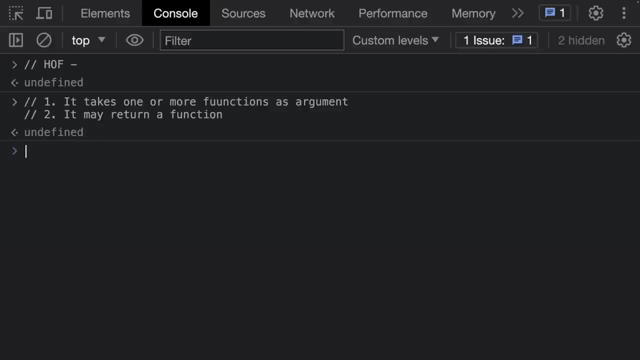 okay. so it means that if i am just taking like a function, okay, let's take a function, let's give it a name call get capture and let's take a parameter called camera. okay. now, if i am doing like this, this is a higher order function. why? because camera is a function and i'm executing this. 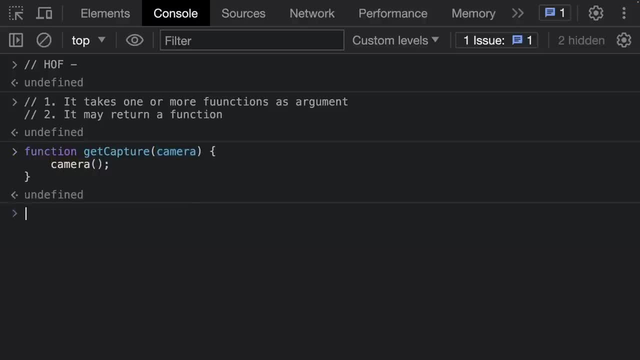 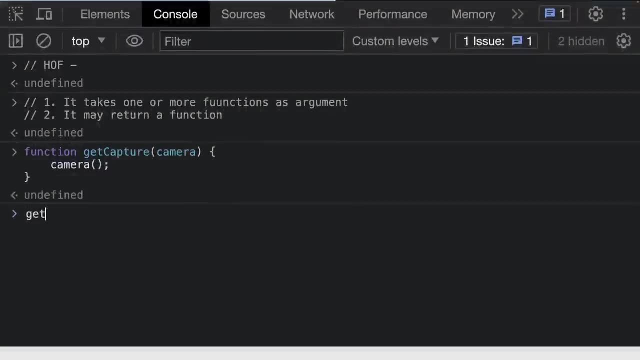 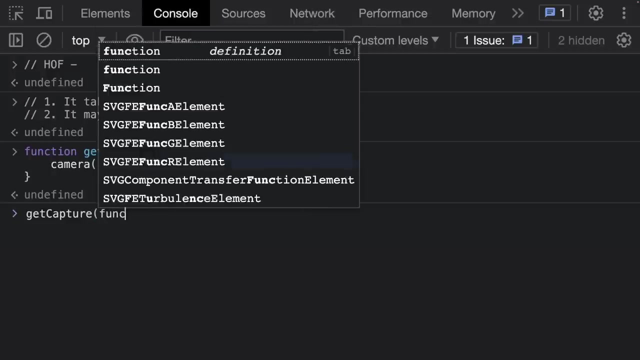 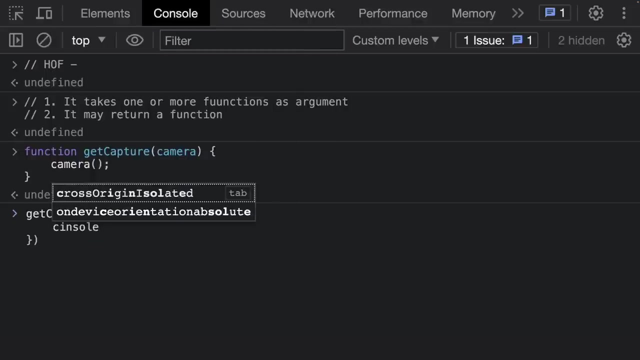 one over here so i can actually call get capture over here. i can call sorry about that. i can call get capture over here and pass a function to it. I can say function. okay, do a console consolelog say canon, okay, so it executes. This is what we have seen when we understood a callback. 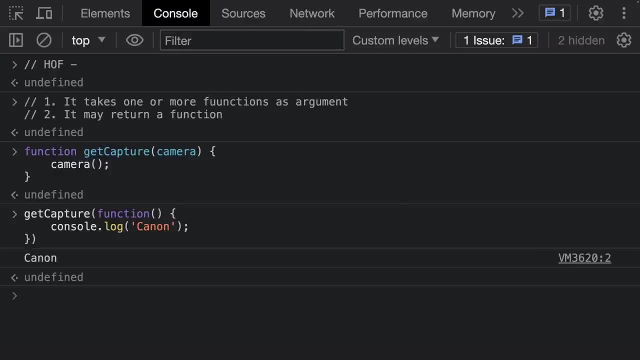 functions methodology. Now we can do the other other part also, like a function returning another function, which is also called a higher-order function. So how it will be, we can actually do like function return the Fn and it can return a function which say consolelog of returning something we are printing over here to 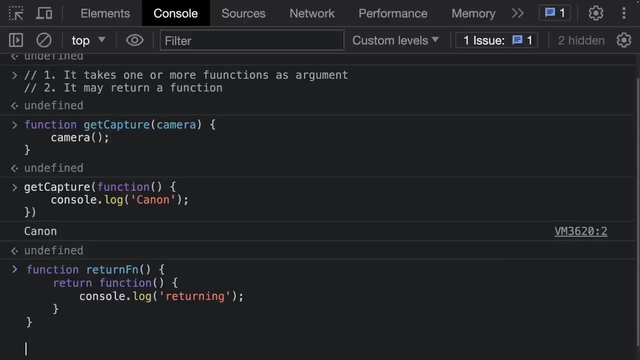 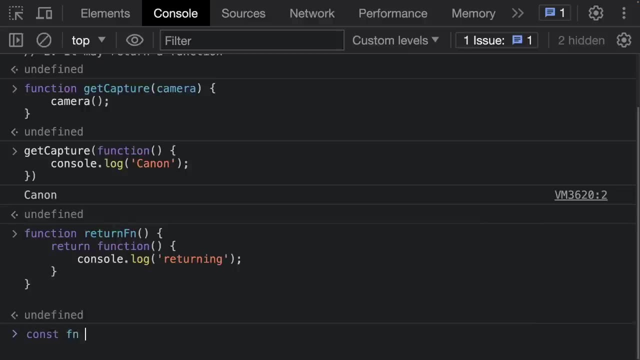 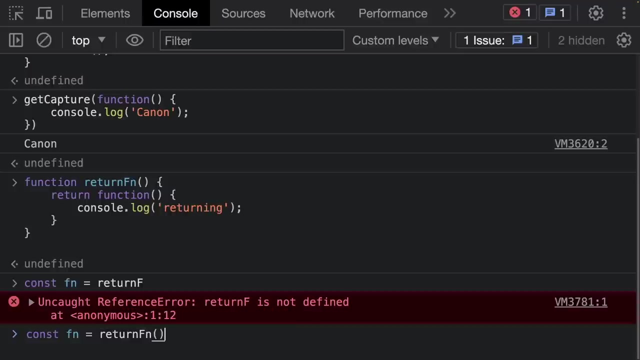 prove that it works. Now how am I going to execute this? multiple ways to execute it. for example, const say Fn equals to. I can do return Fn to return Fn. when I do return Fn, what it does? it return a function right now. so if I do this, 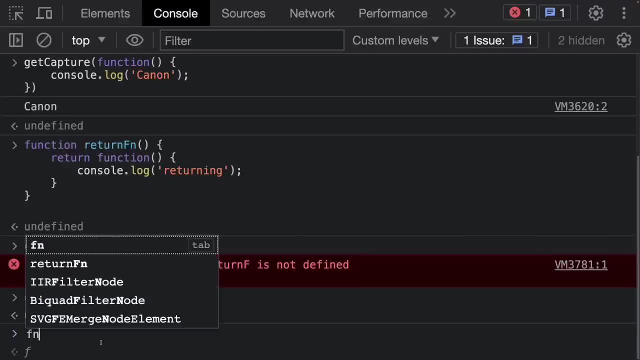 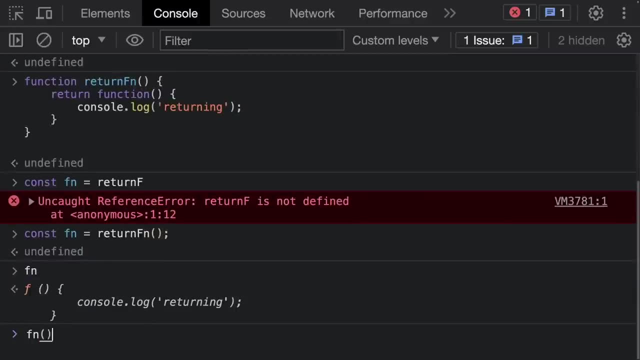 so Fn is now nothing but a function. if you see that the moment I'm typing Fn it is giving F. if I just do a print out over here, it is running a function to execute this one. it means I need the parenthesis. okay, so it will execute this. 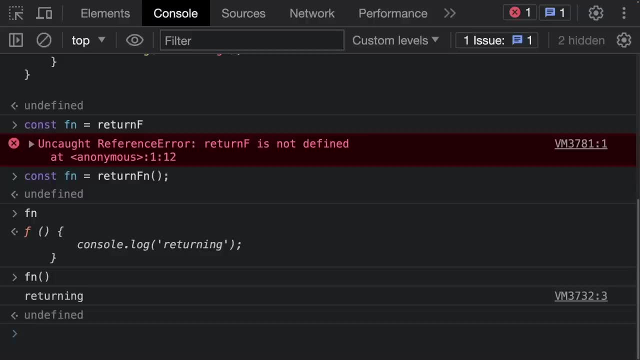 one. so this is one way that I actually can execute this thing. so I hope this is quite clear. now, do you? if you are working on JavaScript for some time, you are already using some of the higher-order function. you know already, and this higher order function is extremely, extremely useful for you know your. 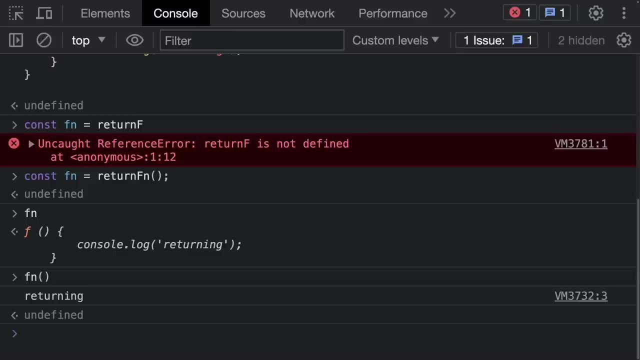 code, reliability, predictability, aspects of it. you are already using some of those things called array functions, like map, filter, reduce. find all this method that you have right on. the arrays are all higher-order functions because they are also. you write a code like you know one. if I take like 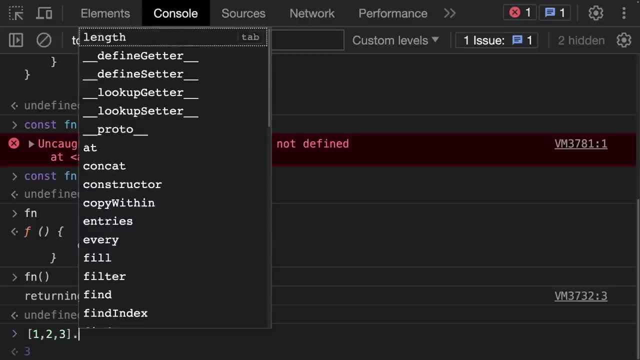 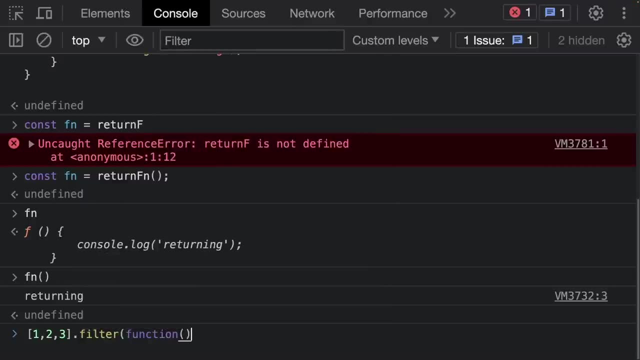 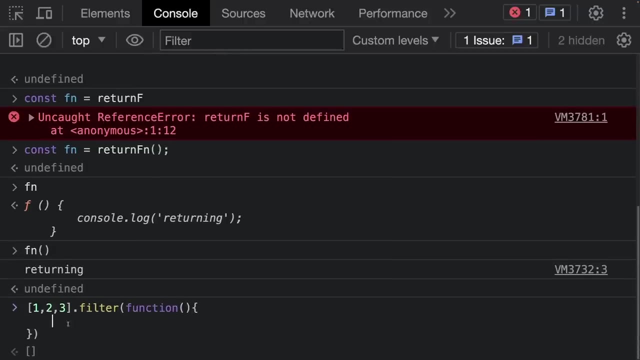 1 comma, 2, comma 3, and on this array you do something like filter and in here you pass a function right, your filter condition you pass over here. if you are using array already, you will know that and this is where you actually put your condition like based on which condition you. 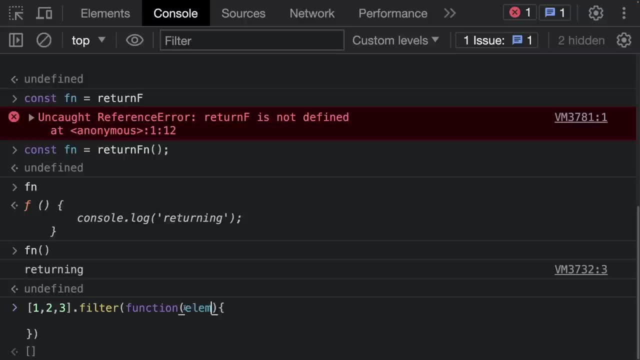 want to filter this one out. right, you get this like element and if the element greater than 2, greater than 3, you know you actually write conditions like that and based on that, you filter the things out. so this is an example of a higher order function like how, why exactly it's? 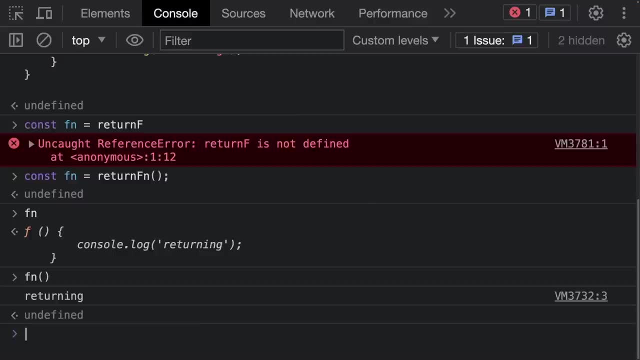 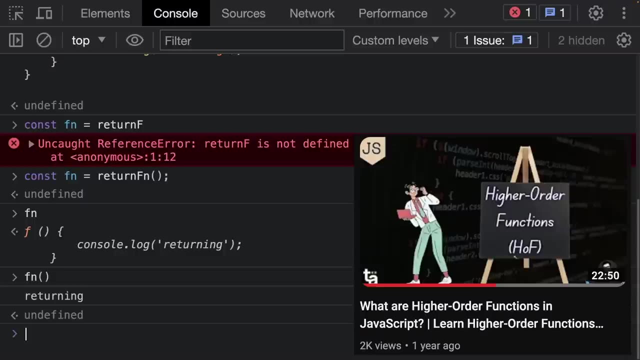 called higher order function and where you use the higher order. now again, if you want to get a very, very deep look of higher order function- as it is crash course, we are not getting into too much deep, but you want to get a very good deep of higher order function. i have already created a video. 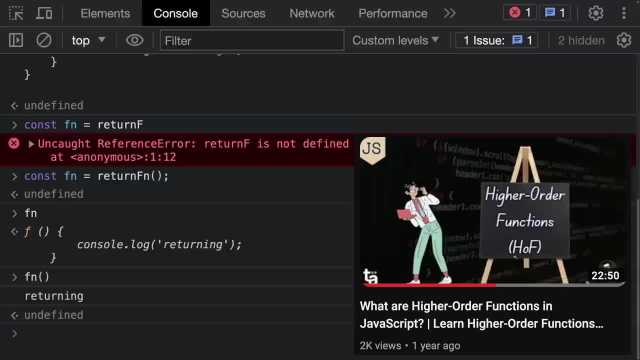 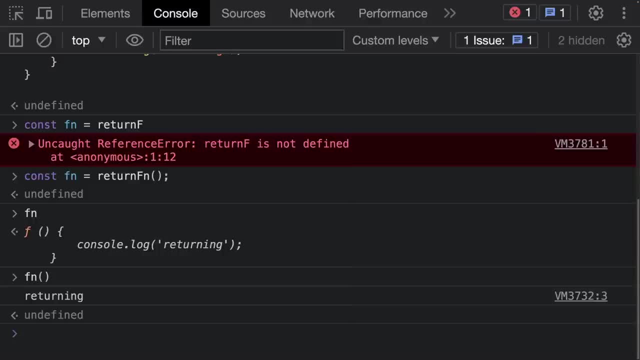 for it. please take a look at it. i'm sure that you will enjoy learning higher order function and try to understand what are the different use cases apart from built-in javascript functions. whenever you are coding, in what cases you will be using higher order functions? please take a look. 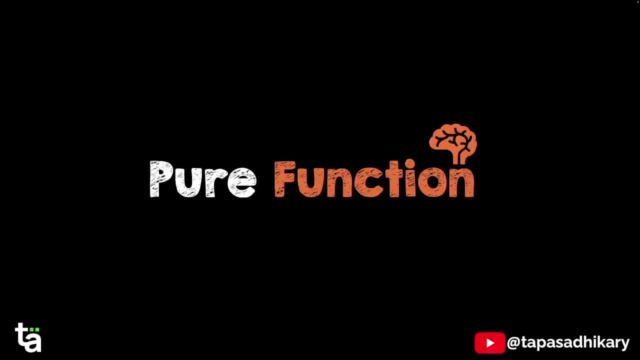 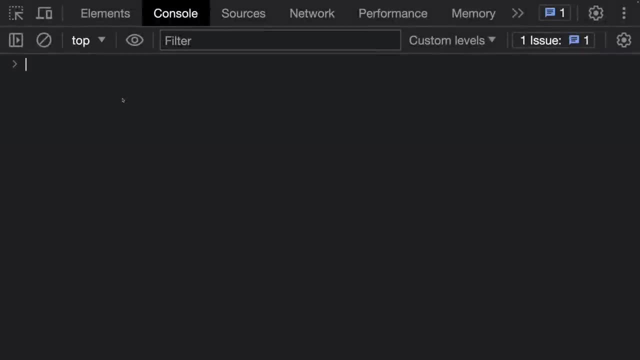 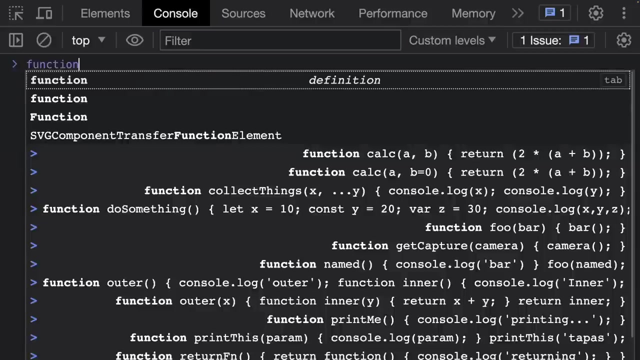 let's see what a pure function is in javascript. when you are dealing with function, you deal with lot of pure functions. you also deal with lot of impure function. by definition, a pure function is a function that produces the same output for the same input. same output for the same input. okay, so function. 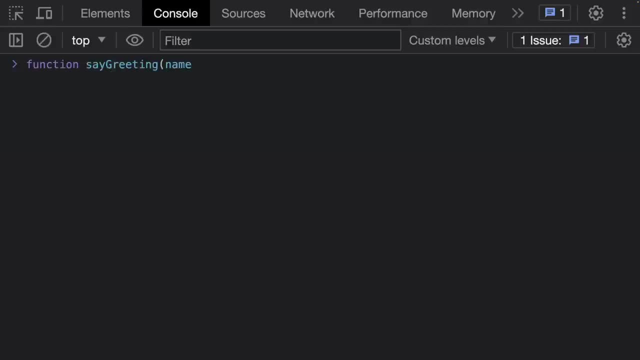 say greeting, input is name and what is going to do is going to return a greeting message. okay, so return hello, and you know. so this kind of greeting message is going to return. so fair enough. so if i call, say greeting and pass my name, is going to return hello, tapas. so for same input is going to return same output. 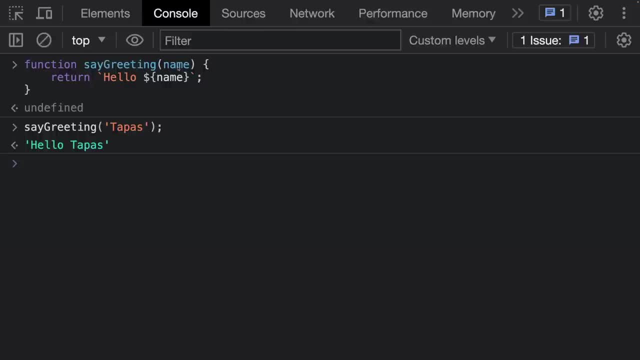 if i, as many times i am going to input tapas, that many times it is going to return hello tapas. if i do hello youtube, it is going to return hello youtube. as many times i am going to input youtube, that many times is going to output hello youtube. pure function. this is pure function, pure function. 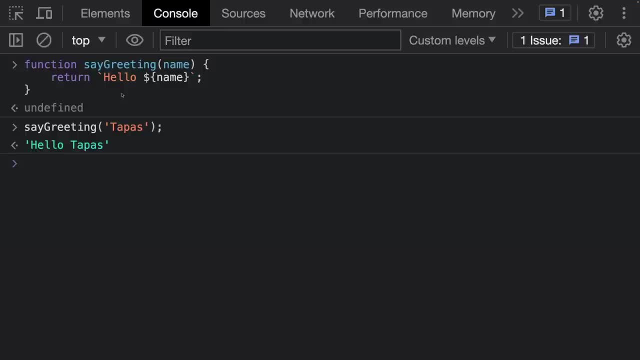 urd computer, that means pequeño npc player. it means, to these size of the Working hour, critical content predictability. it means that if the input is same, output will be always same. so this is very, very predictable. what is, in pure function, just the opposite of that it means. 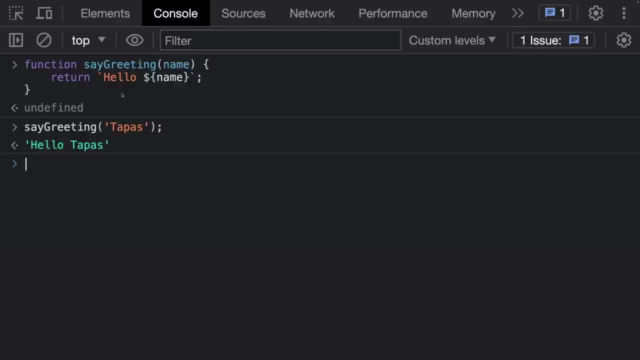 that for the same input is not going to create the same output. okay, so same function if i just do a little bit different way. so, for example, let me create a grabs in pitt, 맞는 way to get some very short wait for next with you, which i was just going to Scriptures, right, exactly. 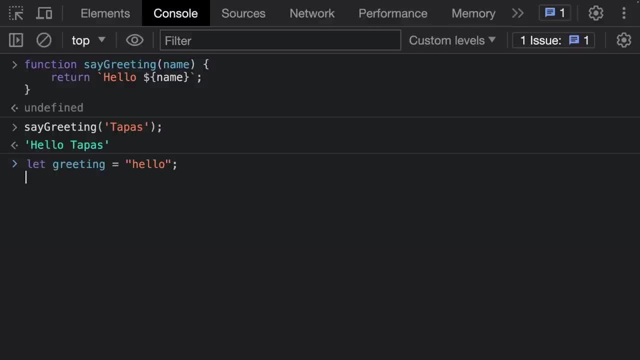 what i did yet. no, initialized with hello, okay, now i have to make images of that. and when you also has to report, what do you actually do? go to Col Bill and check out that, OK, so i would never do that now if i did that, and here im going to go here and describe to you what you can think about is a very similar to that meetings. 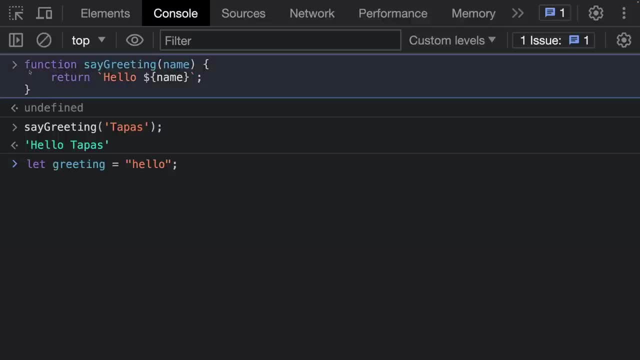 Now I have a function like function. you know this guy. I'll just copy this so that I can utilize it, but I'll change a little bit what I'll be changing. instead of this, hello, hard coding, hello, now I am taking this greeting from here. okay, all right. so if I now say greeting tapas, it will give hello tapas. fair enough. 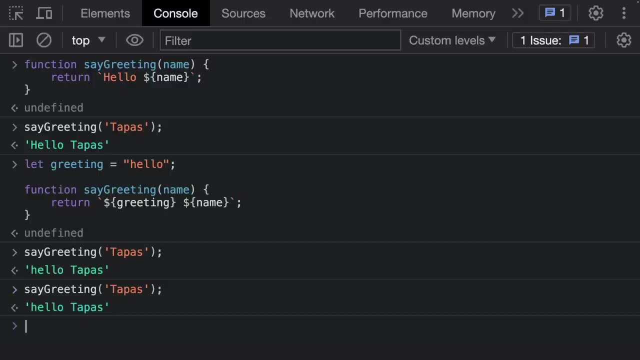 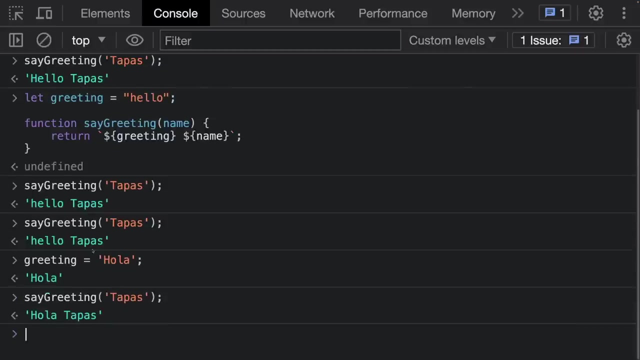 if I give tapas again, it will give hello tapas. fair enough, but if I change this greeting variable value to from hello to hola, hello to hola, and then I do it again for the same input tapas, the output become hola tapas. so from hello, hello tapas it become hola tapas. so this means: 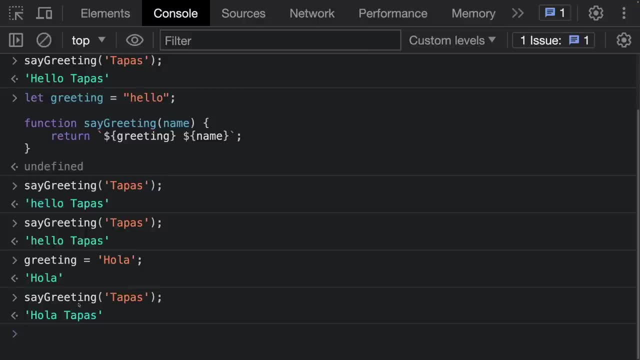 it means say greeting is not producing the same output for the same input right now because it is depending on something and there's something is called side effect. what is the side effect? the side effect is nothing but a variable which is outside of the scope of say greeting function, and say greeting cannot control this particular variable any. 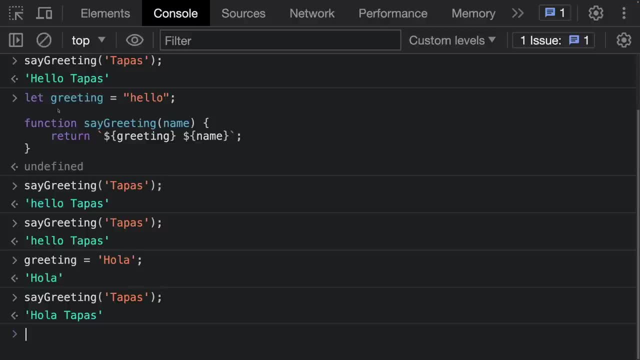 anyone can change, which can create a side effect such that this particular function is no more a pure function. it is no more returning the same output for the same input. so this is the difference between a pure versus impure function. can you write all the functions, as pure function in your application may not be, you may not be able to write you know all. 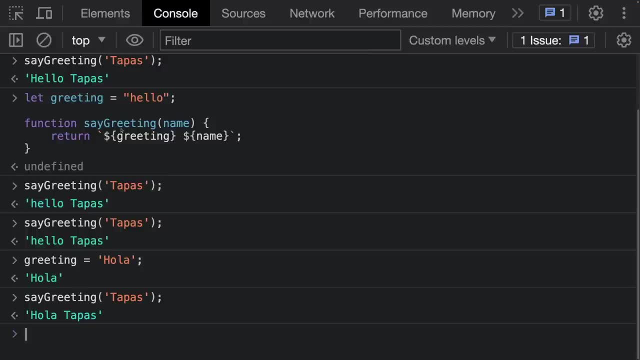 the functions as a pure functions, because there will be side effects. you need things like that. you have to make network call, you have to probably write something on the console log. everything is side effect, but as much as possible. if you can make certain things as pure, you have more, more. 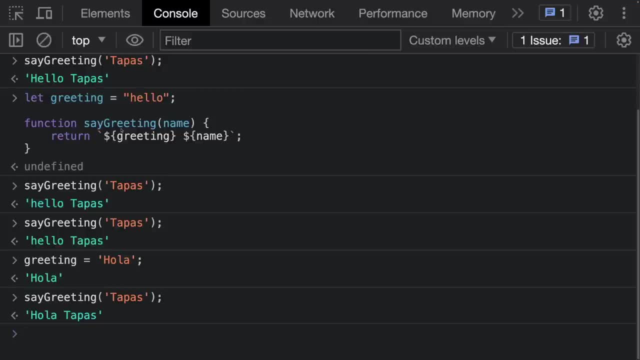 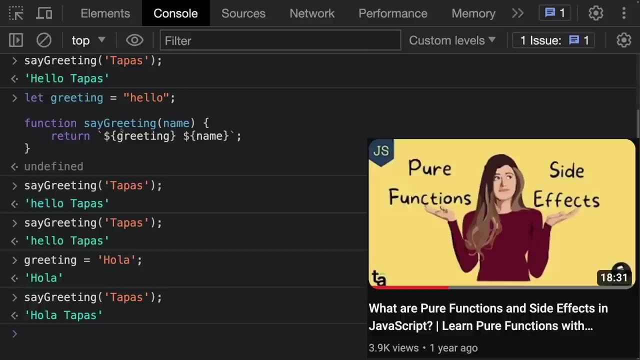 predictability for those cases. so look out for these things again. if you want to get deeper to pure function, you want to learn, like the real life use case of pure function, where exactly we use, where can we make use of it. i have created an extensive video for pure function. take a look at it. 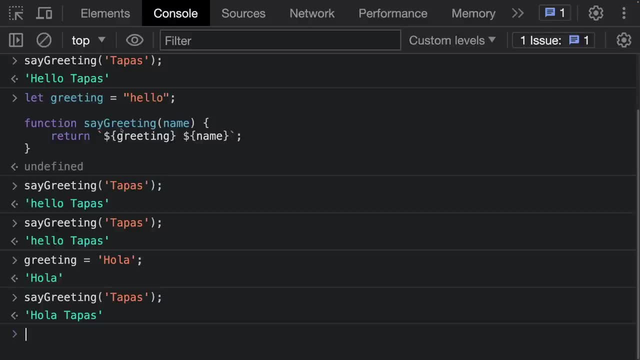 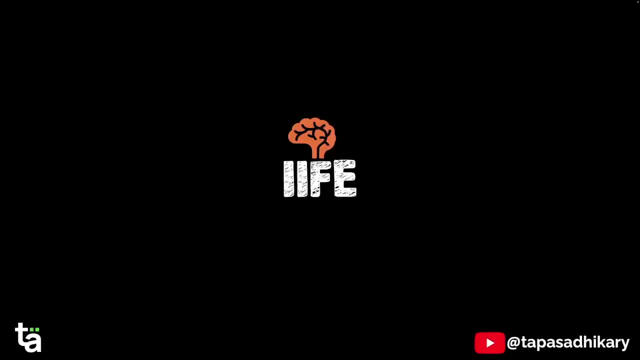 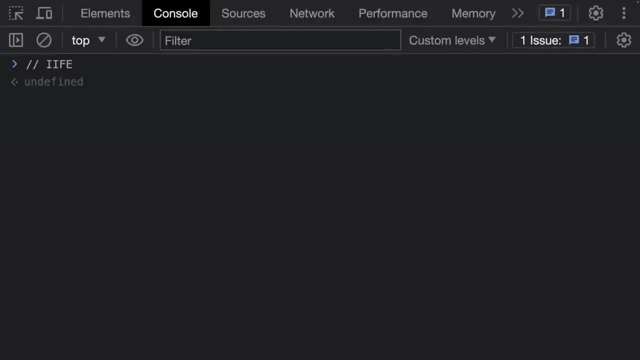 so that you can learn and practice it much more. all right, so i hope now you got the basic, fundamental understanding of a pure and impure function. all right, friends, so let's learn iiafe. what is iiafe? it's an abbreviation of the term immediately invoked function. expressions i for immediately, then i for. 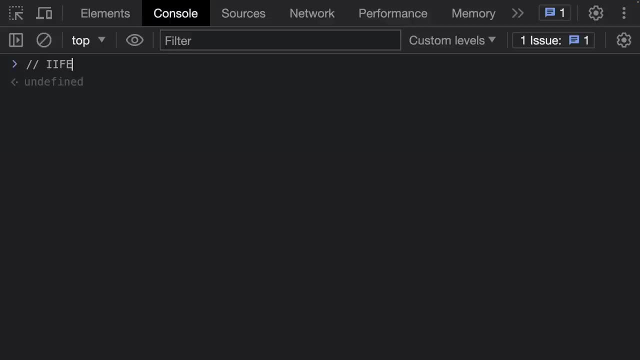 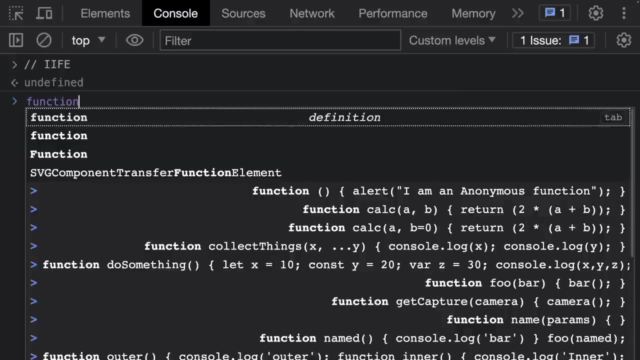 invoked, then f for function, e for expression, immediately invoked function expression. what does it mean? it means it's a function expression. that's where the code inside the function gets executed immediately after it's been defined. now let's take a function, for example function x. this is the function right which is having a name x. 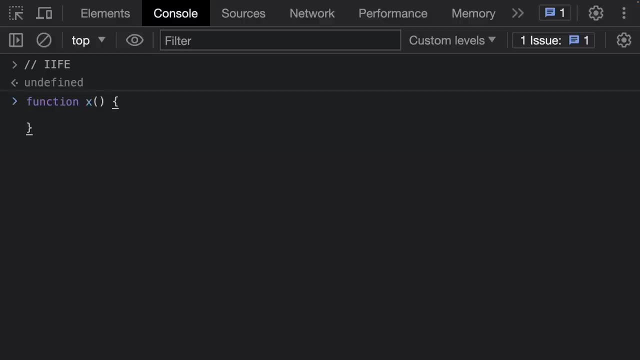 now, if i have to execute this function at a later point of time, whenever i want in my code, what i'll do? i'll just use this name with the parenthesis and execute this function. okay, that's great. now the only reason why this name exists- the x for this function- is because i can use this name to execute this. 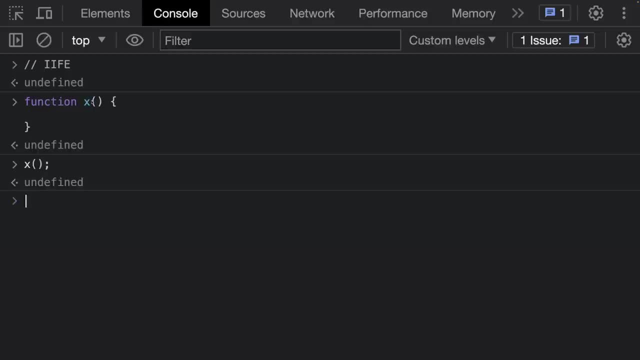 function at a later point of time, maybe wherever i have defined this function after 200 lines after that, based on certain logic, i am: i'm executing, i'm calling, i'm invoking this function- all right, but iiafe says that iiafe is going to be executed. in this case, the use of iiafe is to execute the function. 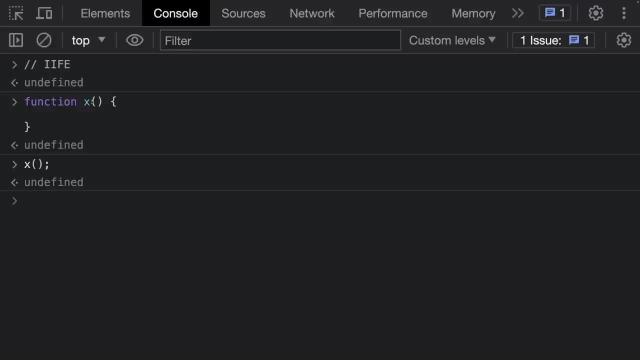 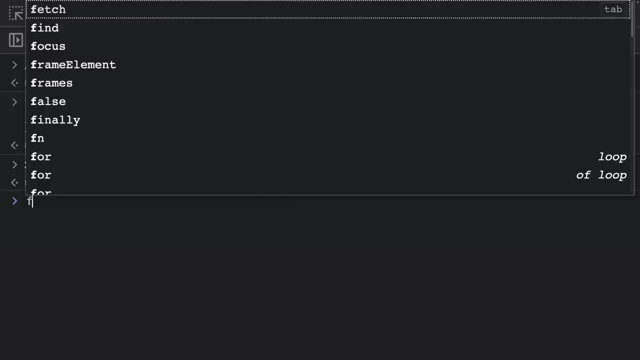 immediately after it's been defined. so if i have to do that, i don't need the name of the function, because the moment i define, right after defining the function, i want to execute it, so i don't need a name. so let's start with something which doesn't have a name. so i did function x before i don't give. 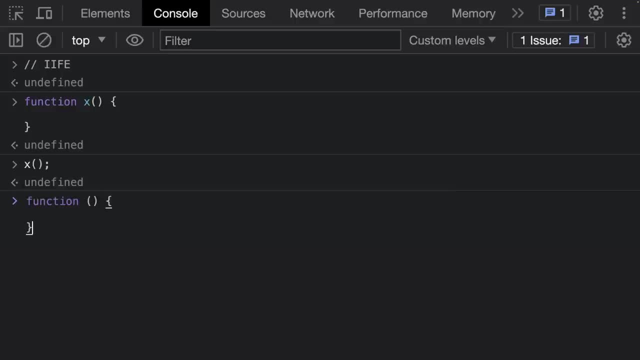 any x now, rather, i have created something like this, but if i try to run this, it's going to give me x, give me a problem, saying that function statement require a function name. okay, so now i cannot create an anonymous function like this and let's just keep it as it is because it's require a 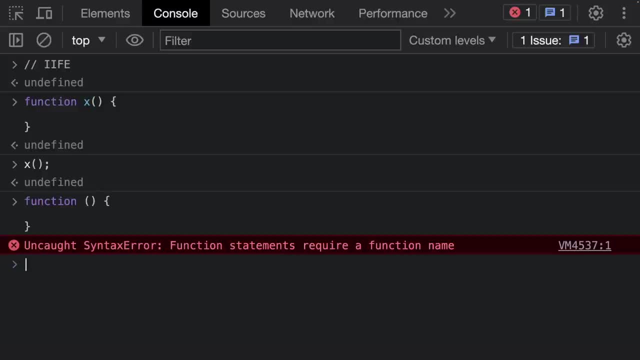 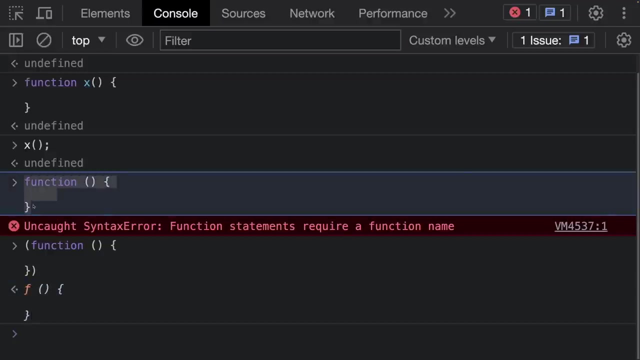 function name. okay, now let me introduce a operator called group operator, which is nothing but a bunch of parenthesis. now, if i put this anonymous function, the function without a name, inside this group, you know operator, what happened? if i just given enter, it actually gives me the string representation of this particular function itself, the string. 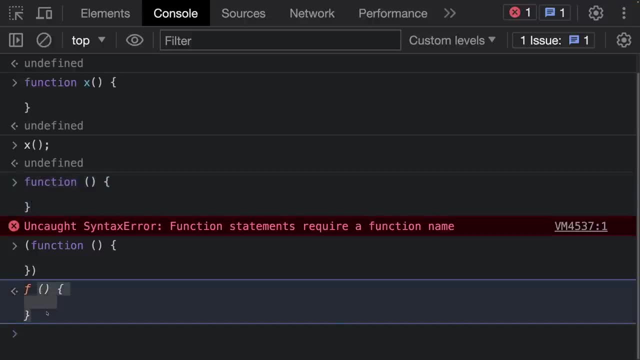 representation of this function itself correct, without any name bursting representation in previous chapters we have seen. whenever we get a string representation of this function itself, it means it's a function. so it means i can actually give the parenthesis after that to execute it. so it means if i take this guy and just put a parenthesis around this, it means it will be. 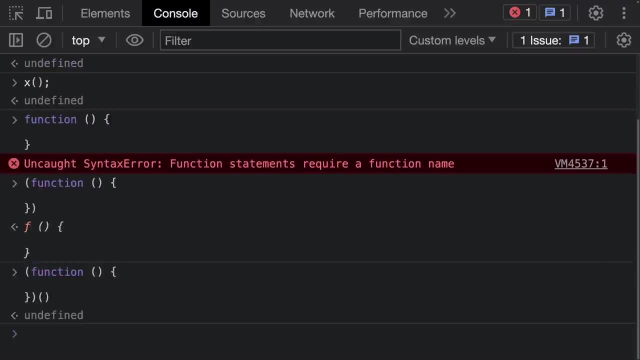 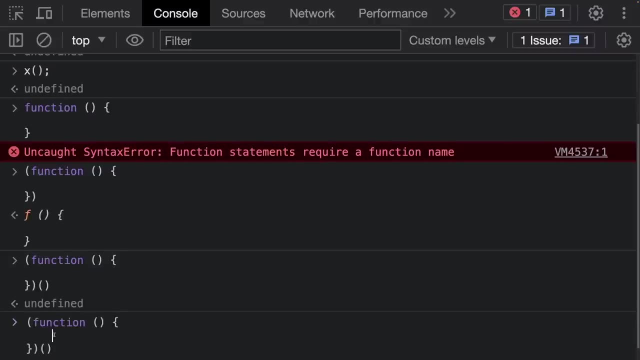 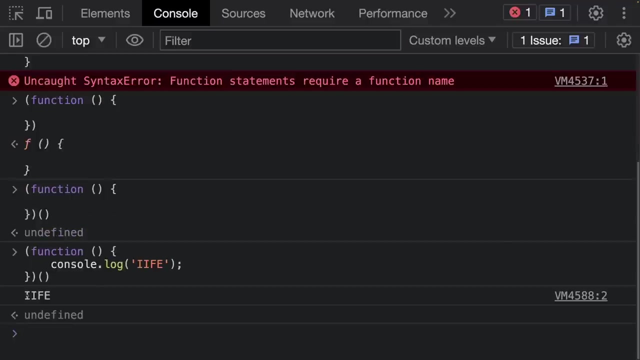 executed. yeah, So I have got a proper function. that's got executed. So this is what is IIFE. So now let me write a few code inside the so that you know that it gets executed. So console dot log IIFE. If I just try to execute this, you see that IIFE got printed. So the function when I am defining at the same time. 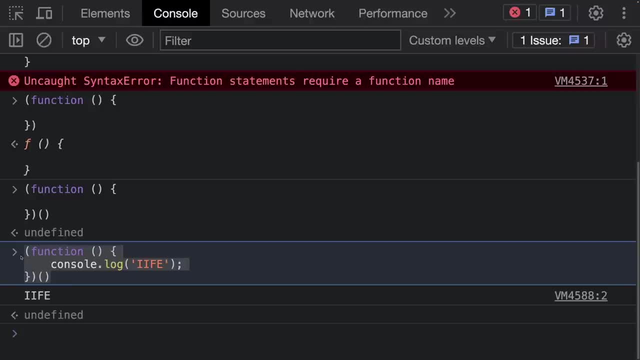 I am also executing this function. That is what is IIFE, That is what is immediately invoked function expressions. Now, if you ask, why does it exist? There are a few reason why it exists Before ES6 and before we had, like late const, all this better way of managing. 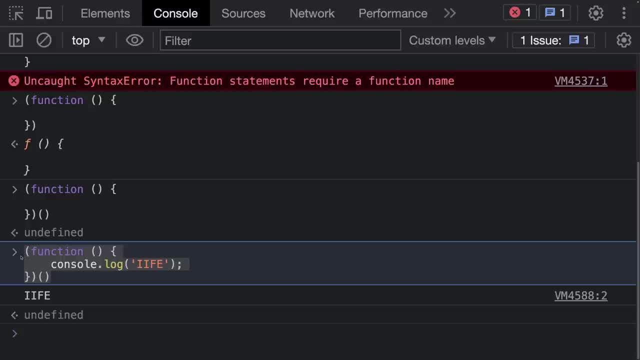 accessibility of a variable, like where it where what can be accessed, where where things cannot get polluted, where you have, you know, before ES6, where you had only var like the chance of your global variable gets polluted, you had no other option that using IIFE to protect them. 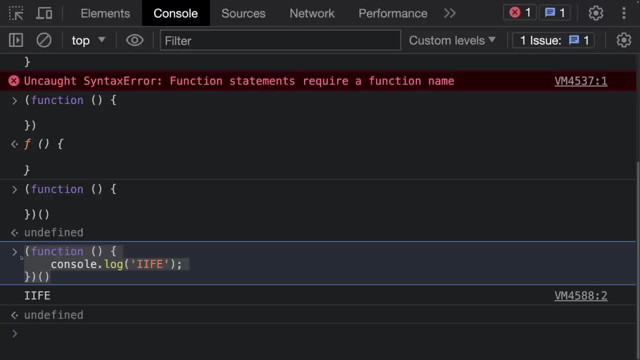 Okay. also, another reason is like. a very normal reason is like when you create a function with a function name, it means the function name. unless it is a like nested function or inner function, the function name basically exist in the global context right and the globally. it is not inside any other function. 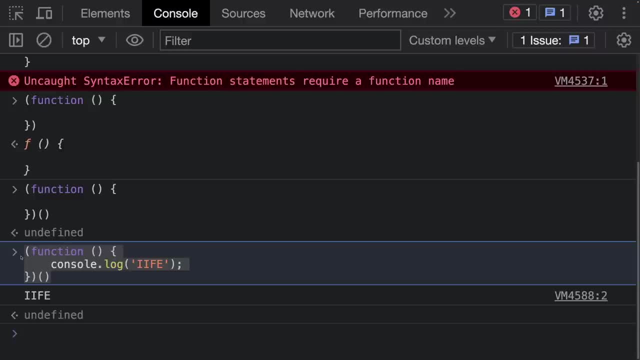 So it means there are chances that somebody else might be using the similar function name somewhere else might. there is a chance of kind of or a variable name with the same name as the function name and the chance of getting it polluted. So for that not to happen, the IIFE can be used. 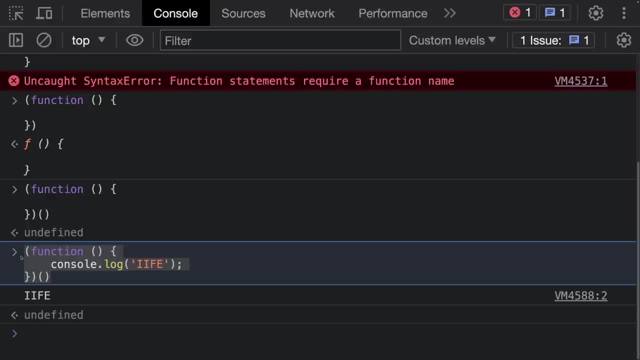 So IIFE can be used for various different use cases, but the concept of IIFE is this: that whenever you actually define the function, immediately after that you want to execute it. Only in this case you use the syntax and use that IIFE. I hope the syntax breakdown also makes sense to you, because it doesn't need a name. 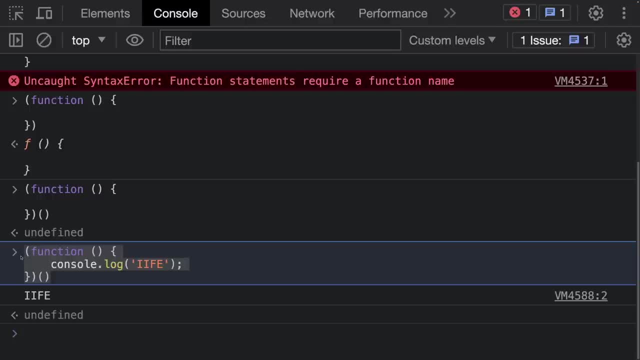 So we started with an anonymous function. Then we actually Used a group operator around that so that we get a function definition and then the last parenthesis- basically a pair of parenthesis- used always to call or invoke the function. We use it along with it and we got an IIFE result then. and there 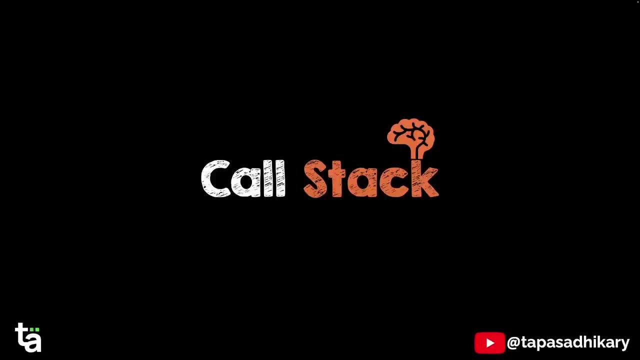 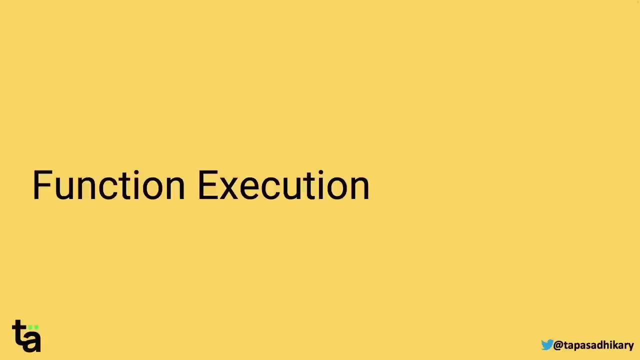 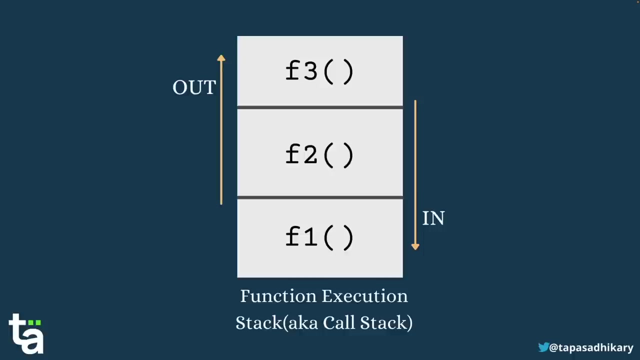 I hope it was useful. Thanks for watching. So you are going to understand call stack, but before understanding call stack we have to understand function executions very well. Okay, So first we'll understand what call stack is and also we'll understand what is function execution, so that you get a complete, clear picture about it. the element that gets inside the stack first, it comes out last, right. so here consider, there are three elements like F1, F2, F3. they went in like first F1, then F2, then F3, but when it had to come out, the F3 come out first, then F2 and then F1. that's how the stack stack works. 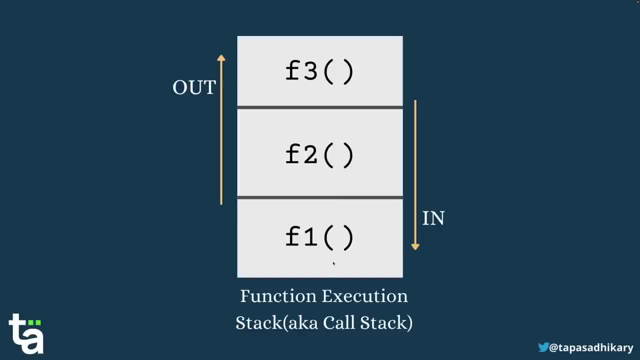 Now, instead of A normal variable, if a function gets inside the stack, then it will be like similar way: like first F1, F2, F3 gets in and then F3, F2, F1. it comes out in this sequence. so when a function gets executed, there is a stack that javascript engine maintains okay, and in that stack it defines like how the execution of this particular function takes place. whenever javascript interpreter go line by line and an encounter with a function, 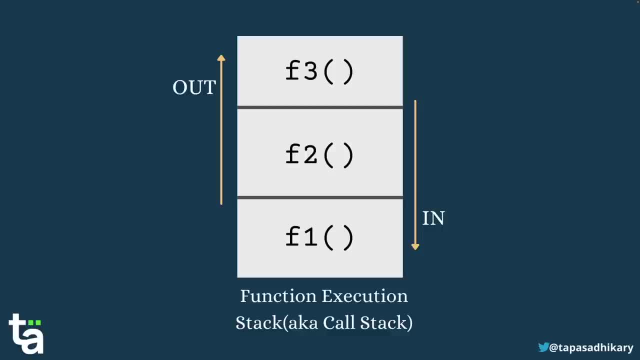 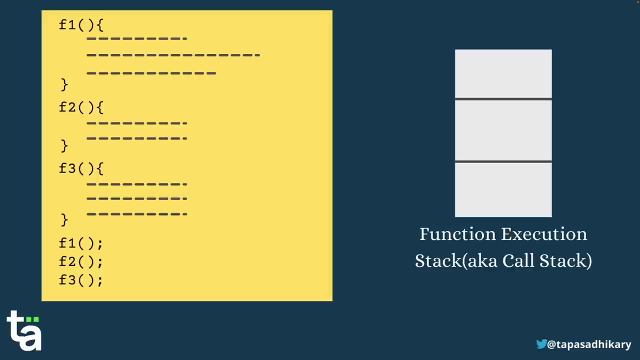 Okay. So when an encounter, a function call or a function invocation, it puts that function inside a stack, execute it and once the execution is over, it takes it out from the stack. the reason for doing this- there is a proper sequence of how the functions are getting executed- can be maintained through the stack data structure. we are going to see that with example. all right, so the first example that we are going to take. there are three functions: F1, F2, F3. you are able to see on the screen. each of these functions have been executed. 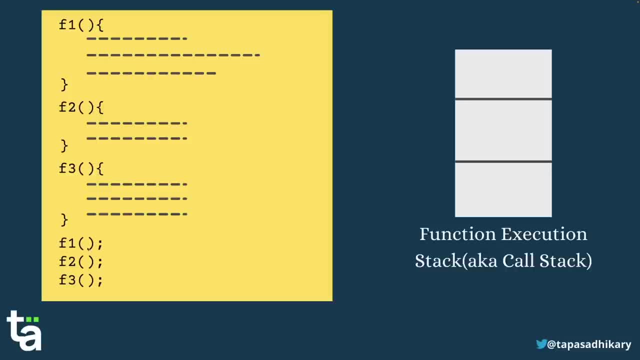 Okay. So we have a bunch of code that can be executed whenever we are invoking or calling this function. we are calling this functions first F1 first, then F2, then F3. right side we have a function execution stack or call stack. so call stack and function execution stack are the same. what we are going to see like when these functions are getting executed, like: first F1 gets called, what happened to call stack, then F2. what happened to call stack, then F3? what happens to call stack? that's what we want to learn. 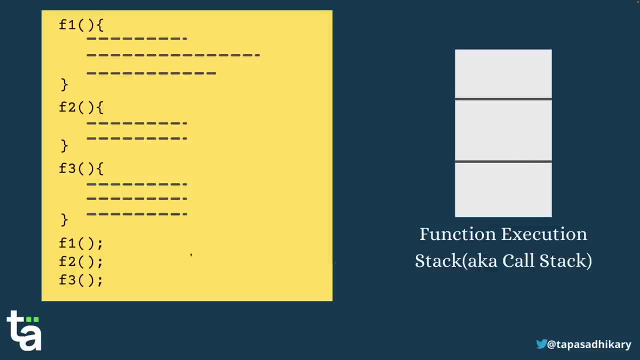 Okay. So please pay an attention To this call stack and also the how the code is getting executed. the first thing: first, F1, F1 gets executed. F1 gets inside the call stack or the function execution stack inside F1- bunch of code. okay, all done, done, done getting executed. there is no function inside it, so nothing else to put at this point of time inside the stack. then F1- execution is over. take out F1 from it. next, F2 gets executed. put F2 similarly over there. there is no function inside it, but execute it. 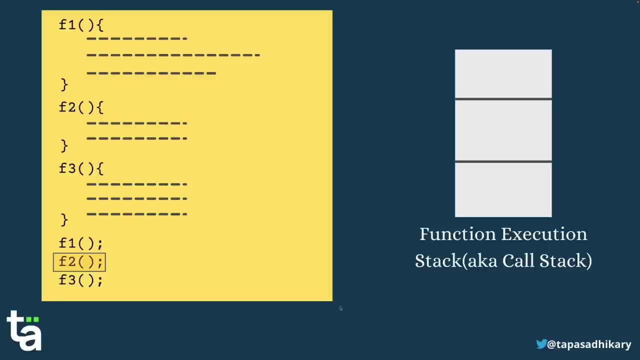 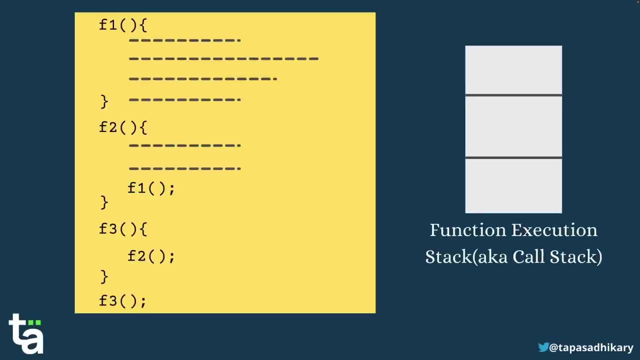 But execute all the code. execute F2, take it out. then goes to F3 again. put F3 inside the stack. execution is done. there is no function bunch of code. get it executed, it's out. It's very simple: F1, F2, F3 is got executed. now let's take a little bit complex scenario with this code. 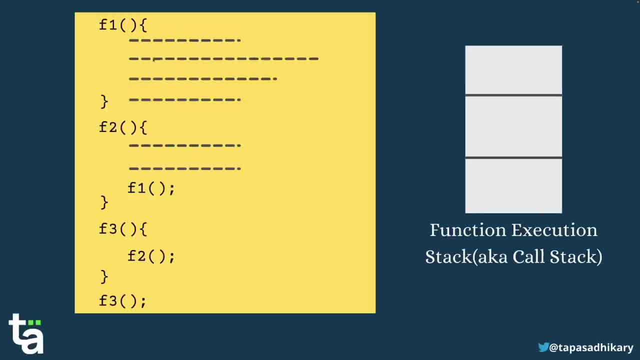 So what is happening here? you have F1. you have bunch of code. there is no function in it. then you have F2. you have bunch of code, but there is a function- F1- which you have defined before we are Invoking over here. you remember, a function can have another function inside it. a function can invoke another function inside it. yes, 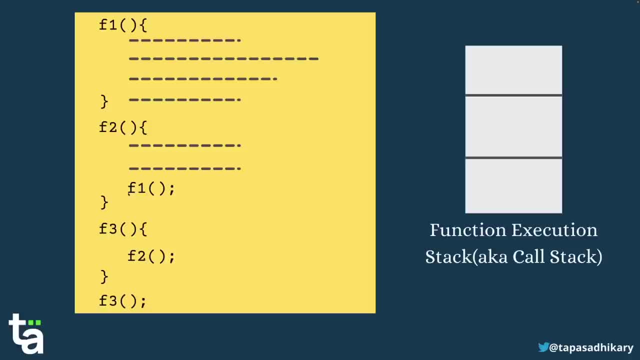 This is an example. so F2 basically invoke F1 or call F1 inside it along with the bunch of code F3. there is no other code other than it is executing F2. this like a chain right. so any invoke a free. it is actually invoking F2. F2 executing a bunch of code and invoking a. 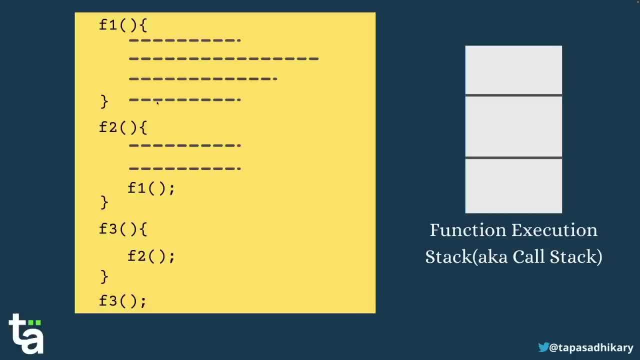 F1, F1, executing a bunch of code but no function getting executed. function invocation inside f1. now how this can be depicted into call stack or the function execution stack. that's what you're going to see, so again, pay attention to the right side. first, what happened? 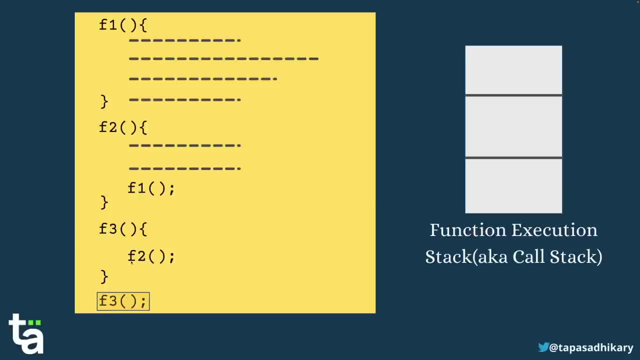 when f3 executes. when f3 executes, it finds f2. but before that f3 has to go inside the call stack, because a function has to go inside call stack to get executed. so now f3 get executed, it finds f2. oh yeah, f2, another function. so before i take out f3 out of it, because f3 will be taken out only- 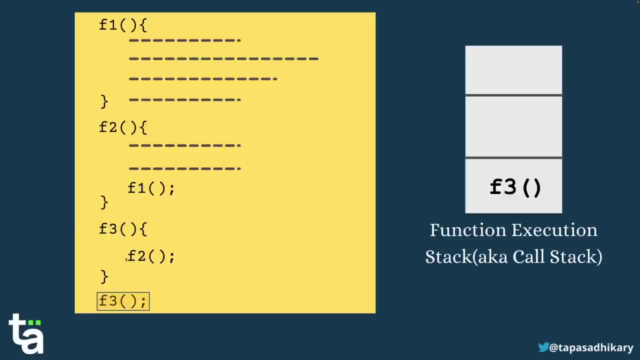 when f3's complete execution is over, but is not over now. the cursor is at f2, so it has to put f2 inside. f2 came inside, the f2's execution gets started, but f3 is still in the call stack. so f2's execution, a bunch of code gets executed. this line get executed. this line get executed. oh, now. 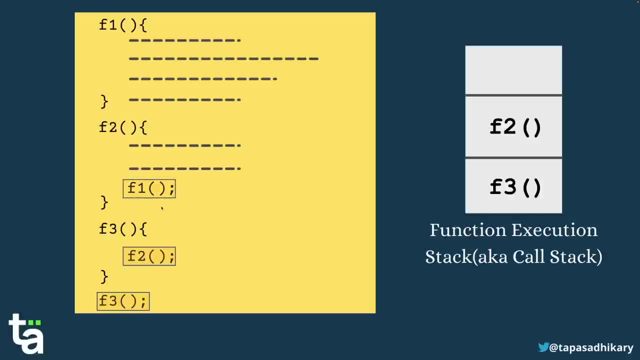 it encountered f1, which is also a function, so it's time to put it in the call stack stack. the f1 got into the call stack. now if you see in the call stack or the function execution stack, you have f1, f2, f3, but in the reverse order of how they have got entered. right now we are at. 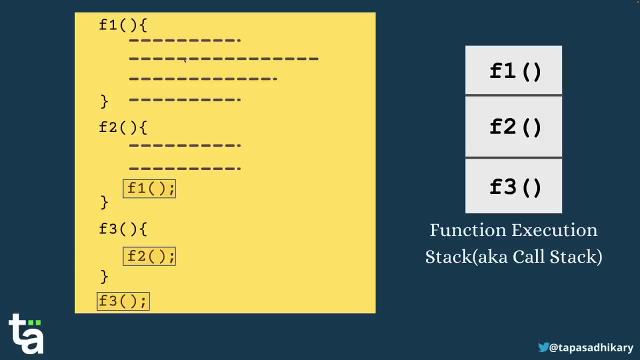 the f1, f1. a bunch of line of code are there. let's execute them one by one, but there is no function. so nothing else to put into the call stack, but execution. when it is over for f1, we have to take it out from the call stack. f1 is over now. our cursor is over here, so f1's execution is over. 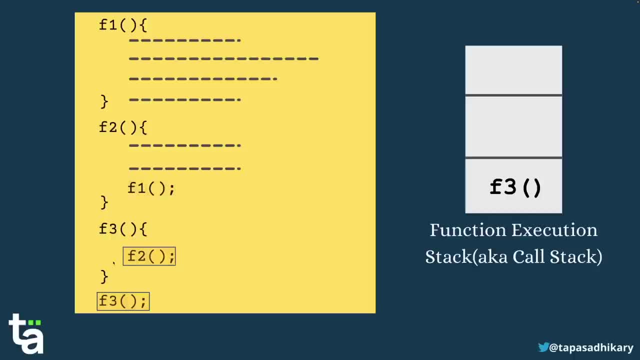 that means f2's execution is also now over. take out f2, so cursor is over here. f2's execution is over the next line. there is no more code. that means f3 time to take it out. isn't that awesome. so this is exactly what: function execution, stack or call stack. that's how it works. that's how. 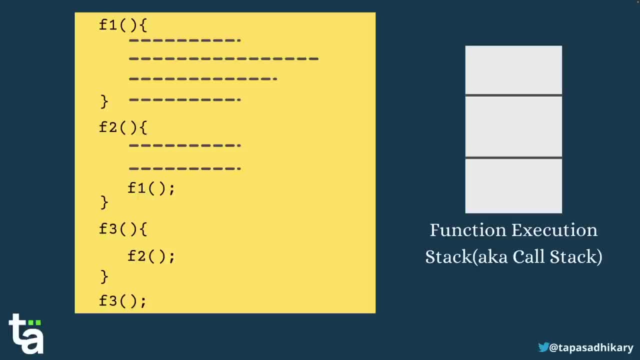 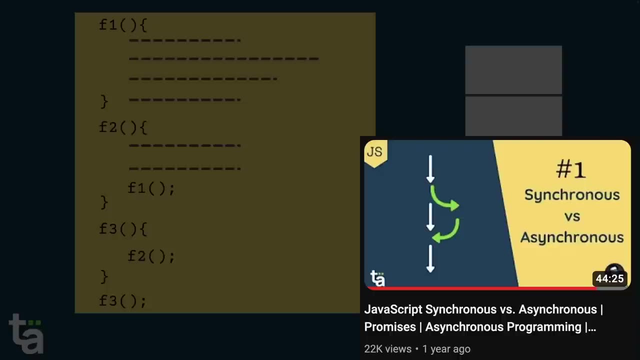 javascript engine maintains at what sequence your function should be executed. i hope it is very clear to you right now. now this particular concept is very, very important if you want to learn javascript asynchronous programming deeply. i have a complete series created for javascript asynchronous programming. if you are interested, go ahead and take that. 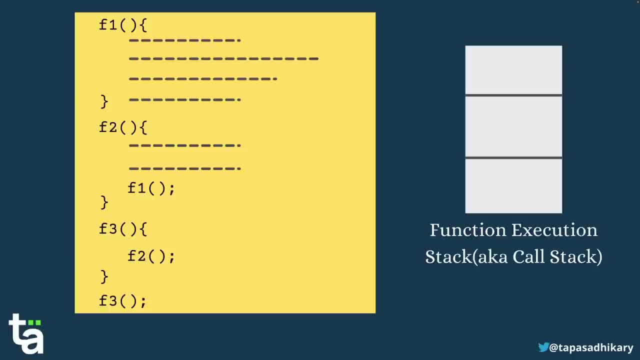 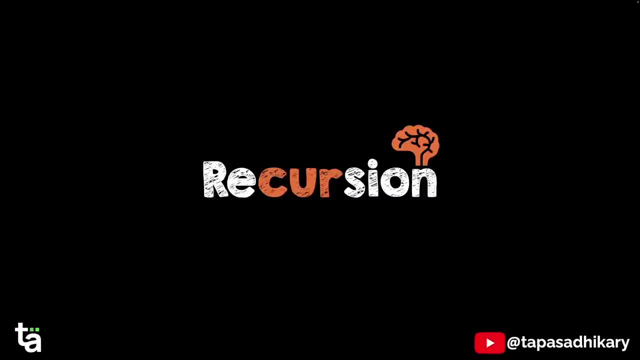 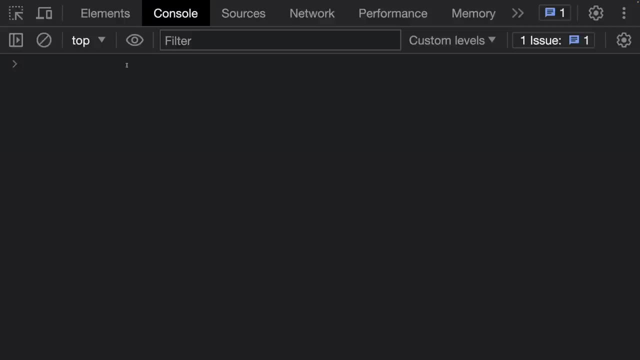 series. i'm sure that you will be able to master that concept very, very quickly. all right, thank you for watching. hello friends. let's talk about recursion. what is recursion? recursion means a function that refer or call itself okay. what does it mean? let's create a function, let's say function foo, and inside that we create, we do, we. 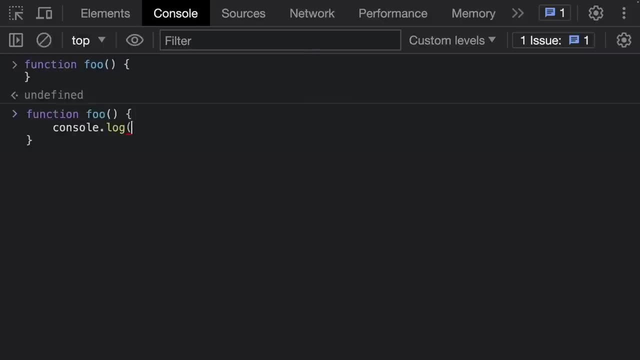 okay, function foo. inside that we do a console dot log, let's say foo- and then we say that a recursion is something where the function can refer or call itself. in this case, we'll call itself when, when we invoke this, so we invoke foo. okay, are you with me? what is going to happen? 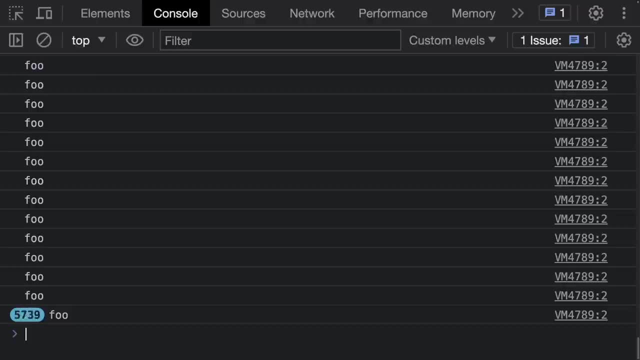 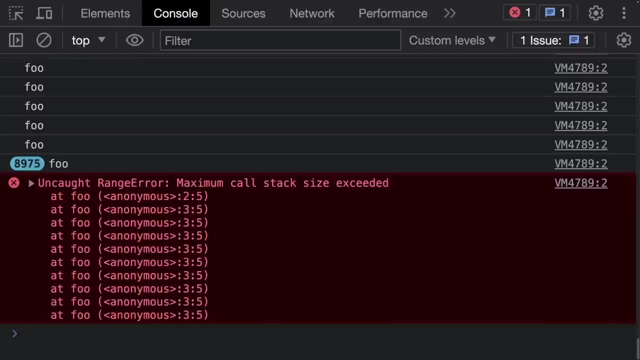 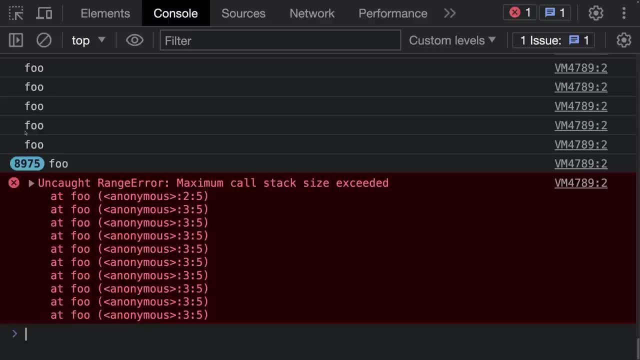 call stack, call stack, call stack multiple times and once will happen. the call stack has a max size defined when the max size limit- the threshold limit reached is going to give the error call maximum call stack, call stack exceeds. so that's the error that we are getting. okay, but if you're 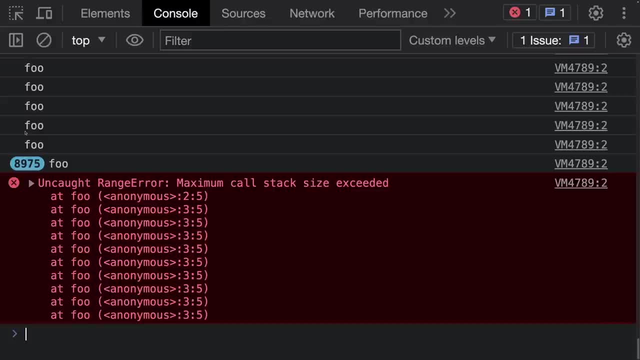 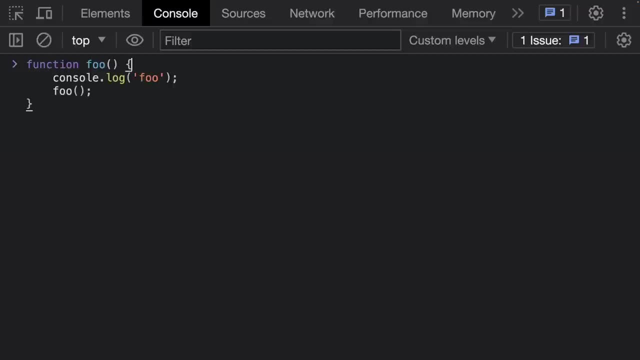 getting an error? what is the use of our recursion? okay, we'll come to that just a second, but before that, this is one way that we can actually define recursion like a function is actually invoking itself. let's do another way, that way how the recursion can be done. so, for example, const foo. 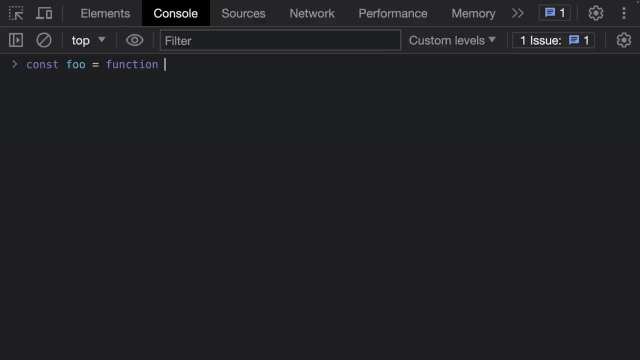 equals to function bus. and then inside this, what i'm going to do, i can call foo like this. what will happen? so in this case, i have created a function and the function is assigned to a variable called foo. so that means foo itself is a function. so in this case foo and bus are almost same. 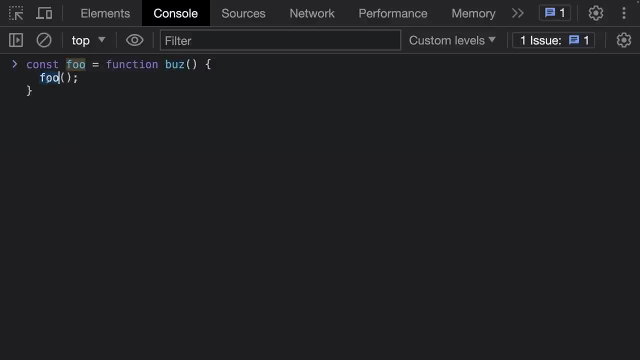 so whether you call foo here or you call bus here, whatever it is, you are actually creating a recursion here, because now you are referring to this particular function either with foo or with bus, whatever name it is, is the same function. so that's the another way you create the recursion. so in this case also, 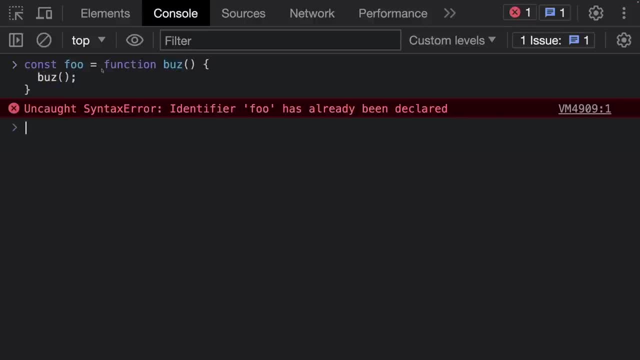 it will just. okay. foo is already exist because i've used this name before. so if you actually use it, it is going to actually create the recursion for you. okay, both the cases are same. now we saw, like, with recursion, what was happening. it was just creating uh, it was calling itself. 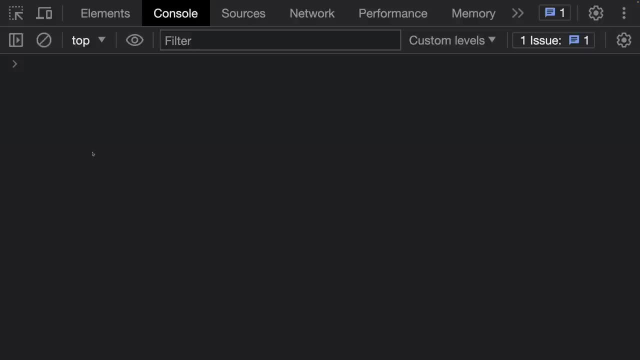 calling itself, calling itself, and then it hits the maximum heap size, and, and and the error out, then why should we use recursion? okay, so one thing is like: whenever you are using recursion, you have to make sure that you have something called best condition. okay, this is very important. 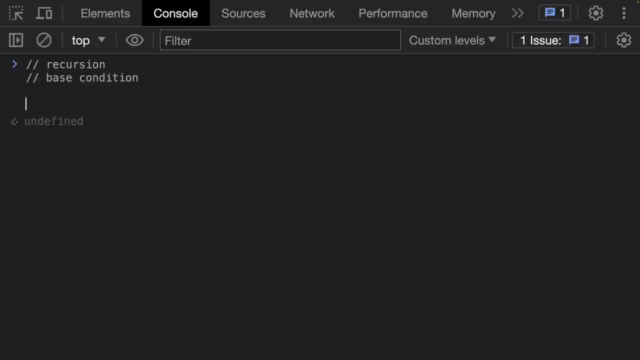 so recursion without a best condition is not of much use. best condition means under which condition you have to stop the recursion. so you have to stop the recursion at some point of time because you want to stop the execution of that function to execute itself at some point. 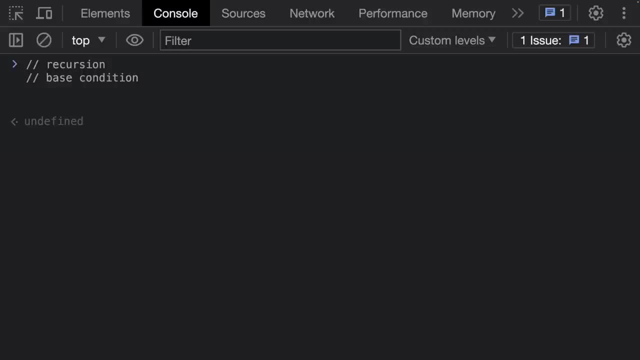 of time so that you can exit it out or do something else. so that condition is called best condition. okay, so usually how you will be writing things in recursion in a recursion program, so you will be writing something like function recurs, function recurs if it is a best condition. 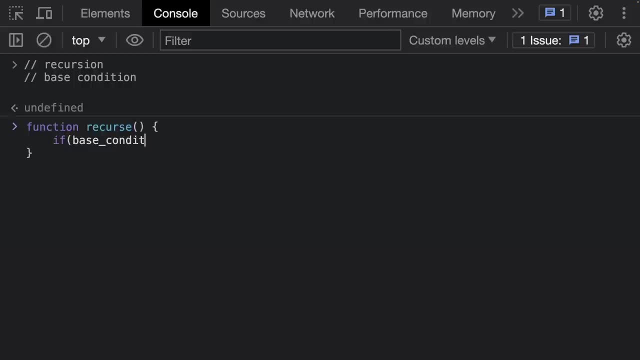 if best condition, in that case you probably do something and after that you return, otherwise continue to recurs. so this is how you actually do recursion: you should have a best condition and if there is a bit best condition, you do something and then return from it. otherwise you continue to recur. okay, let's write a program so that we can actually 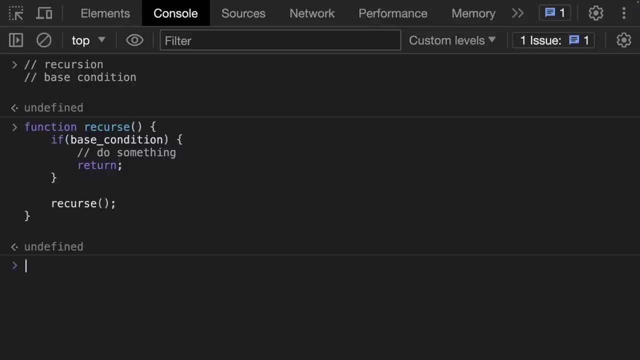 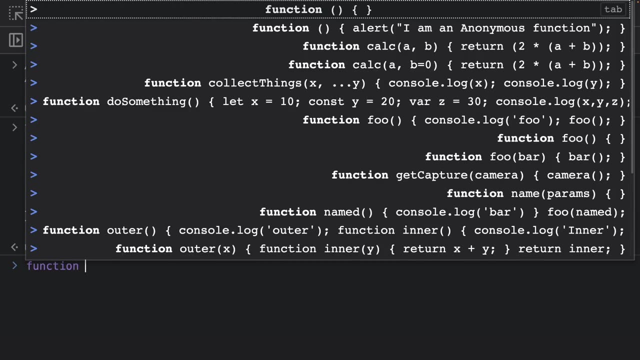 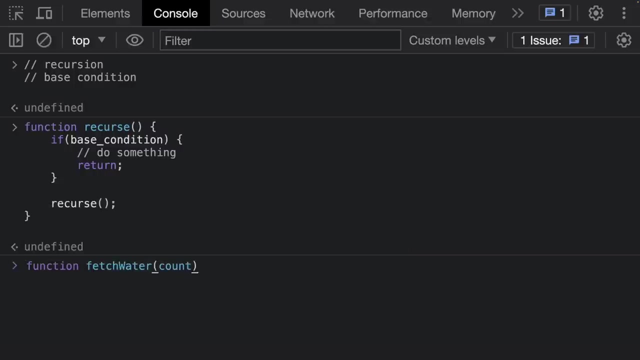 understand it in in much better way. okay, so the program that we'll be writing is about. let's say, we'll be fetching water multiple times, so let's call a function, create a function called fetch water, and let's take a parameter, call count, like how many times we want to fetch those. 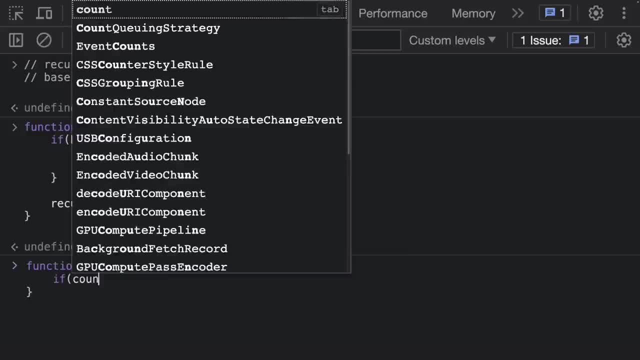 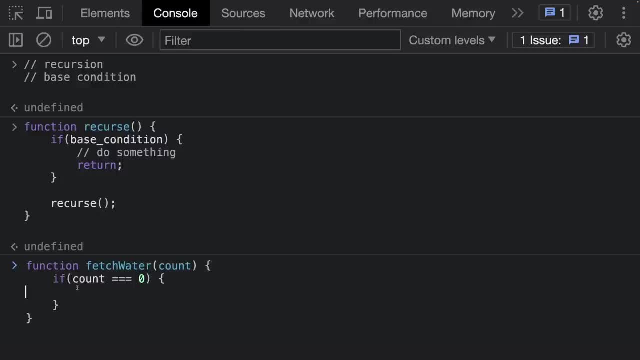 water and we say, if the count is zero, this is our best condition. okay, we have written the best condition. in that case, you do something. maybe I'll do like consolelog and say, like no more water left, so sad, okay, done, and then I will return. otherwise keep fetching the water and 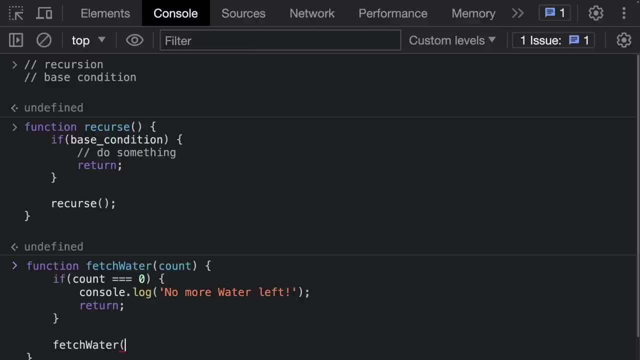 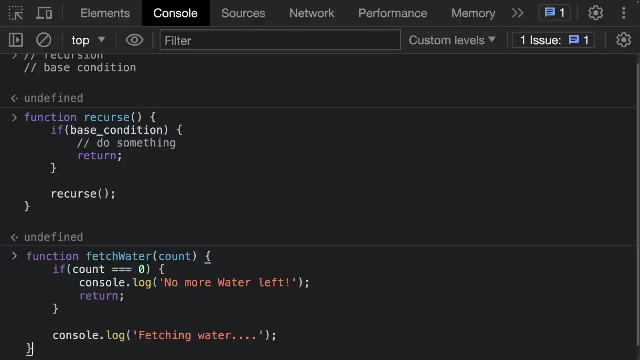 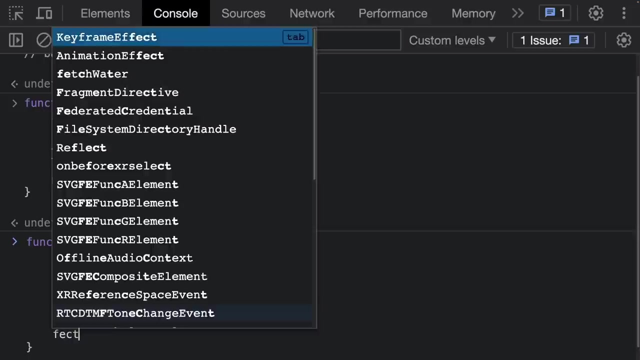 I will do like count minus one, and we can do a consolelog here also saying consolelog: fetching water. okay, we'll see the entire code and then after fetching water, we'll do that line got deleted somehow. fetch water, count minus one. all right, so let's read this code once more. 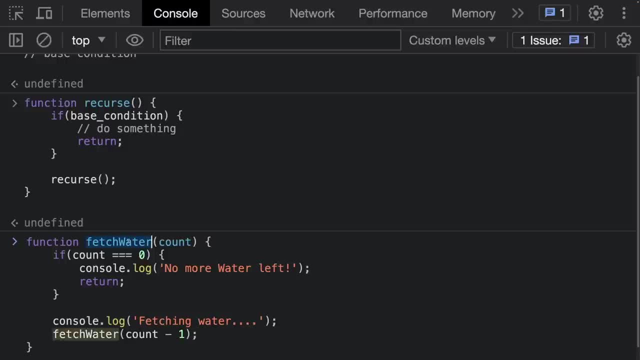 water, count minus one. and then I will do like count minus one and I will do like what we are doing. we have a fetch water. we are calling fetch water again here. so it's a recursion, of course, but we have a best condition, also the best condition. 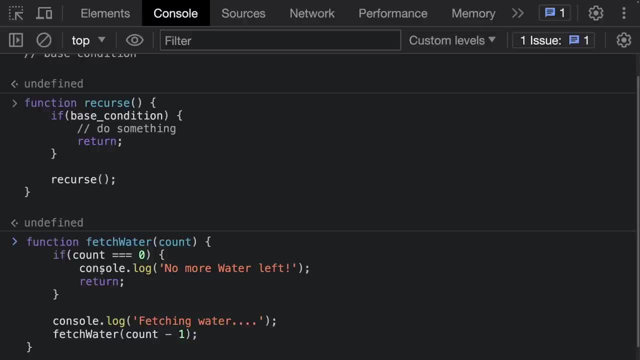 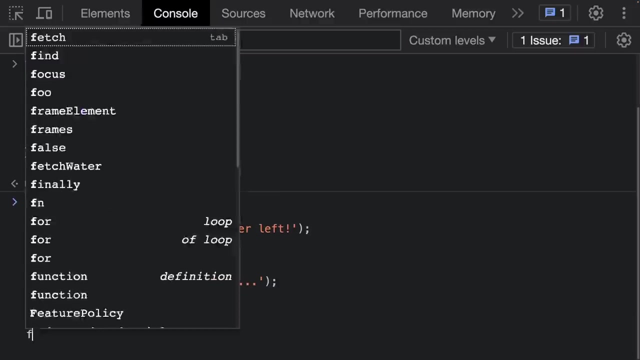 is when we'll be exiting from this recursion. our best condition says even the count is zero. then I am saying no more water left and break this recursion. but until count is zero I am just recursing it, just fetching the water correct. so now, if I say fetch water, 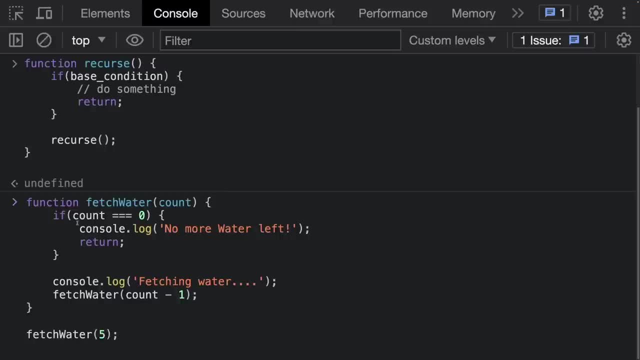 five times what will happen? it will go. count is five is equals to zero. no, it won't go inside. that best condition doesn't meet. fetch the water become count four, so count four means again call the same function with count four, so count four comes here. is four is equals to zero? no, again best condition. 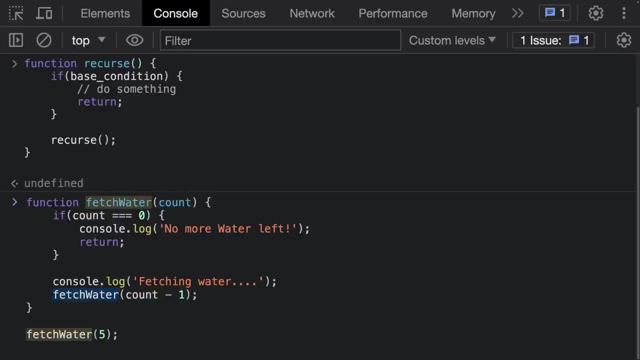 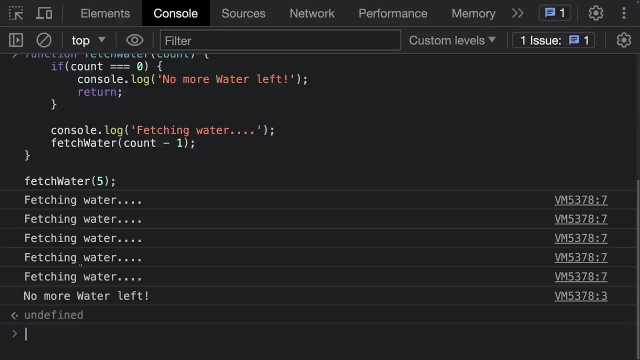 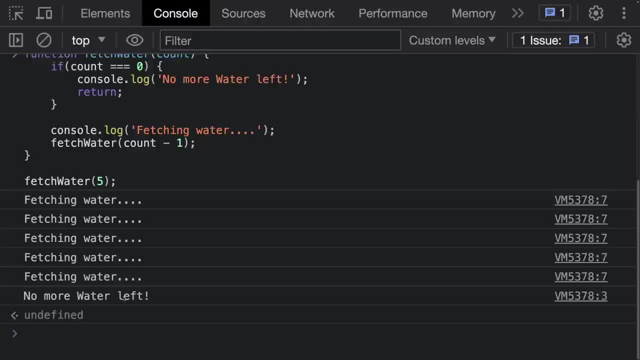 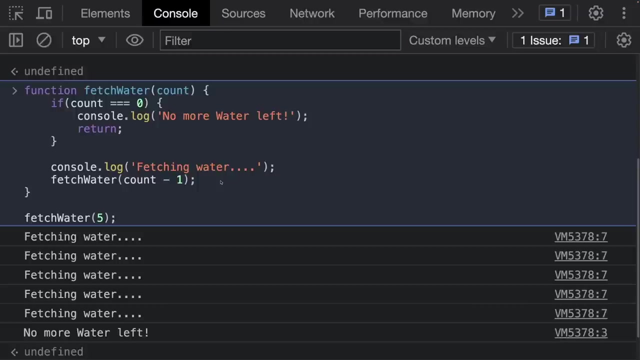 we have written a program using recursion and we also have the best condition through which we exit this recursion right now, the same thing you could have done with for loop, isn't it? the same function, same functionality would you could have done it with for loop. so there is always some debate like: 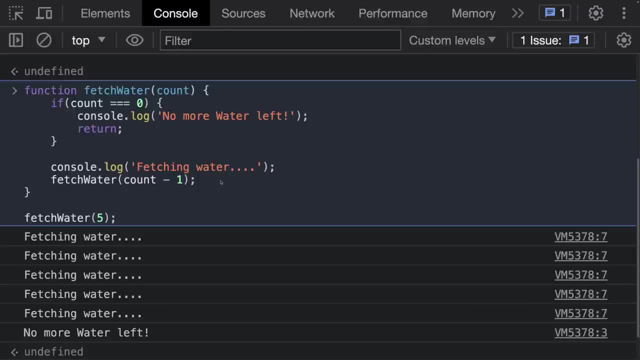 whether we should be using recursion versus we're using for loop. wherever the for loop applicable, maybe we should be using for loop, but in some cases, for example, you want to create the factorial of a number. factorial means factorial of n or factorial of 5 means 5 into 4, into 2, 3. 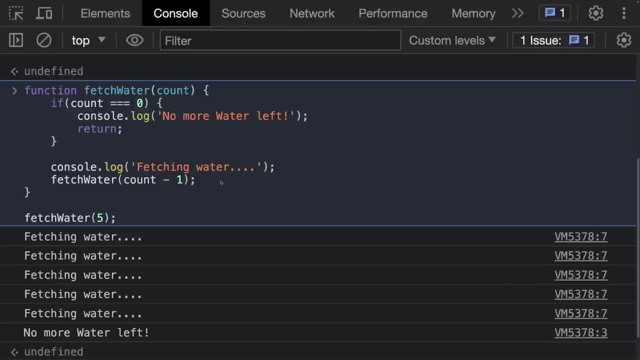 into 2 into 1, right. so the if you want to do a factorial, maybe the recursion is the right way to go, because it makes the code much more readable than doing a factorial using for loop, right. so readability is one of the factor that you want to probably take it into account when you 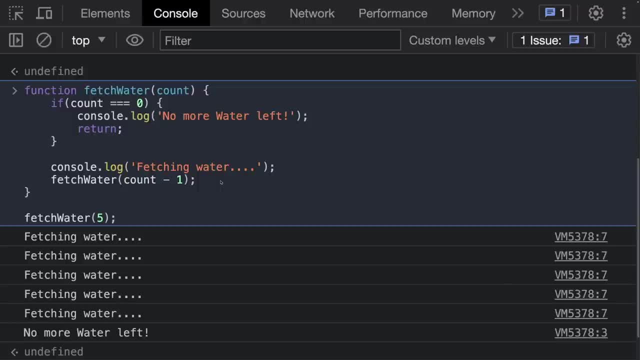 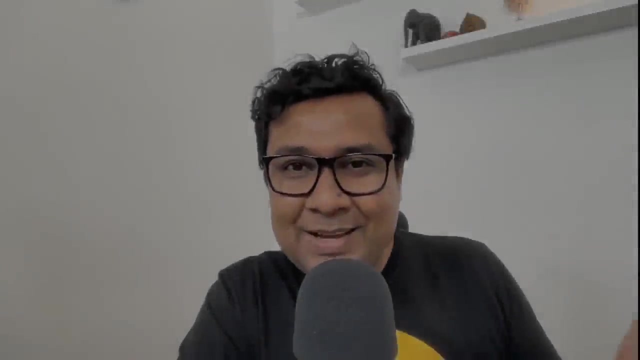 use recursion over for loop wherever recursion is applicable. so that's all about recursion. you, whenever somebody is asking about you about recursion, please also mention that you have a best condition where you can exit out from recursion. I hope it was useful. it's alright, friends, everything has to come. 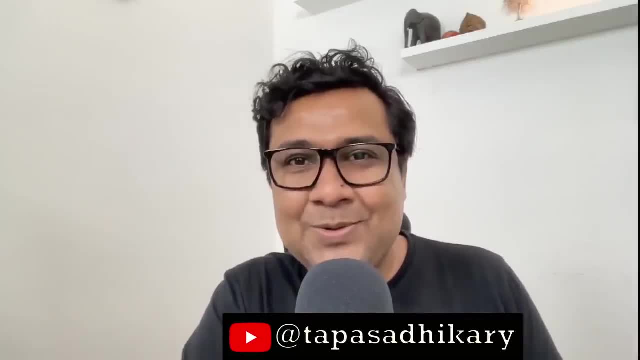 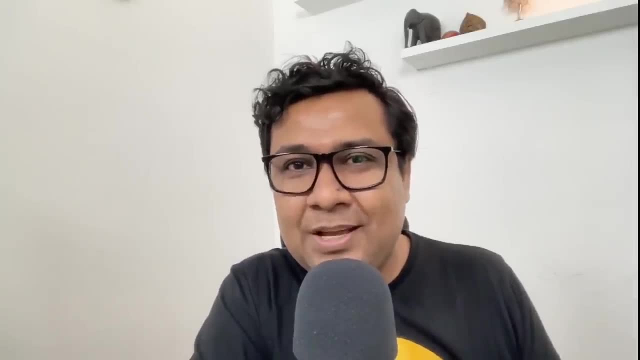 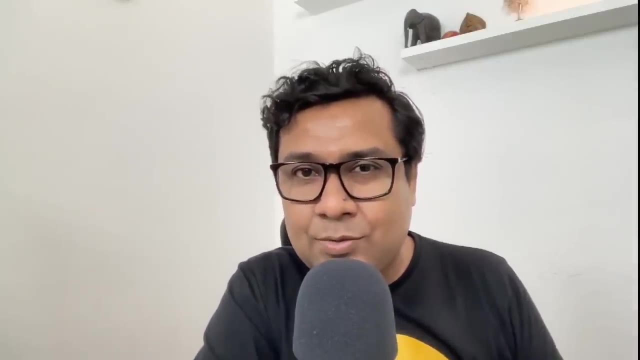 to an end, so our this crash course also has to come to an end. I hope you enjoyed learning all about the functions, all the things about functions, some of them after high level, some of them in depth. but the purpose of this course was to do a crash course where we can run through all the aspects of JavaScript functions. 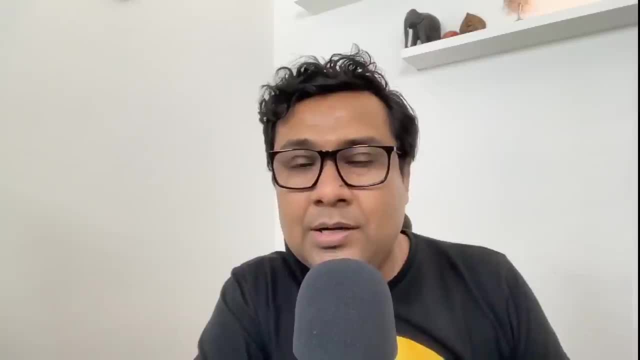 and give you an idea, give you the confidence that you can learn some of these concepts if you learn incrementally, if you learn by connecting the dots. so we started with very basic things like how to create a function and ended with recursion. in between, we touched nested function, function, scope. 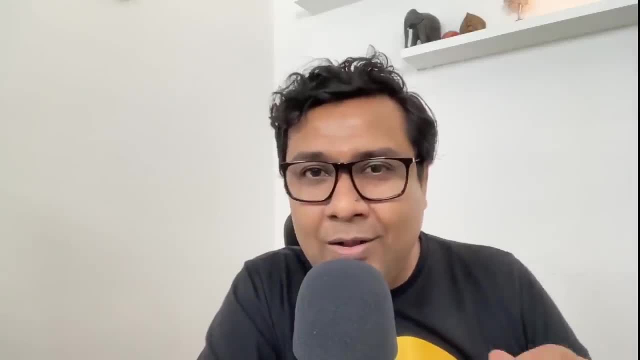 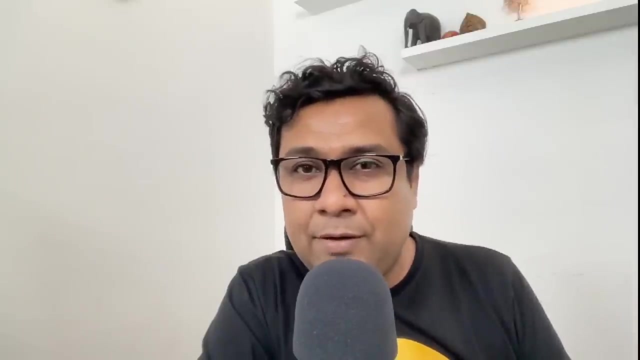 closure, pure function, callback. all this very various aspects. but your learning should not stop here. you need to keep practicing each of this concept much deep by with your hands-on, and I have videos for some of this concept to teach much more deeper way. for example, call back: pure function, HOF. you know a lot of these things are having in-depth real 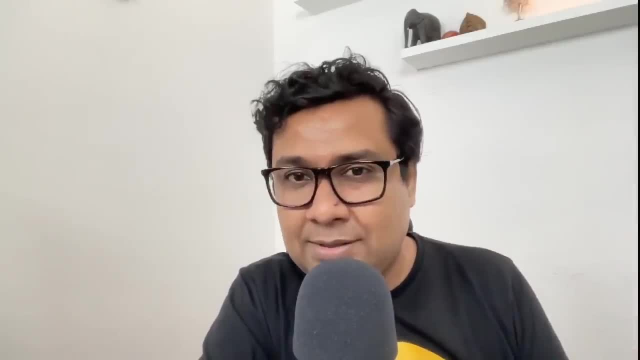 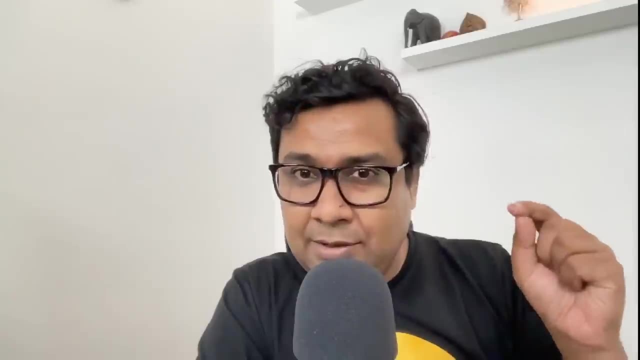 life use case scenario videos. please go and watch them if you're interested. or if you want to read it from somewhere or from some other YouTube channel, please feel free to do that. but the learning should not stop here. you need to keep. learning should not stop here. this crash course purpose was to give you a 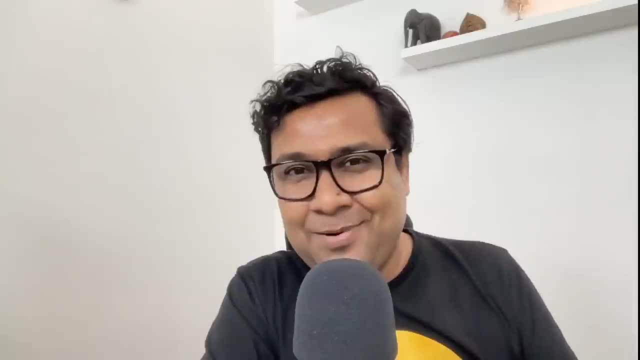 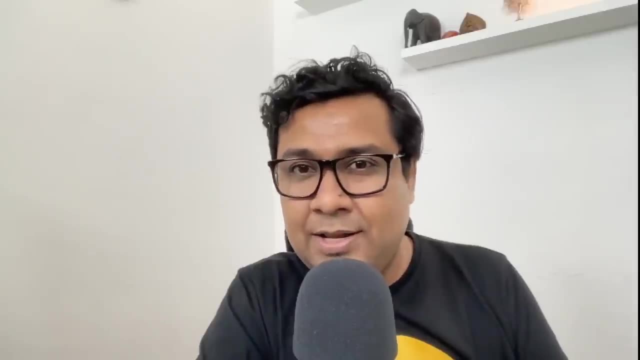 start. give you the required confidence so that you can now keep learning. all right, all the best. and again, a simple and small request: please subscribe to the channel, if you have not done already, and hit the bell button so that whenever I publish a new video, you get a notification off. all right, take care of. yourself. I'll be come back another video very soon, thank you.